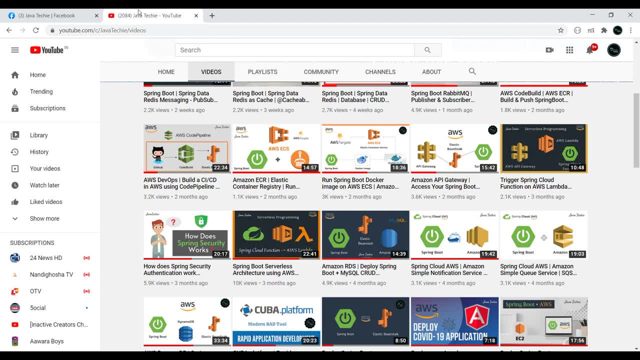 Hi everyone, welcome to Jabba Techie. This tutorial is remake of our earlier spring security video, as lot of people faced issue on existing code and they suggest me to remake this content. That's the reason I am repeating this again. Okay, Alright. In this tutorial we'll implement role based authorization by considering one real time scenario. So if you have been part of any Facebook group, then you must have some role assigned to you. For example, this is the group which I created, right? 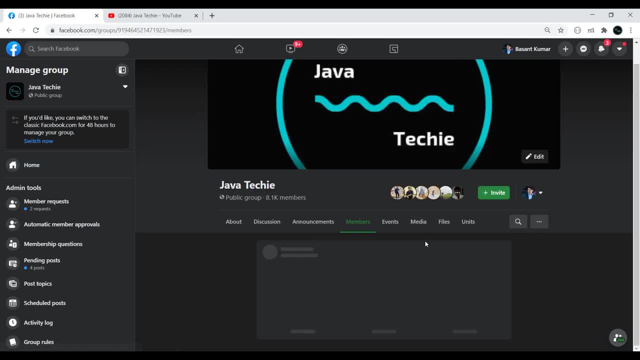 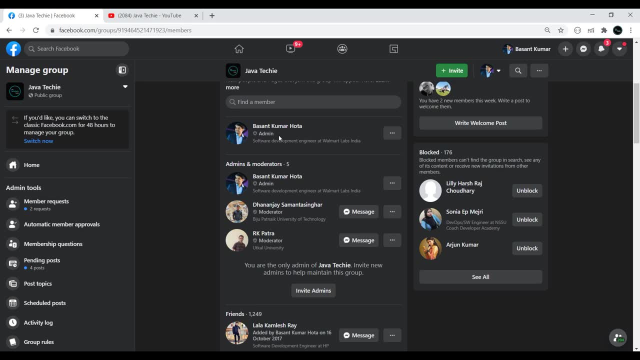 Now, if I'll go to this member section and if I'll go down, I can find couple of role here. right As I created this group, I have admin access and there is couple of member who have moderator access. So by default, if a new user joined to this group, so the role will be user and as a admin or as a moderator. if I want or moderator want, we can assign him as a moderator. But as a admin, either I can give admin access to the user or 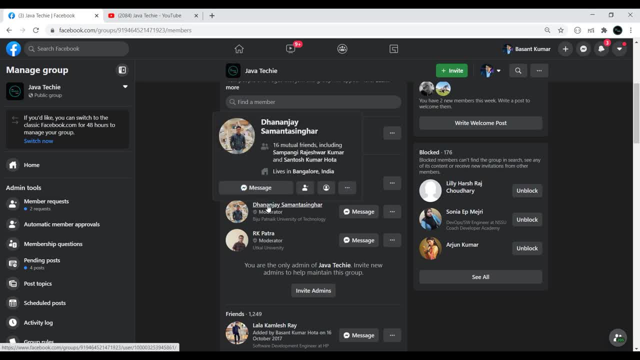 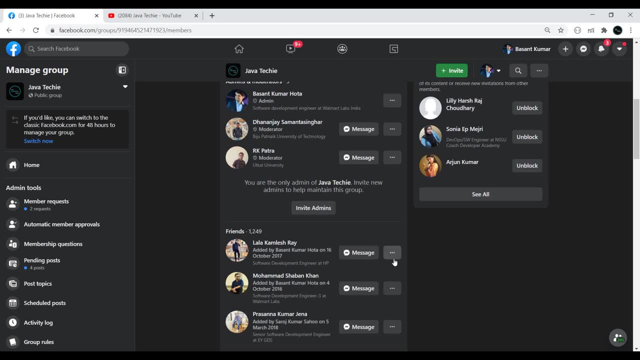 moderator access to the user. But let's assume this Dhananjay- he is a moderator, he can give only moderator access to the user. So, for example, as I have admin access, so if I'll click on this Muhammad Sawan Khan, and here I have option to make admin or make moderator, if I'll click on make moderator, he will be moderator and the invitation will send to this particular user. Similarly, if there is new post in group, a admin or moderator. 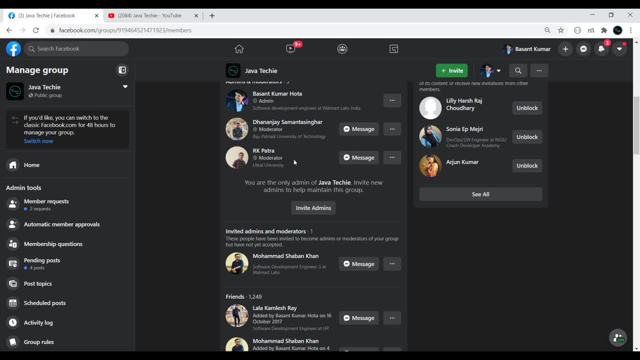 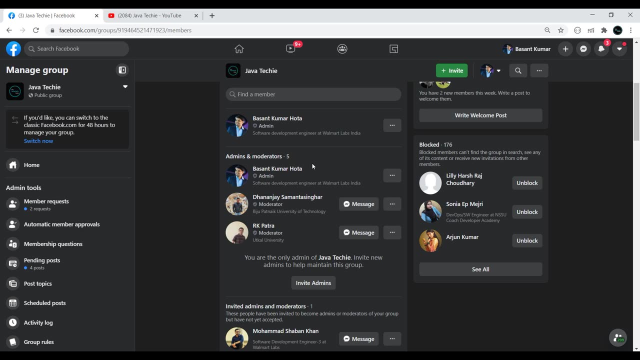 can only approve that. either they can approve or they can reject, either they can approve as a single post or they can approve as a bulk post. Okay, so this is what the feature given by Facebook. So we are going to implement same kind of features using this spring security concept. So in this part, one video, I will just cover this role based authorization. By default, the user who will join to this group have the role user And, as a admin, we can give someone to the moderator access. or, as a moderator, we can give someone to the moderator access. 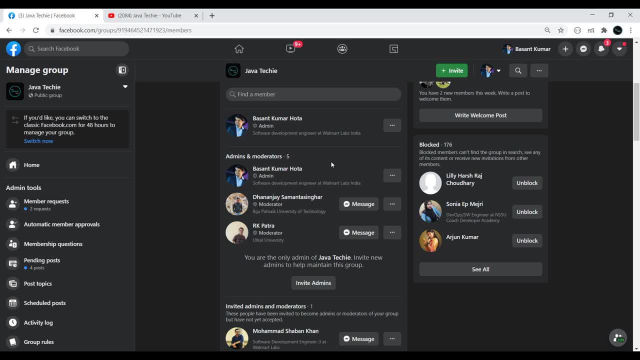 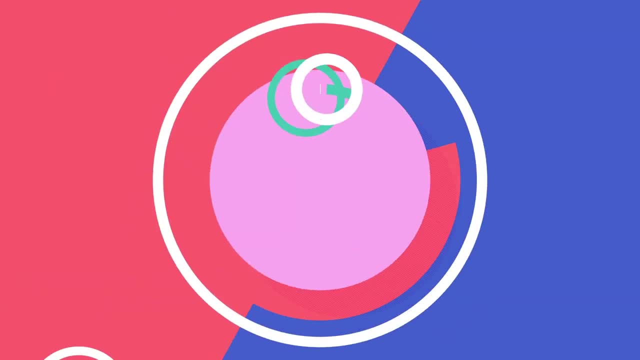 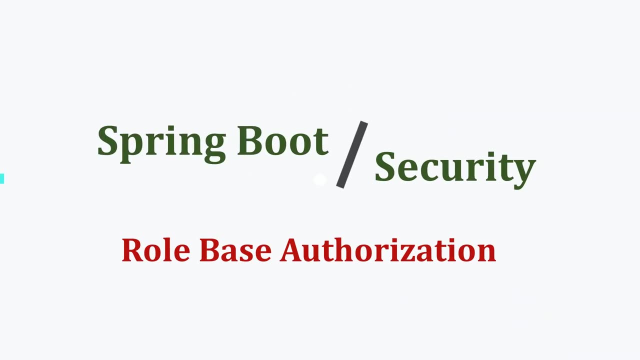 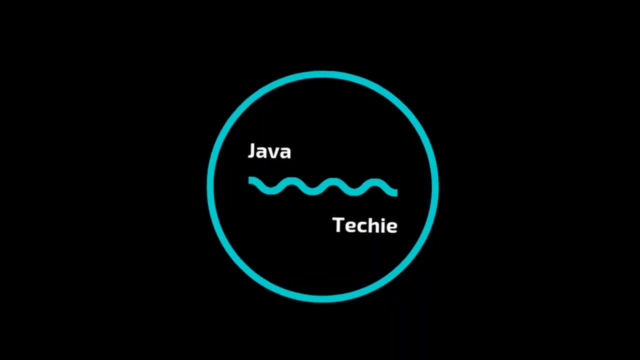 someone to the only moderator access. Okay, so this is the scenario we are going to cover as part of this tutorial. So let's begin with the development. Let's get started. So let's quickly create one spring boot project. click on file. 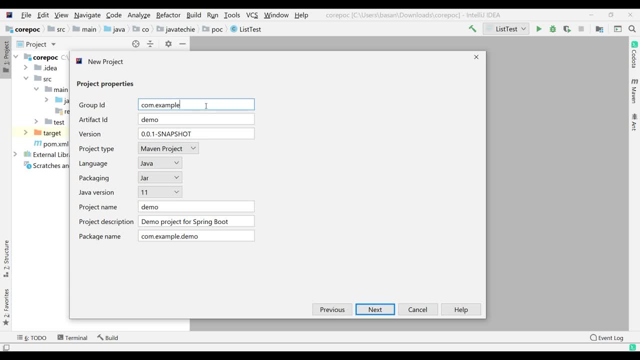 Click on project, click next, So specify the group ID: comjavateki. Then I will specify the project name as javateki group service or something like that, Then change the Java version to eight. Also I will specify the same as my project name, then change the package here: comjavatekigroup. Okay, now click next. So let's start the project. 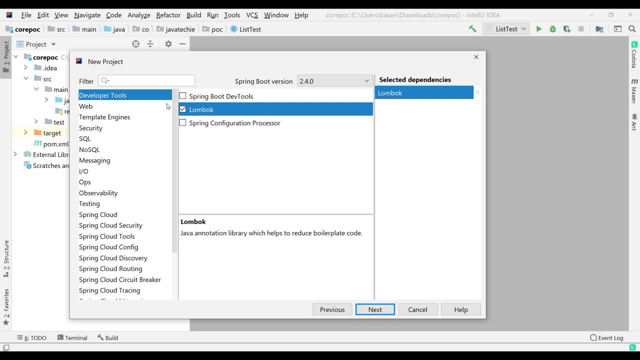 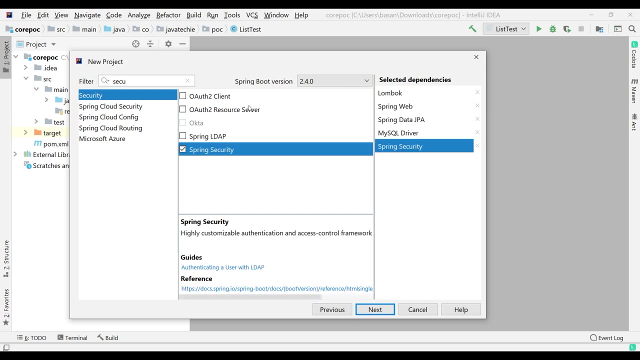 So now we have the required dependency- Lombok- Then we'll add spring web, Then we are going to integrate with database, So we'll add spring data, jpa. Also. we want my SQL And we want spring security. Fine, Also, if you observe the spring boot version, we are using 2.4.0.. So click on next. 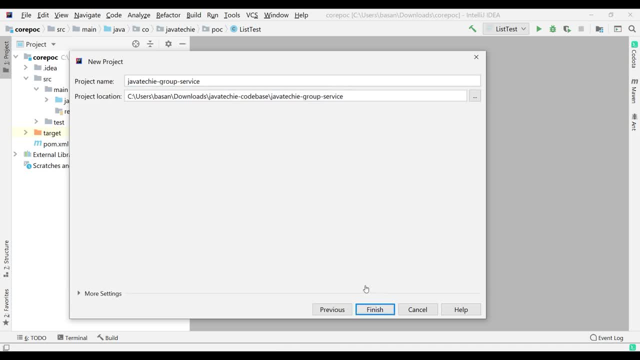 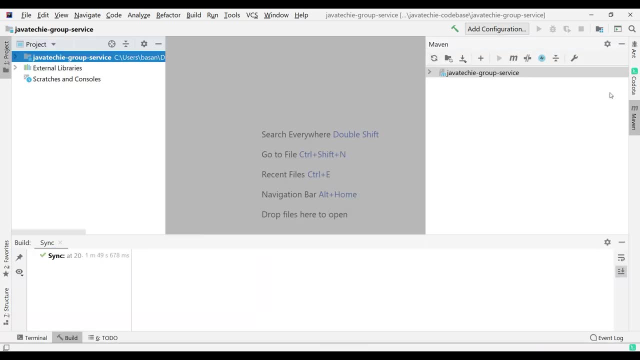 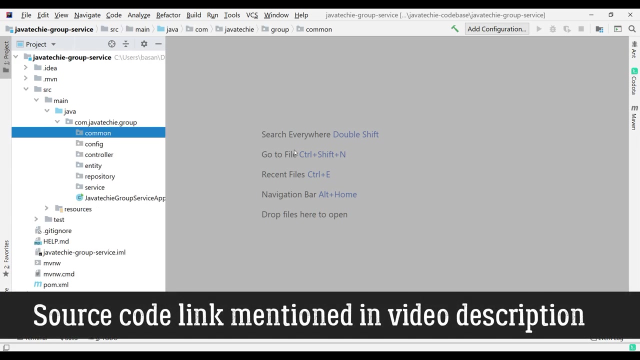 if anything else we need, we will add later. click next now. click on finish. let me minimize this. now, if you will go to the project, go to the src main, java, then the package. so let me create couple of package. so let me pause this video. so if you observe, i created couple of package. common config controller entity repository. 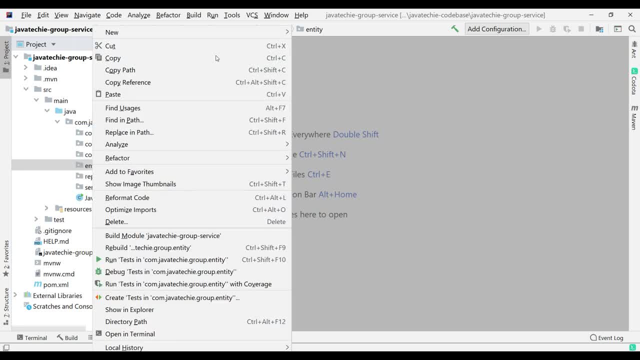 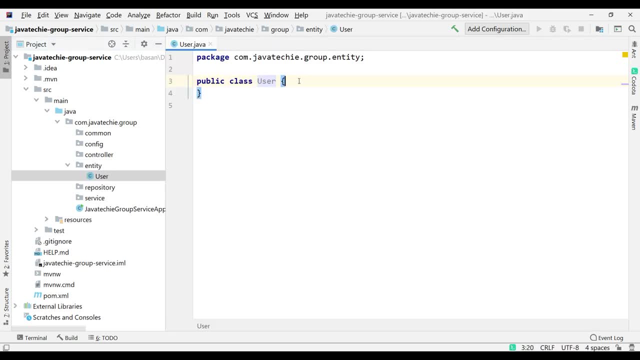 then service. ok, so let's begin with entity class. let me create a class, let's name it user. then let me add couple of field: id, usrname, password active under role. ok, so you can create separate multiple entity. you can create entity called user and you can create entity called. 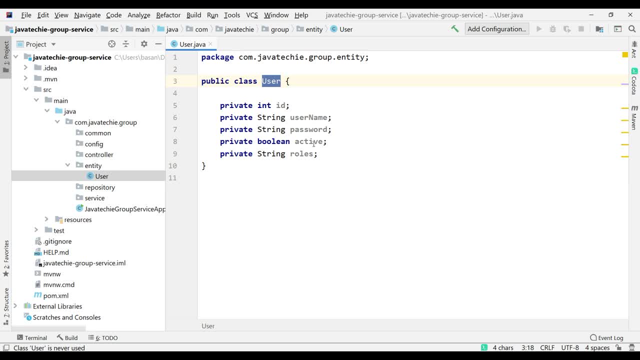 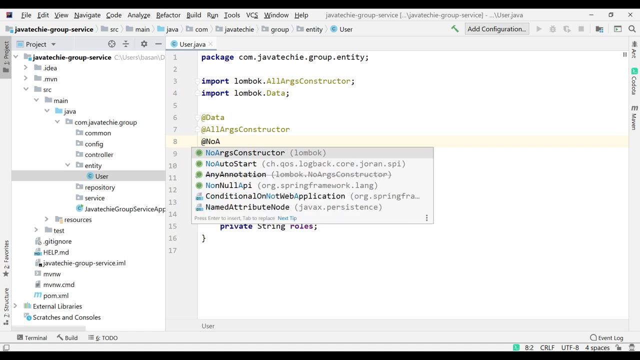 roles can make them a relationship one to many, but for this example i directly keep in a single user class. okay, as you added lumbok, we can directly annotate your at the rate data. we want all argument constructor. we want no argument constructor. also, we can give to string as. 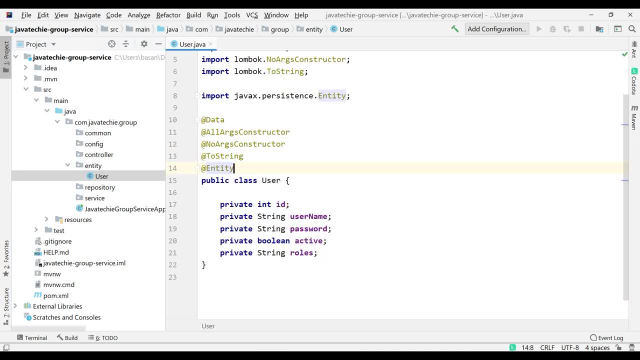 this is my entity. i need to annotate at the rate entity and i need to specify the table name. okay, i'll give user auth tbl, something like that. okay, and as this is the id which is my primary key, i need to annotate at the rate id and i want this id value should be auto generated, so i will use. 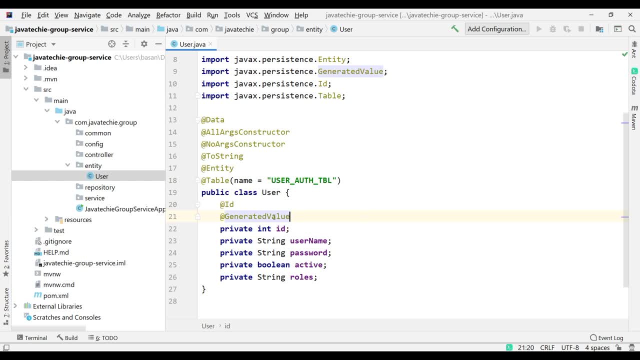 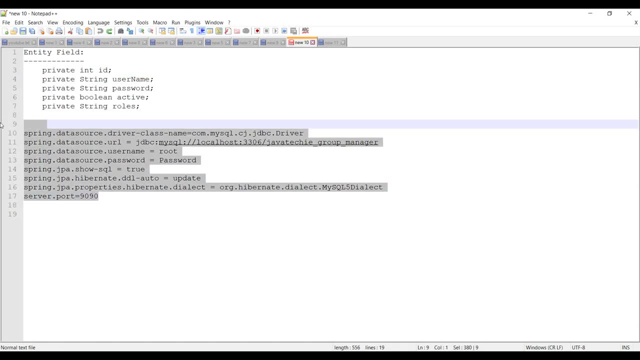 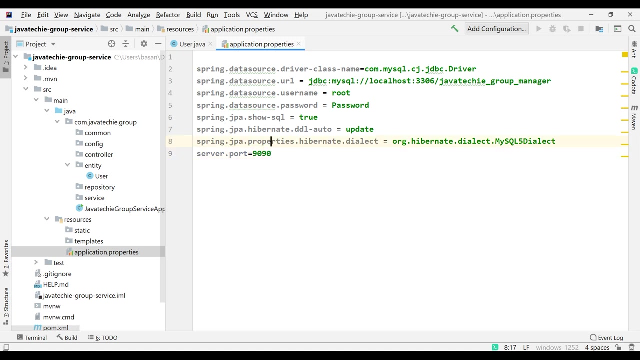 i want at generator generated value. fine, we created entity. now, as our application need to integrate with our mysql, we need to add our data source related properties in our application, right? so i have that. let me copy this. fine, so let's format it properly. so these things you need to change based on your configuration. okay, so this is what the database. 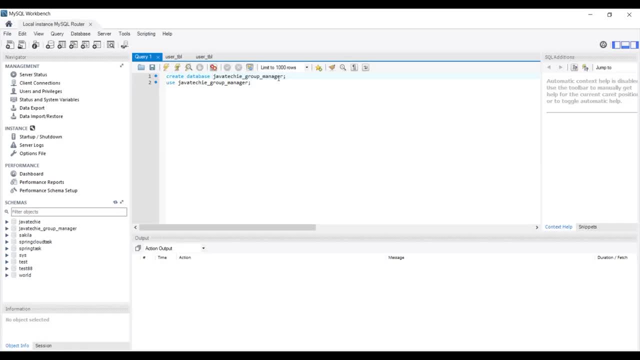 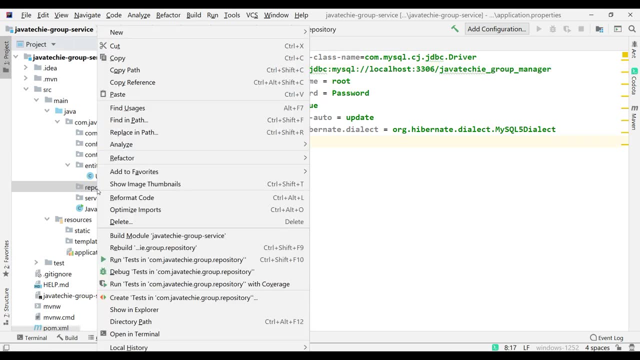 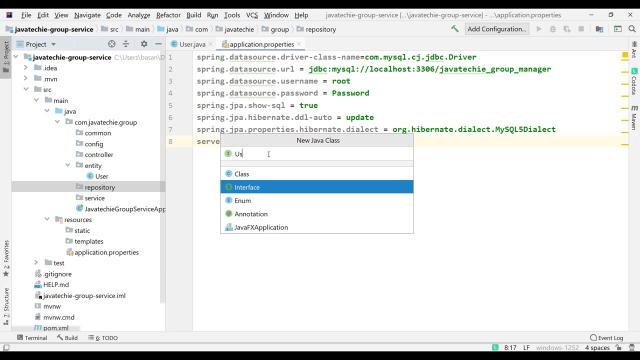 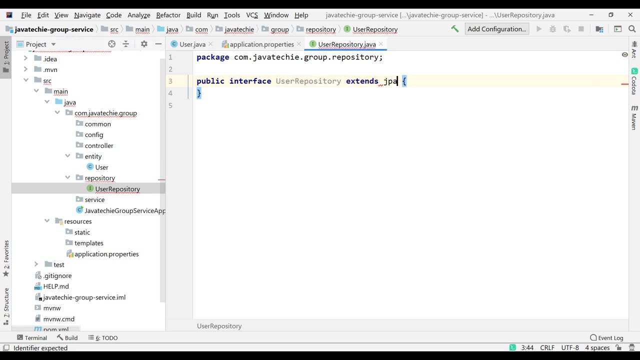 name which i created. so if you'll go to my mysql, this is what the database i created. right now let's write our jpa repository, okay. so just create a class now, make it interface, so i'll name it user repository. then extend it from jpa repository as you are using spring data, jpa. 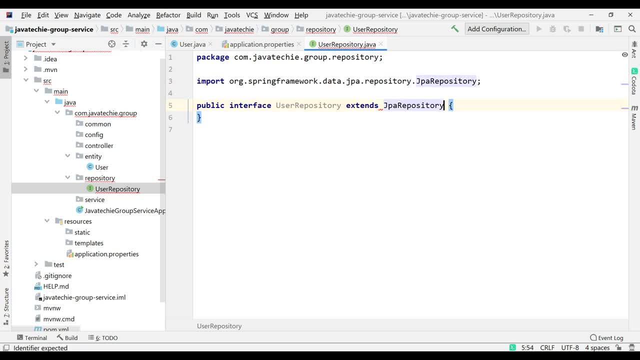 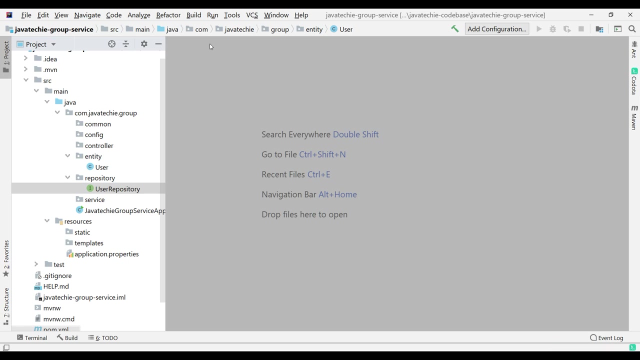 okay, so the first argument will be your entity. so the entity is user and then primary key of your entity, that is the integer, right? fine, we created our entity and we configure all the data source properties and we created our user repository. now let's write the config file where we can authenticate the user. so go to the config, create a class. 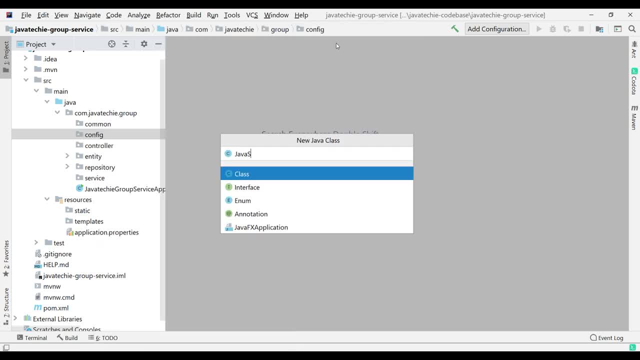 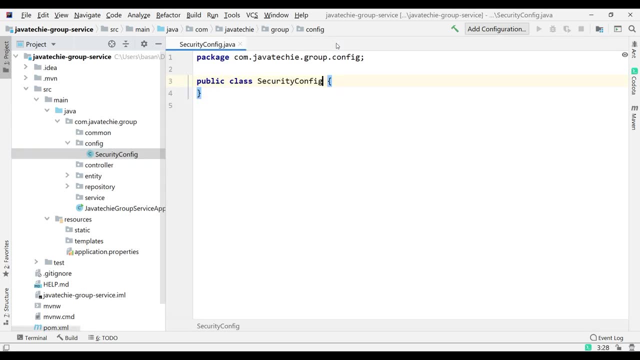 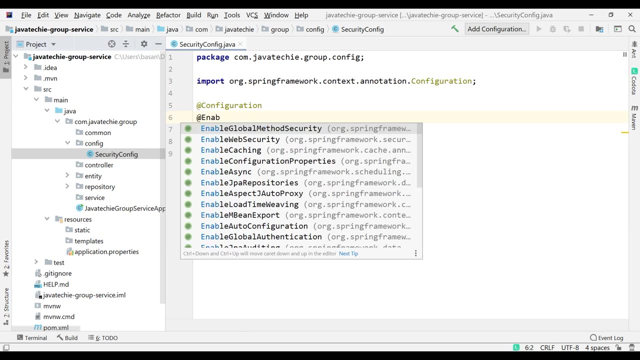 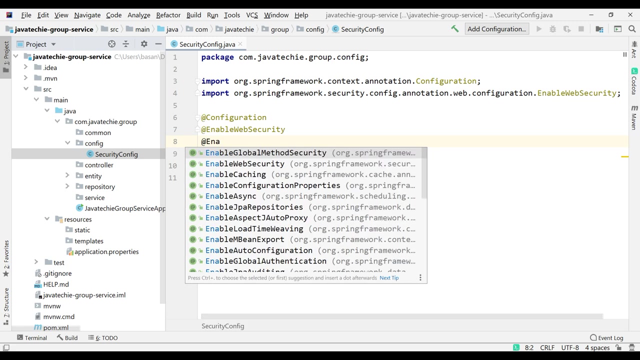 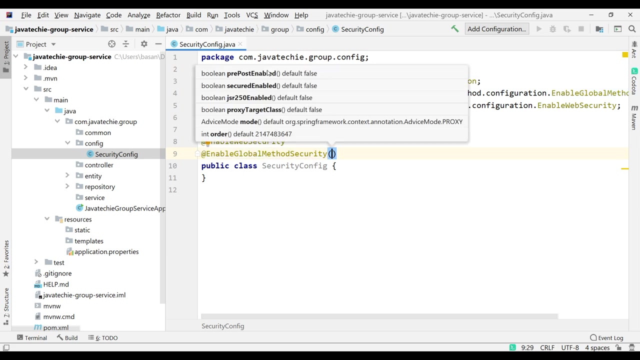 create a class called java security. i'll directly specify security config. we need to annotate this at the rate configuration. then we need to annotate enable global method security or enable web security. also, we need to enable global method security. okay, inside that, we just need to specify the authority. 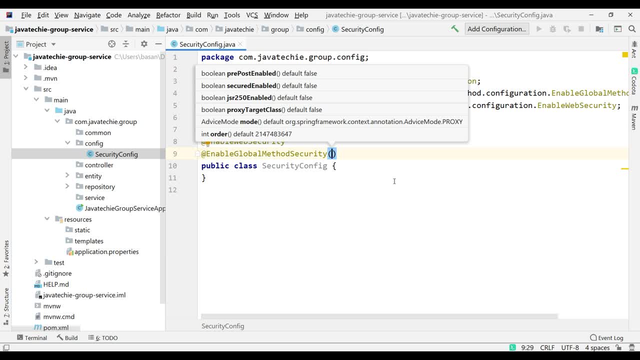 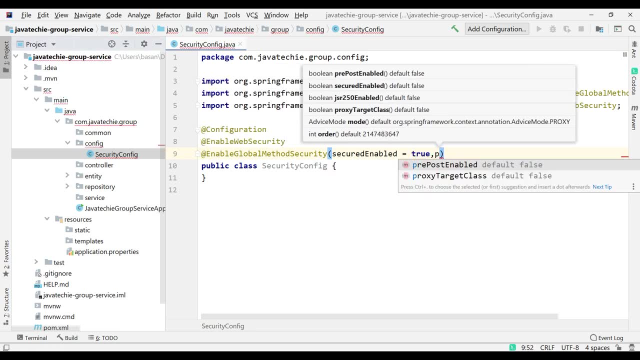 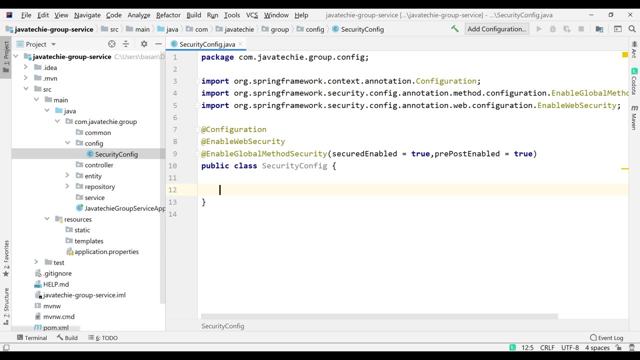 role right. so based on the role, user can access the api. so that's why there is something called secured enable- make it true. and pre post enable: make it true. fine, now here we just need to overwrite the configure method. but to overwrite the configure method, we need to extend. 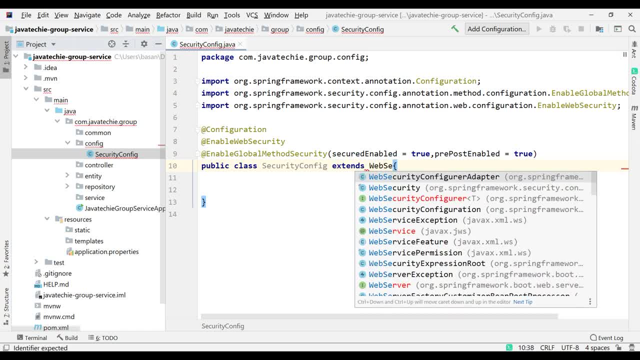 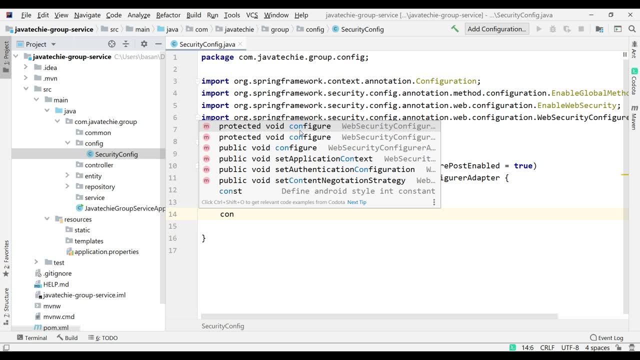 this class from web security configure adapter. okay, then you need to overwrite the configure method. so if you observe here there is three overloaded configure method, right, so the purpose of each method is different, so we will use order method rather than the standard method, these three methods. so as of now i will implement the second one. okay, so just overwrite this. so if 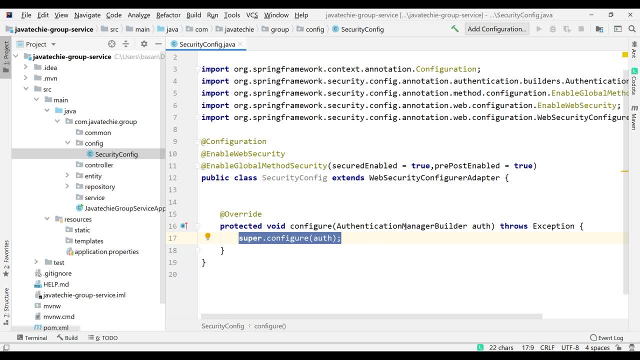 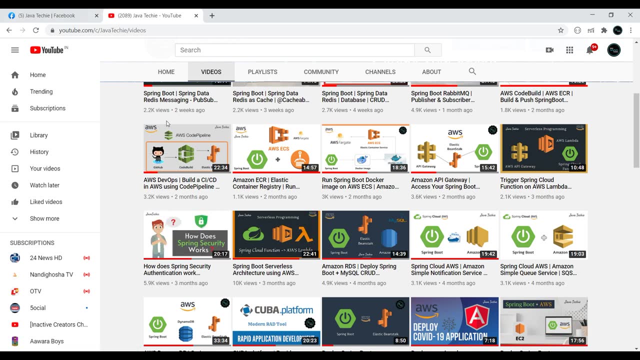 you observe here there is a authentication manager builder. with the help of authentication manager builder, we can authenticate a user. so if you are not aware about spring internal flow, spring security internal flow, you can check out this particular tutorial. okay, how does spring security authentication work? so if you understand this, then it will be easy for you to understand. 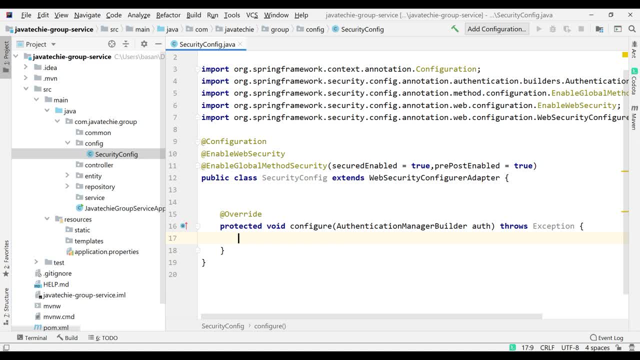 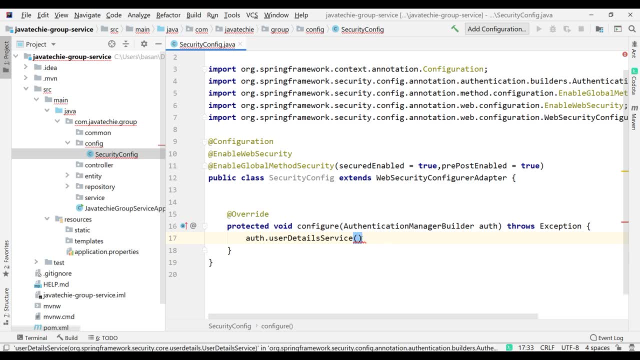 so what we'll do here? just remove this auth dot user detail service. and here we need to pass the user detail service where we need to write the logic to face the user details from our database based on the input: username and password. okay, so what i will do? i will just inject a user detail. 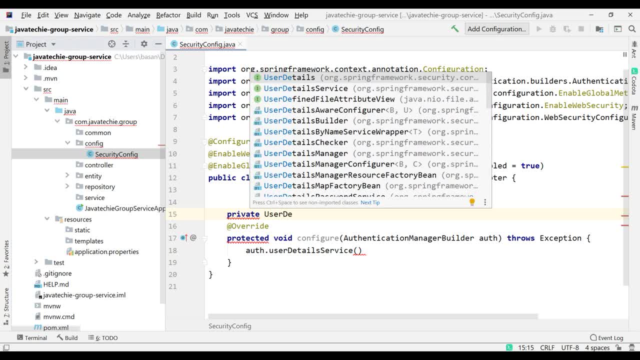 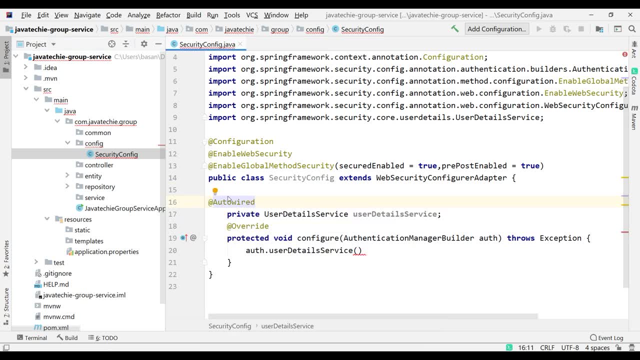 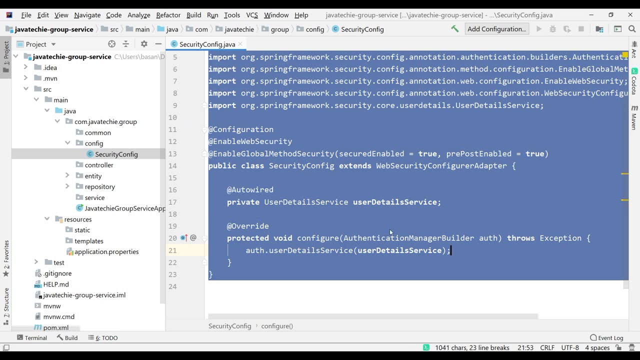 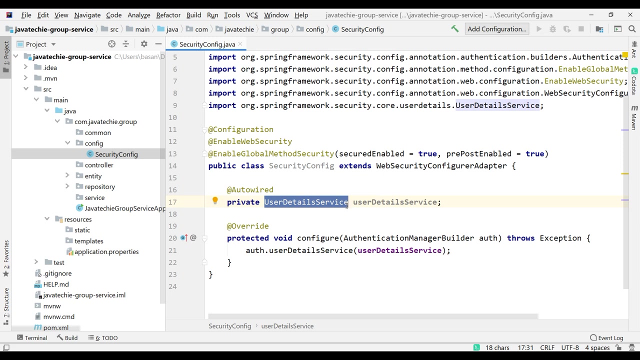 service class, so i will inject using auto add. so i will inject using auto add. same user detail service i need to pass here. okay, fine, now we need to create a implementation of this user detail service where we need to inject our repository so that we can interact with our 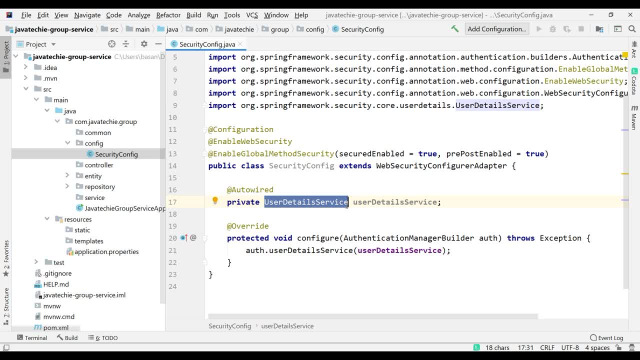 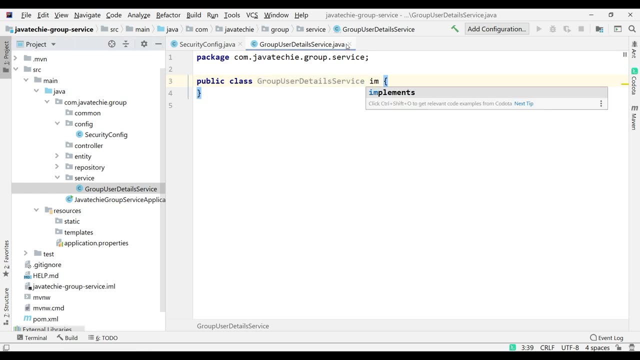 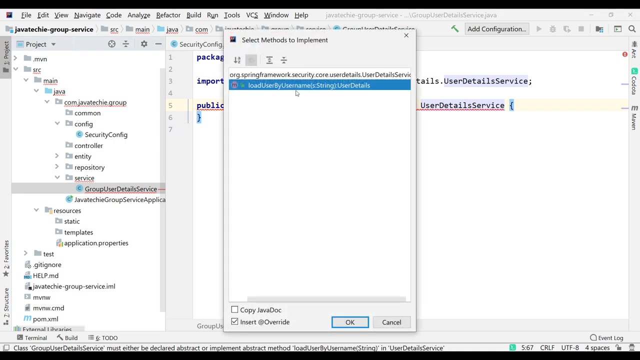 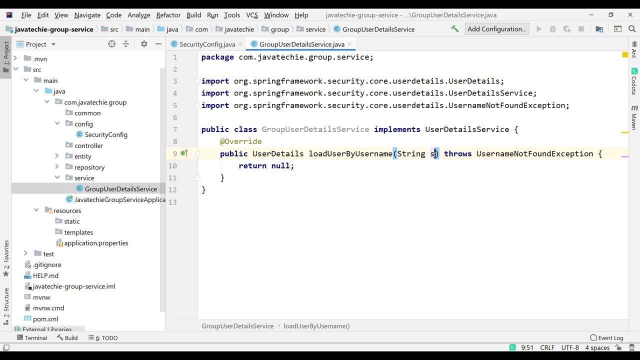 database and we can load the user based on the user input. okay, so what i will do? i will just create a class here. i will name it group user detail service. so then implements it from user detail service. okay, now we just need to override one method. so if you observe this method, load user by username. okay, so this will be your username. 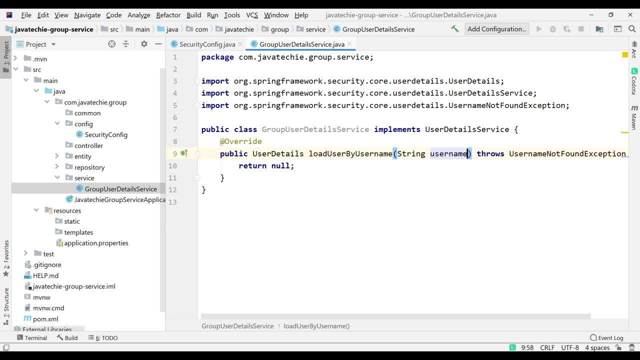 which will pass from the spring security. then, based on username, we need to go to our database and we need to load the user. then we can verify whether that particular user is exist or not. right? so for that, what i need to do, and i just need to inject the repo here, right? private user repo. 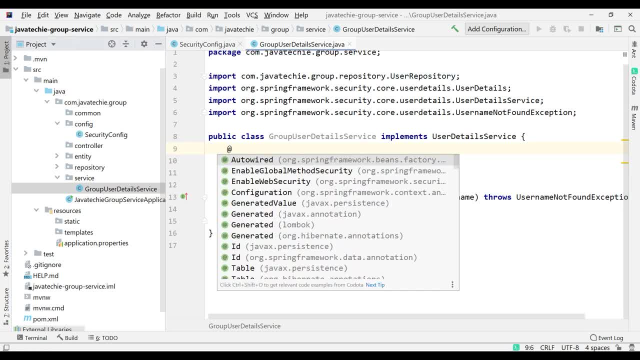 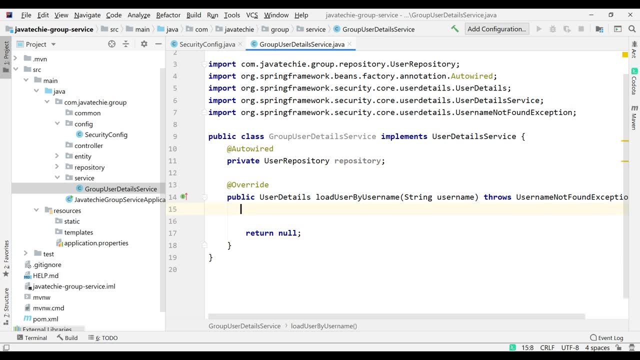 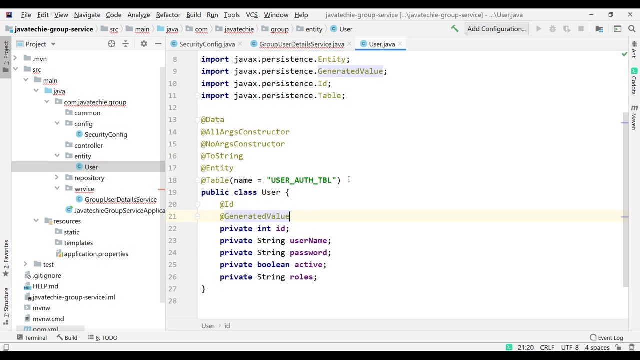 then here we just need to write a api or method to call our database right so we can directly write repository dot, find by username or whatever the field we have. so this is the format we need to write in spring data jpa. so just go to the user and the name we specify: username right, find by: 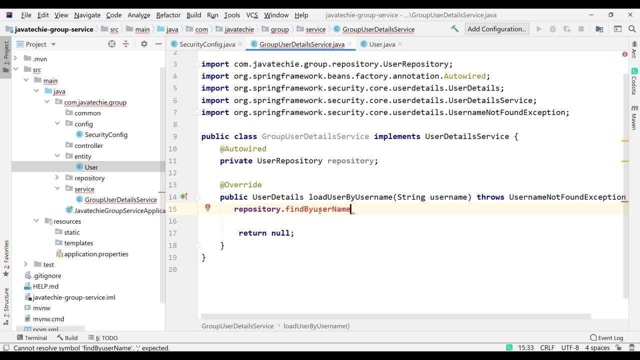 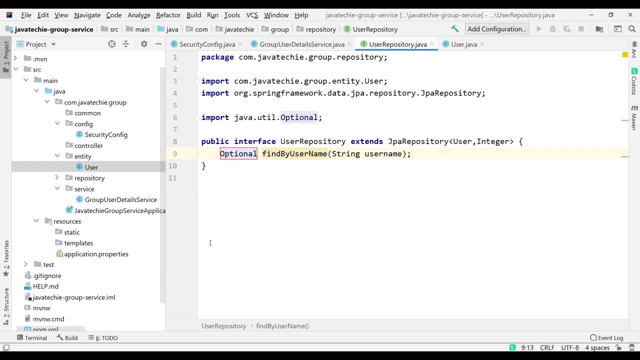 then field name we need to specify, so it should be capital- then pass the username. now let's create this method in our repo so let it return optional of user. fine conv end, and let's just change it now. let's do the change in our service so add the return type. 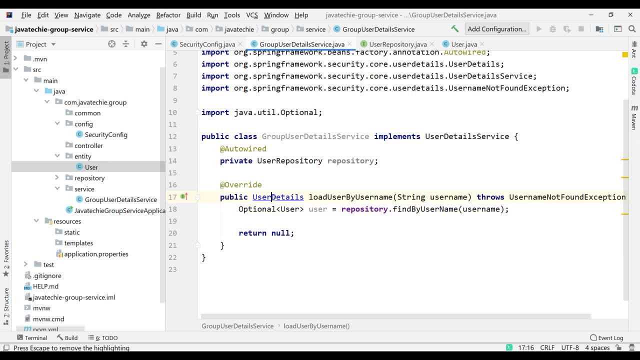 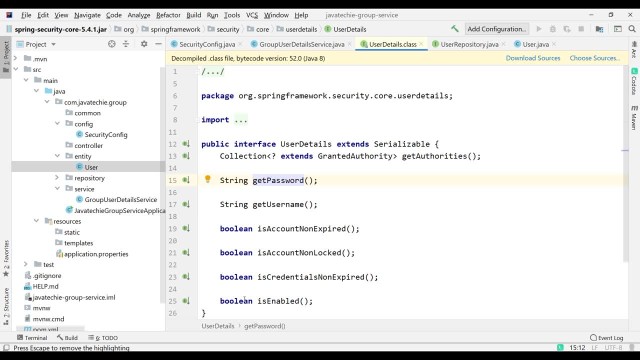 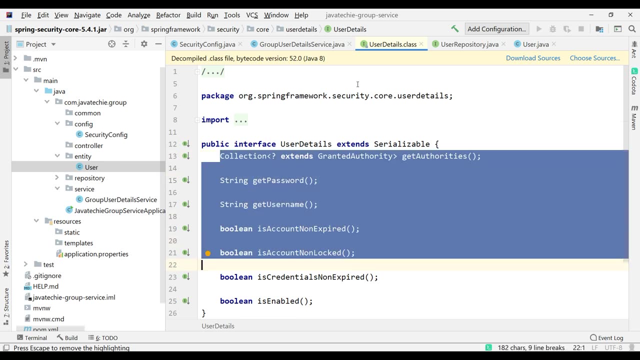 user. okay, but if you observe your, the return type of this load user by username is user details. so if you go inside this user details, it will have the password, username and whether your account expired or not, account logged or not. these are the field we need to pass. we no need to pass the user object directly, right? 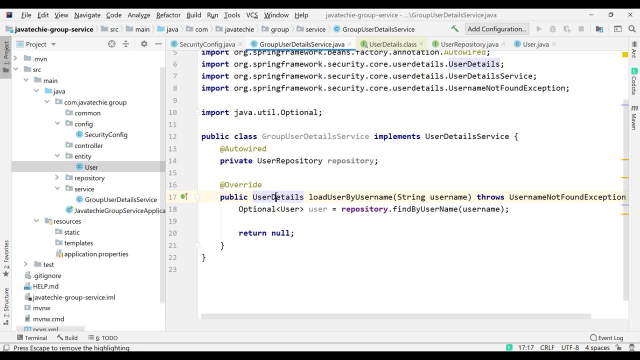 so we need to convert our user object to this user details object. that's the reason what we need to do. i will create a class. this is also an interface, so i will just create a class- user details. so i will name it: group user details or something like that i will. 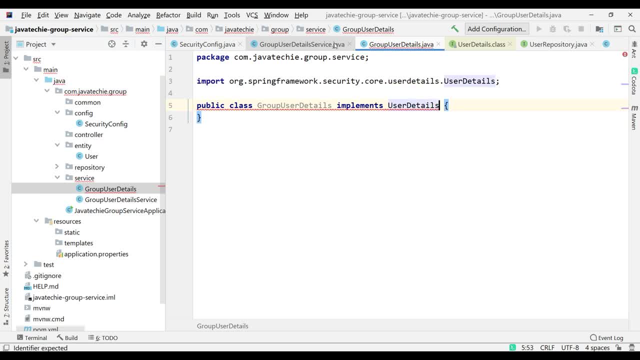 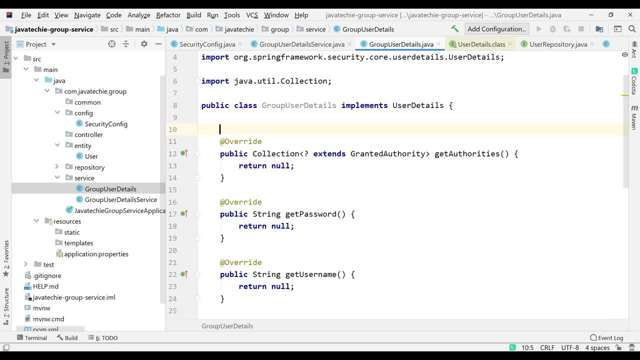 implement it from user details. now i will overwrite all the method. fine, what i will do? i will just create a constructor and i will pass the user object directly. okay, from the user object we will set all the value. so i will write a constructor, public group user details. i will pass the user object. 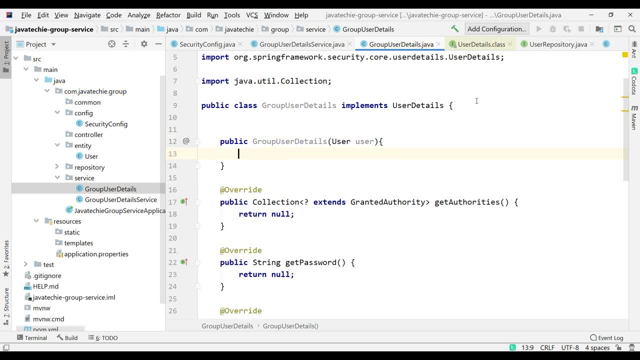 now what i will do. i will just declare few field, so something like password, username and authorities. so, based based on that, we just need to set in the method return type. okay, so i will name it: private string username. private string password. private boolean is active. private boolean is active. 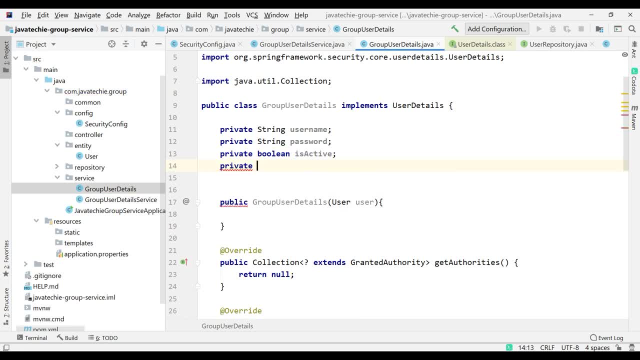 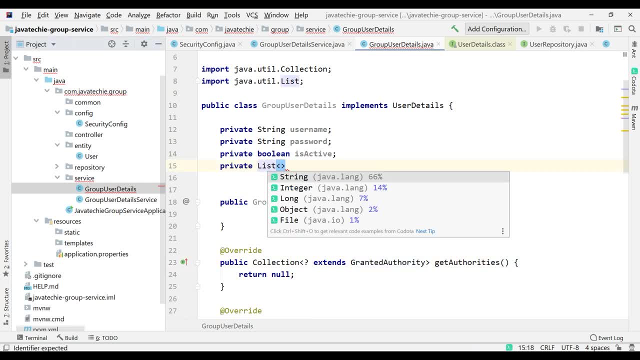 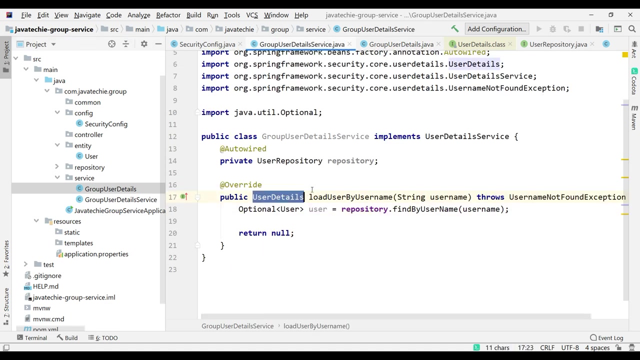 tricky. we will do control v. i didn't copied it. fine, now what we will do. this is what we will do in this version. we will do the first one: user name dot. user name dot. user name, user dot. get user name right. so this particular local variable i am assigning to the user which i get from my database. 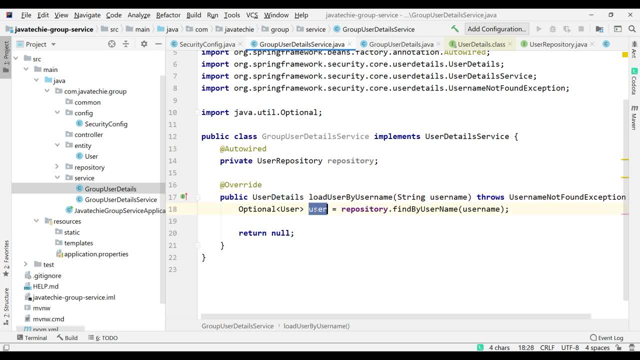 because ultimately, i just need to convert this user object to user details. that's what spring security understand. spring security don't understand your own user object. you will always search for the user details. so that's what i explained. so that's what i explained in that internal security flow video. you can check that once. 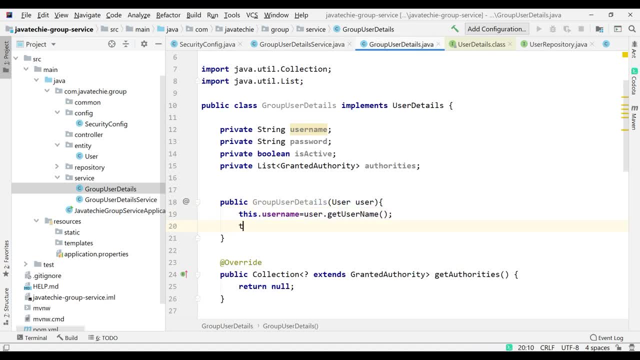 okay, similarly initialize all other fields. this dot password equal to user dot, get password. then this dot is active. equal to user dot is active. now the tricky part is this one, this authorities. because if you observe in our entity class the role we are storing as a string, so the role can be something like: 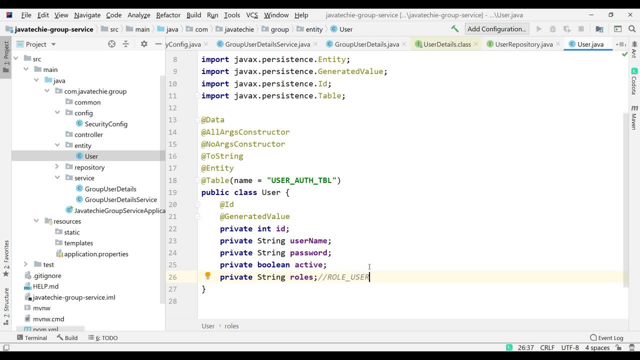 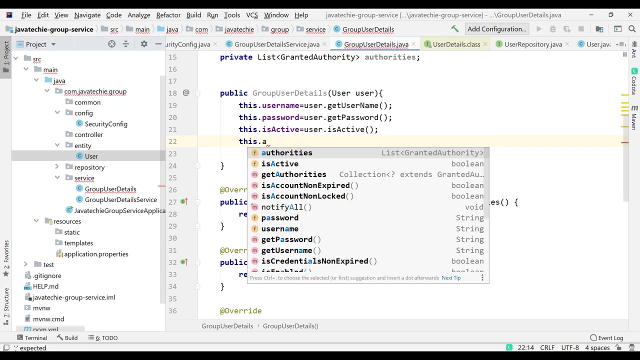 this role underscore user. even a user can have admin access role underscore admin, like this. so we need to split this string and we need to convert it to the collection, right? so what we need to do for that go to the group details. so here what we need to do: this dot authority. 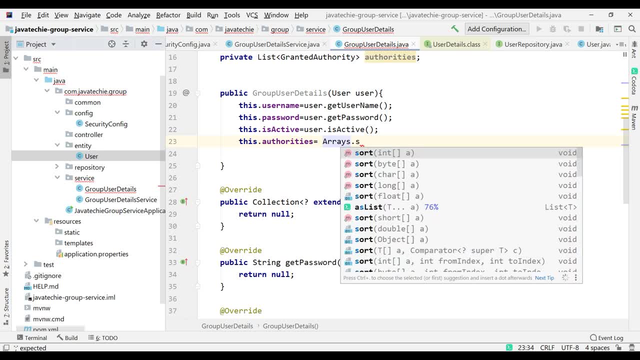 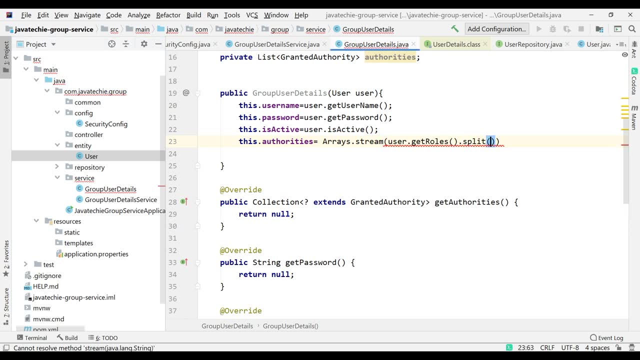 dot studios dot utilities equal to RS dot. stream of user dot. get rule dot split. you need to split using comma, right? that's how we are storing in our database. then we just need to map it to simple grant authority or um, yeah, then we just need to convert as a live locationаш this of me temporary file following down: 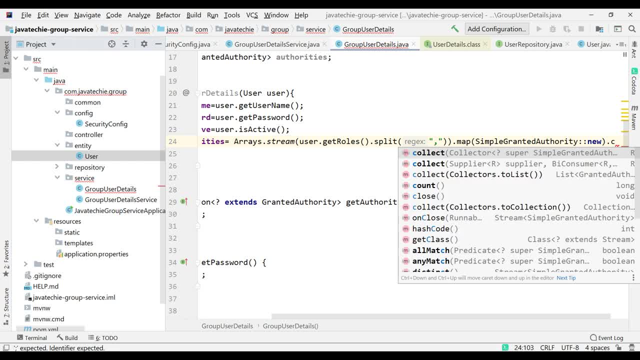 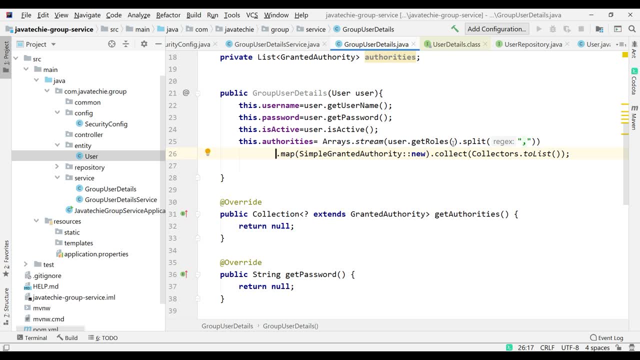 a name today. so it is how this is everybody simply emphasising it? okay, and if you have an account, you can also do that. we are really satisfied in the list. fine, so let me format this. yeah, so the role i split based on the comma, then i convert that. 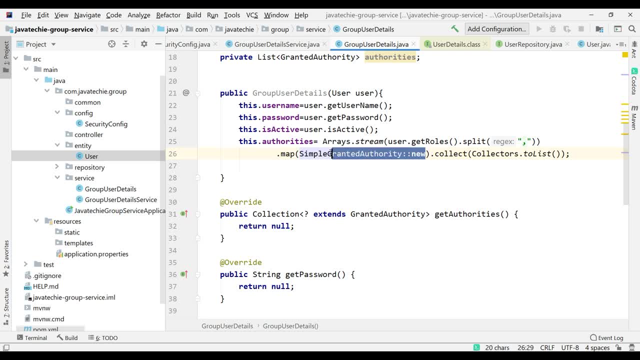 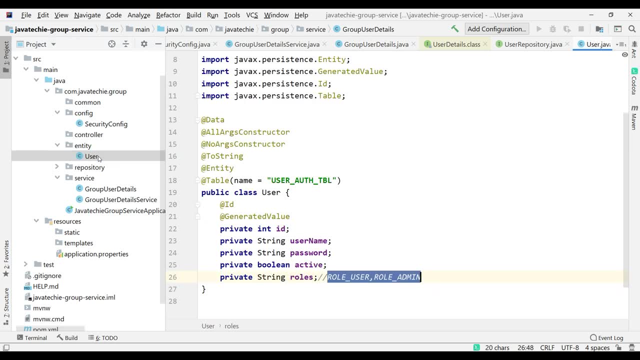 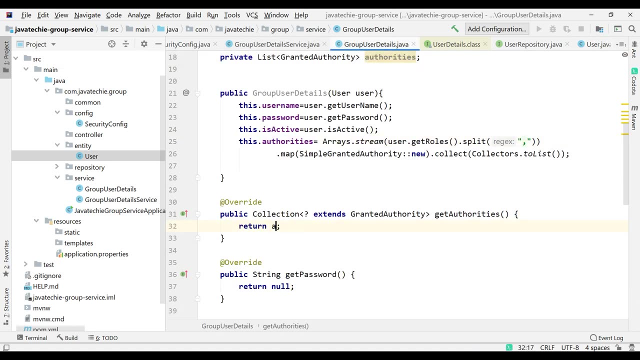 role to the simple grant authority. i created this new object, then i convert that to list. okay, now these authorities will be store these two list, these two role. so this one role, user, and role admin. that's how i designed it. now, what we'll do? we'll just return it authorities. 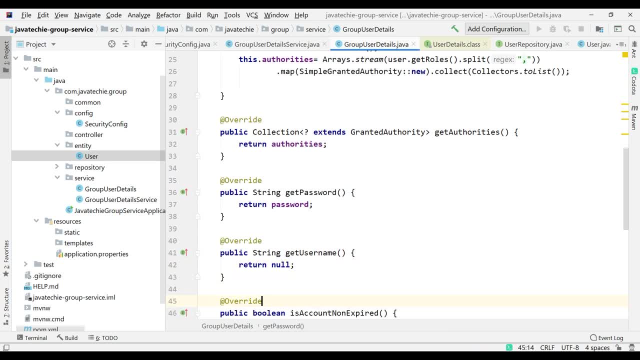 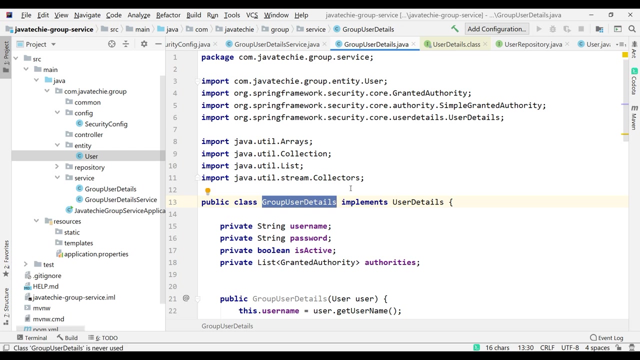 and password, then username. so let it be true. we don't want to assign this value. make it true and this is enable will display as a is active. format it fine. now what we did here: we just convert our user object to user details object, which is group user details. right now let's go to our group user details service class. 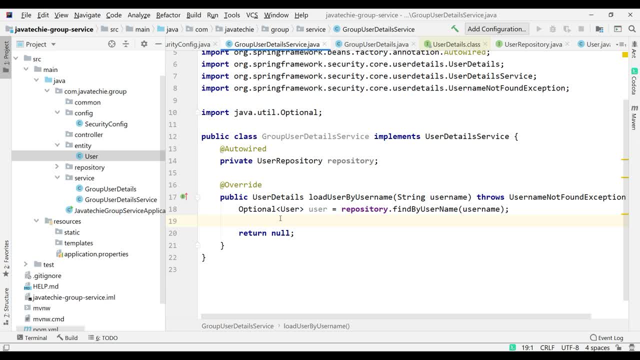 and here we just need to call that method right. so just simply do this user dot map. okay, then our class. this is what the group user details we created right. this user object we want to map to this group user details. that's how i did this, so just. 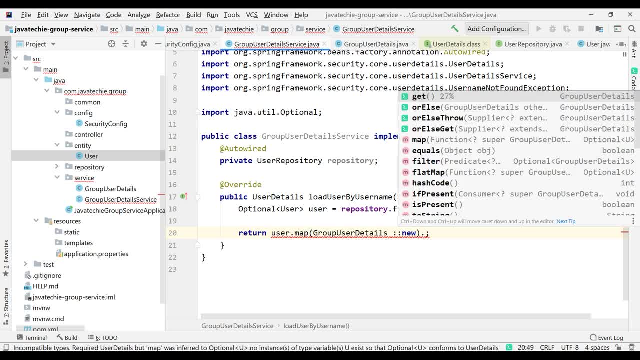 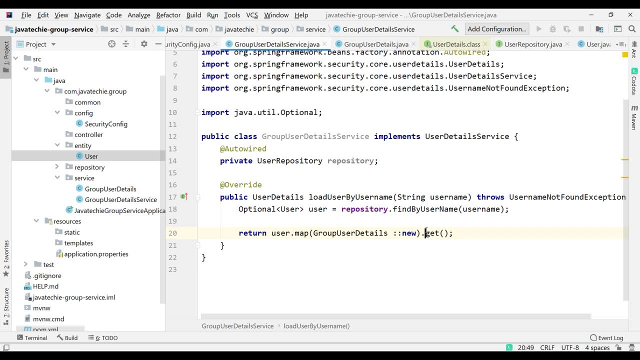 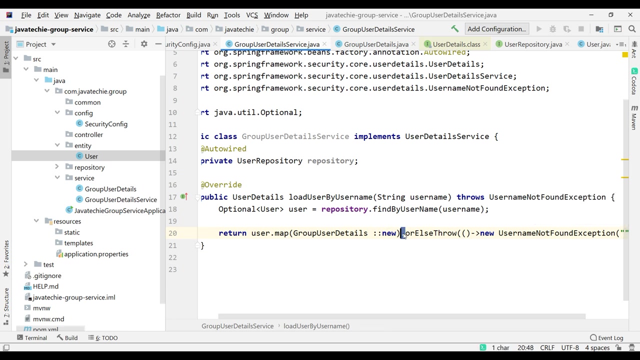 add it here, then get it. but if this user is not exist, then what we need to do before that i'll i'll directly not return, i'll do here or else throw new. this user not found exception. okay, so i'll return some message here. so let me format this. 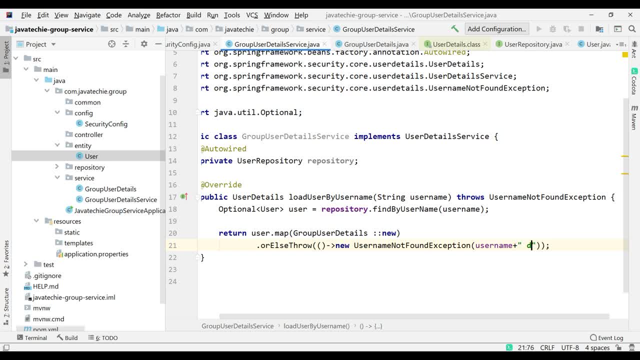 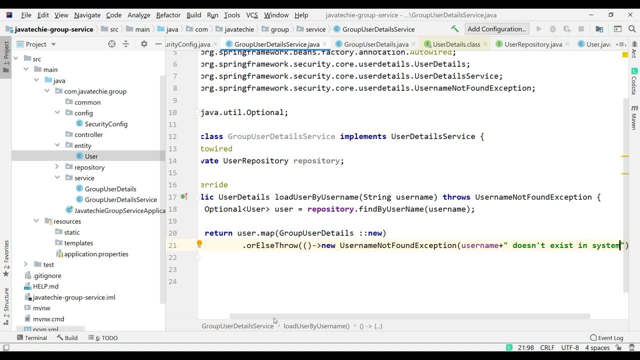 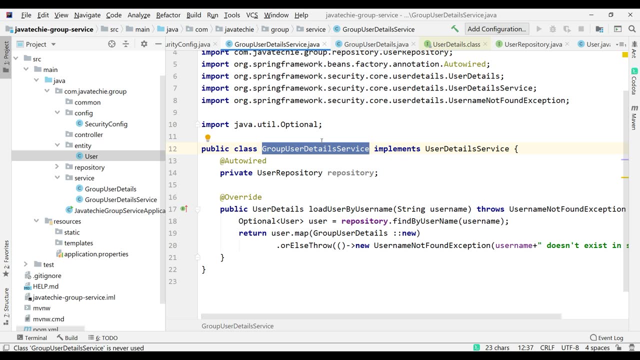 username does not exist. something like that exist in system. it makes sense, right? fine, so we created our own user detail service where we can authenticate a user based on the username. so while login i need to pass the username and password. based on the username, i'll load the user object from my database. 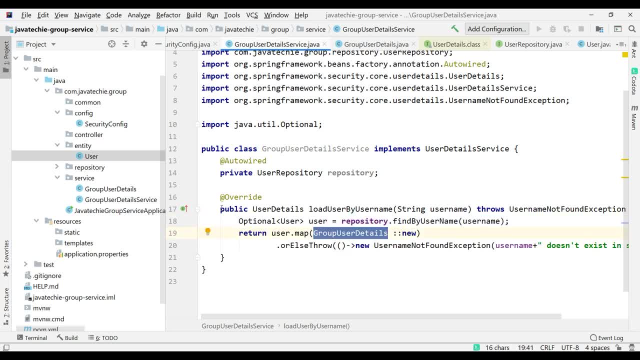 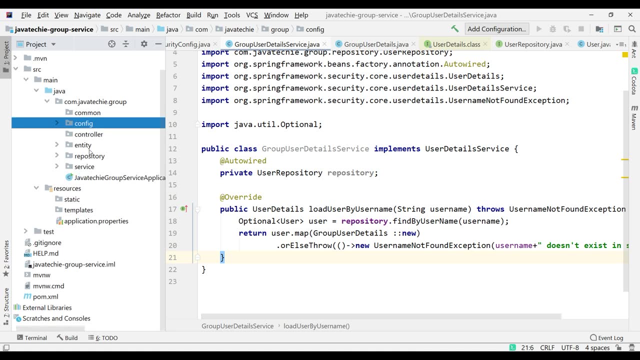 then i will convert that user object to user details object. i will return it so that it will set to my spring security context. okay, fine, so we created the config and we created entity repository and we wrote the authentication logic. right now let's write the endpoint, then we'll. 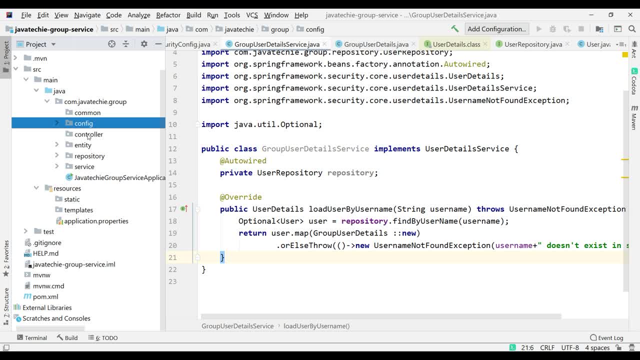 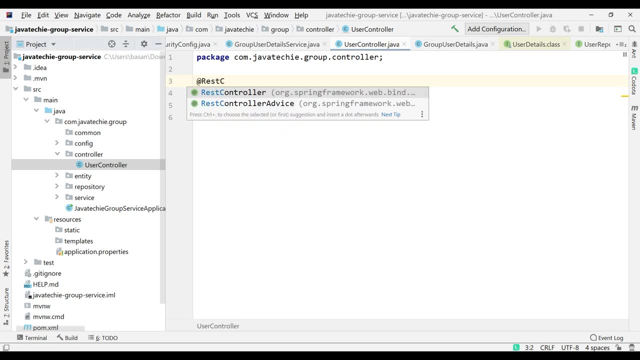 specify the method of authentication. right, this is the бли称 delicacy, the role and authority who can access my API. okay, so what I will do? I will just write a class in controller, Java class, and name it user controller. then we need to annotate this with, at the rate, rest controller. fine, then I need to annotate: 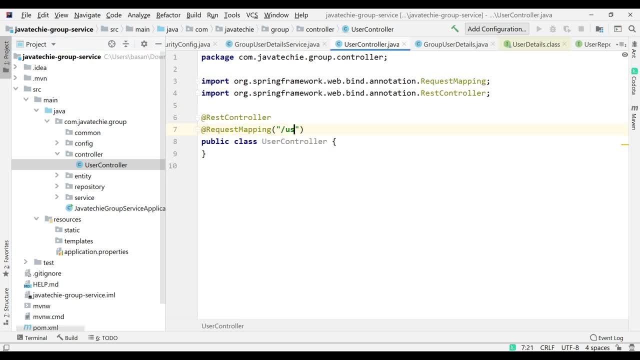 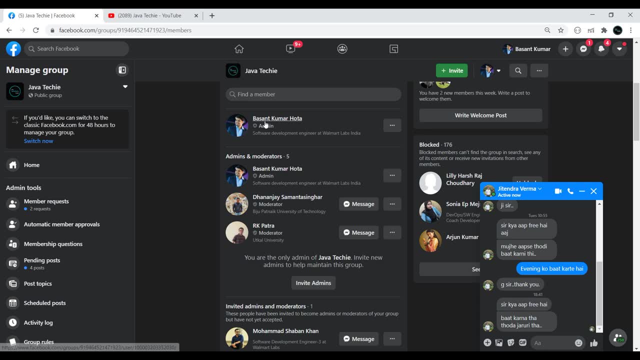 at the rate request mapping, I will specify the root URL as a user: slash user. okay, so, as I explained, there will be two API. I am going to write once the user need to onboard to this group with the role by default- user role- and then I have. I need to write one more API to give the access to that particular user. 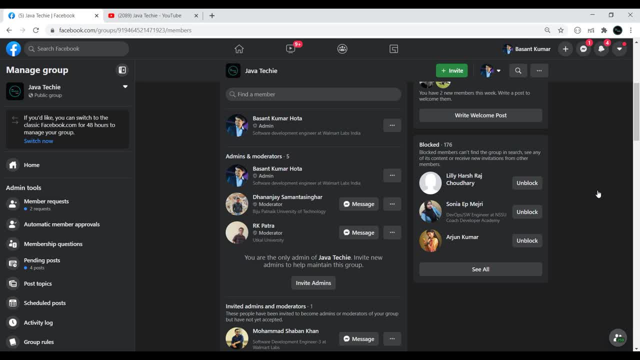 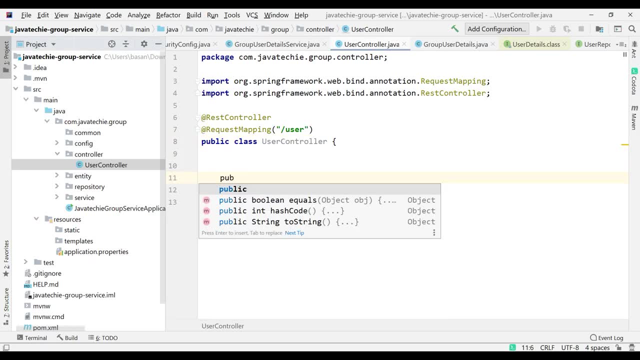 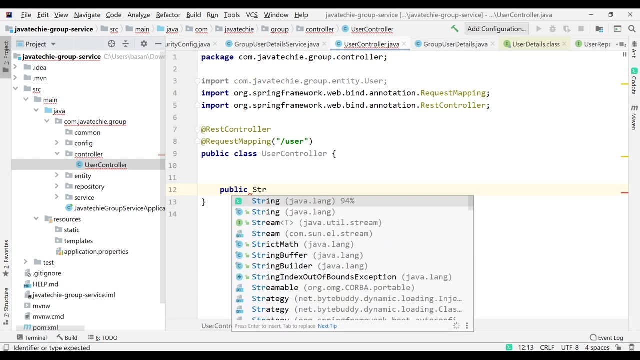 either as a moderator or either as a admin. okay, so these two endpoint I am going to write here, so public. then I will return the user object or else I will simply return the string object: join group. okay, so this will be my post method. so I will annotate at the 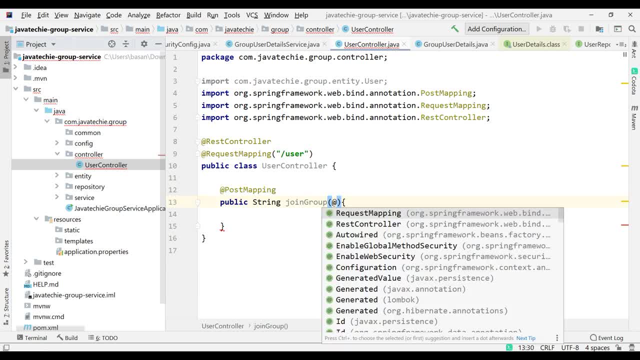 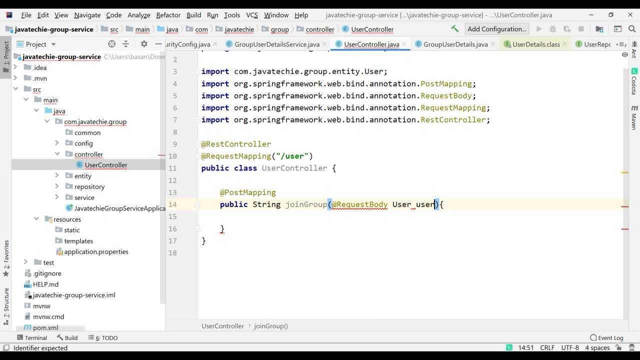 rate post mapping. then I just need to pass the request body annotation and I need to pass the user object which I want to persist to my database. so I just want to interact to database from this controller. so I just need to inject the repo here: private user repository inject using auto add. so now what I can do, I 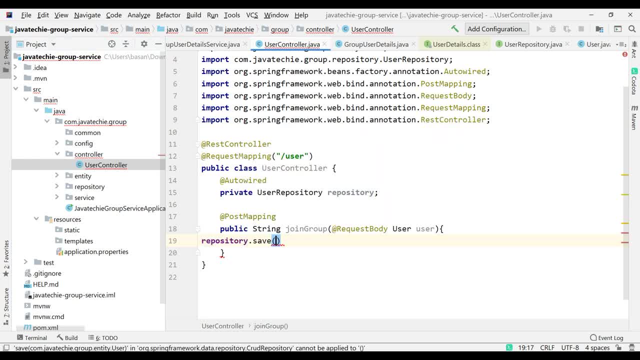 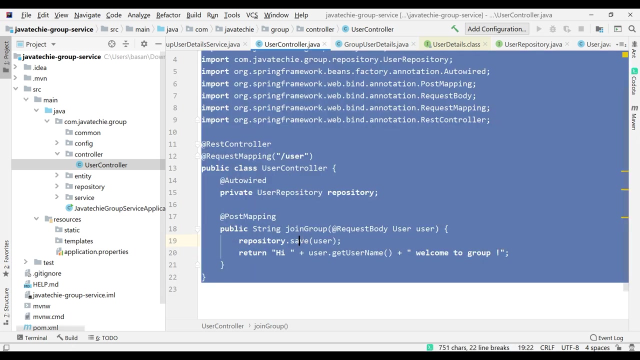 can directly use repository dot save and I can pass the user object right and I will return some string, something like this: user dot: get username welcome to group or something like that: right, welcome to group. fine, but if you go to this user class we have a field called password. I don't want to store the 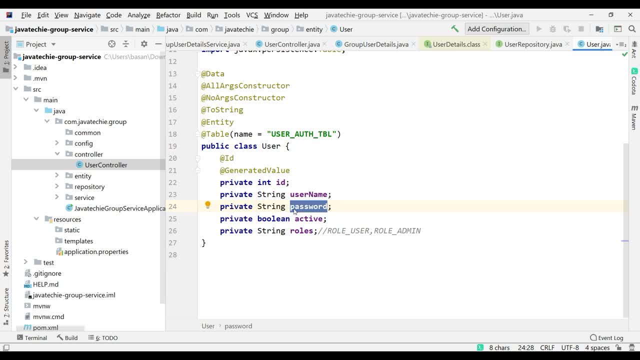 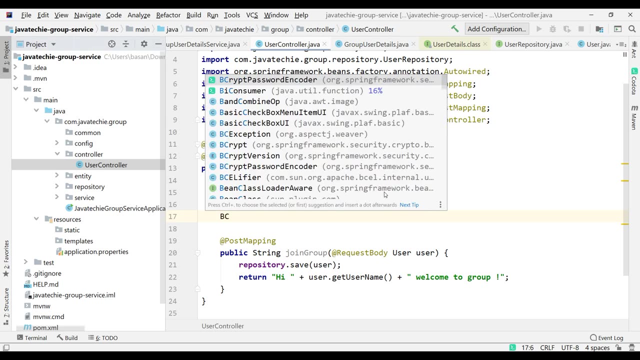 password in hard code format. I just want to encrypt it right and also by default, I just want to assign the role as a user. that's what we just need to modify here. so go to this user controller to encrypt the password. there is a class called BeCrypt password, so declare it as a. 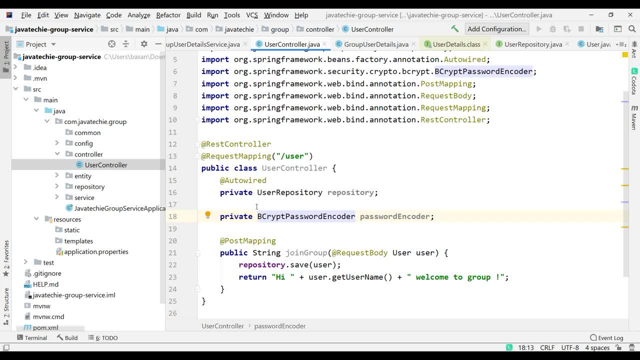 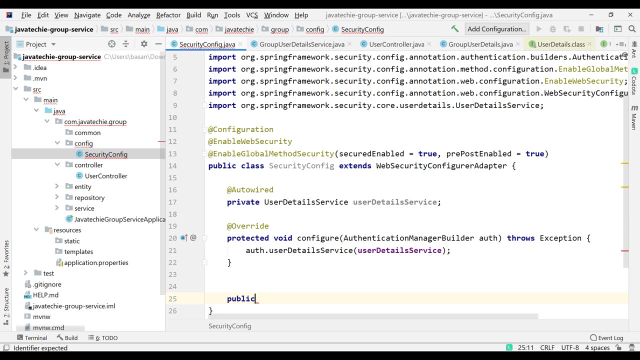 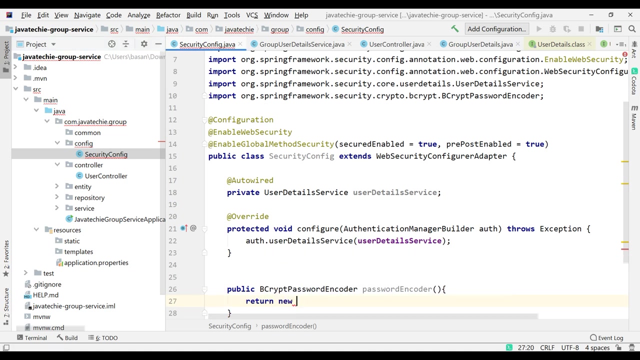 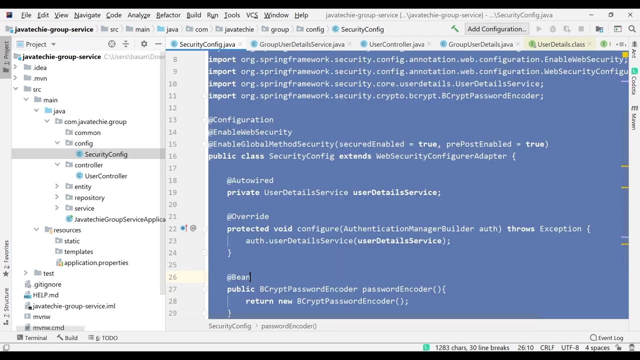 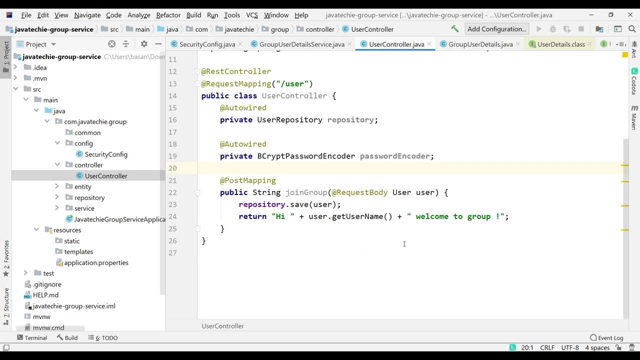 private, then I just need to auto edit. also, I just need to create a bin of this in my config class. go to those website type: security config. I will create a bin of this class. return, new this object, just annotate at the right bin. ok, now go to this controller class. so we just want to encrypt the password. 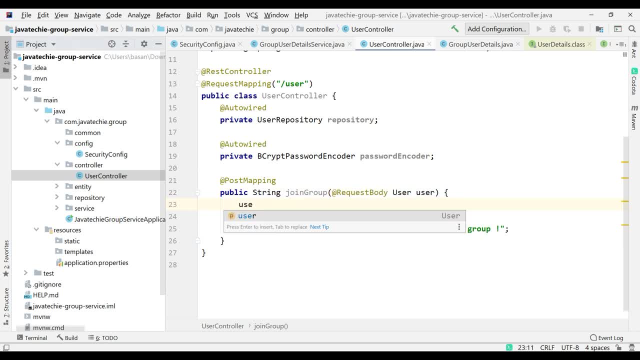 and we just want to define the default role of a user. so user dot set roles. I will specify role underscore user. ok, so let's not hardcode here. I will define as a class label variable default role, something like that. ok, it's not typing, ok, ok. 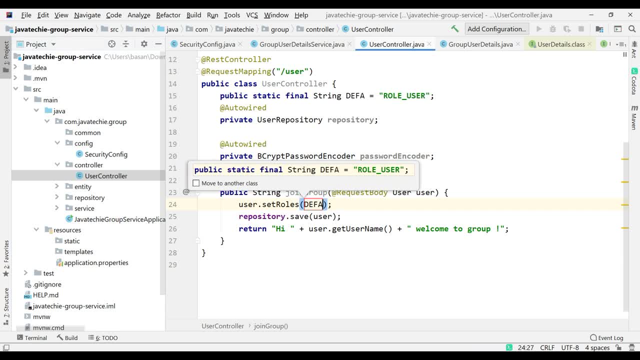 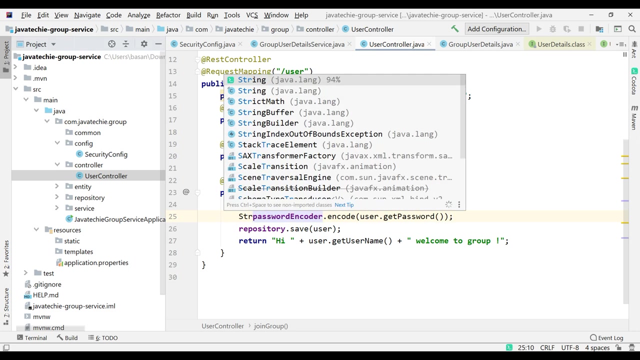 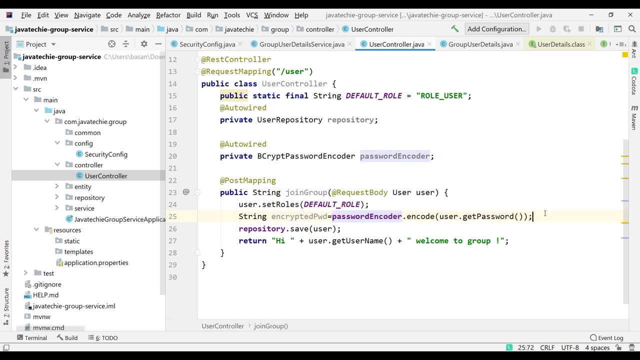 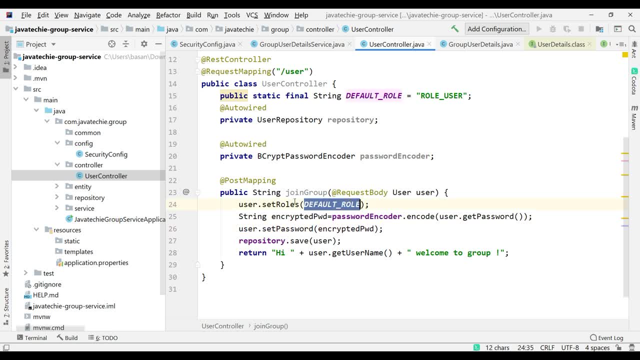 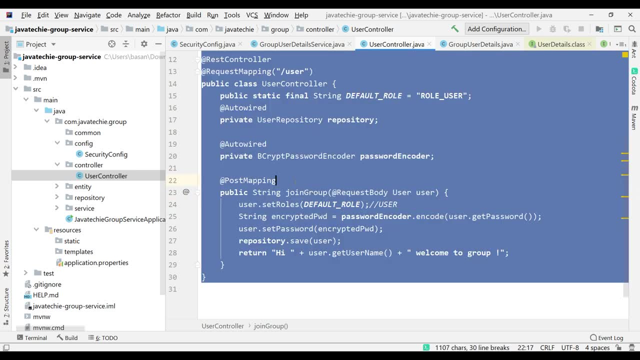 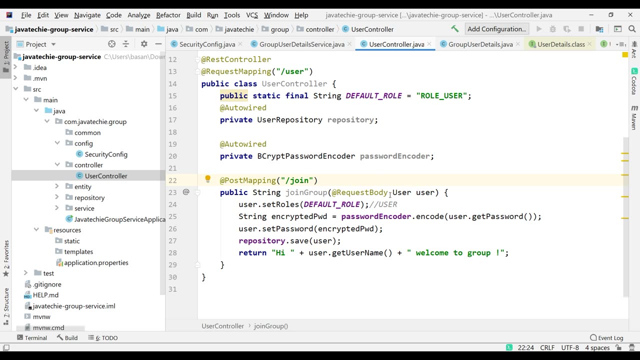 we fine, now we just need to write one more API. so in that API we just need to write a logic to give permission to the user. so I will write the condition here: if logged in user is admin, he can give two access, either admin access or moderator access. but if logged in user, 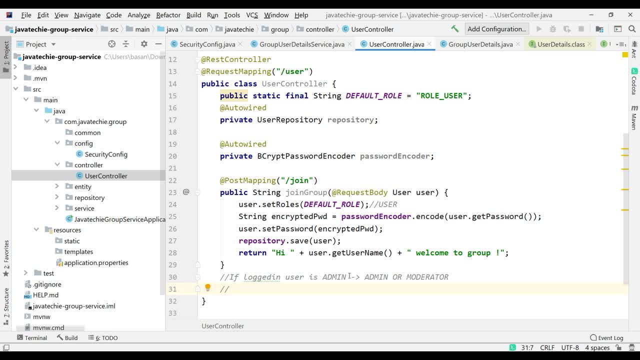 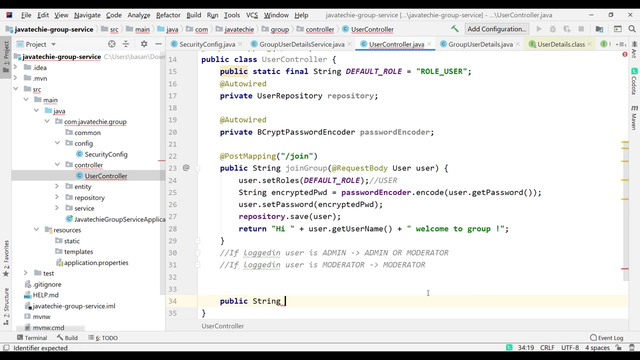 is moderator. so I will copy this: if logged in user is moderator, he can only give moderator access. ok, so this API. we are going to write the next one. ok, so let's write this: ok, it public string: give access to the user. access to user. pass the user ID. pass the role which. 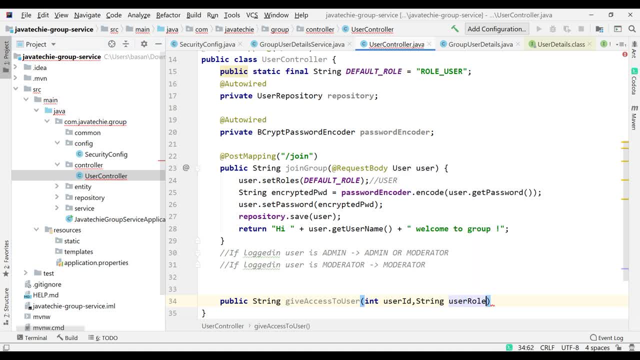 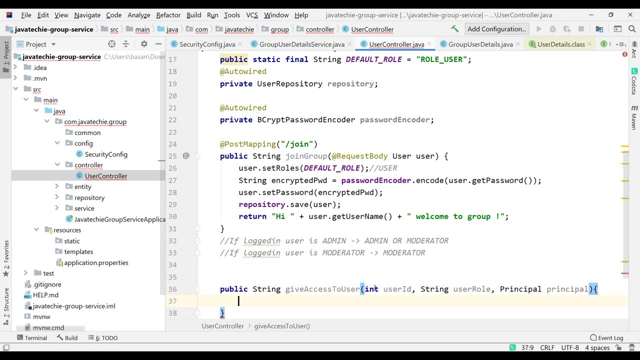 you want to provide user role? okay, and pass the principal object to know who give that access. okay, principal will always give the name of logged in user. so what I need to do, I just want to pass this value as a request parameter. so I will specify path variable, so this value also. I. 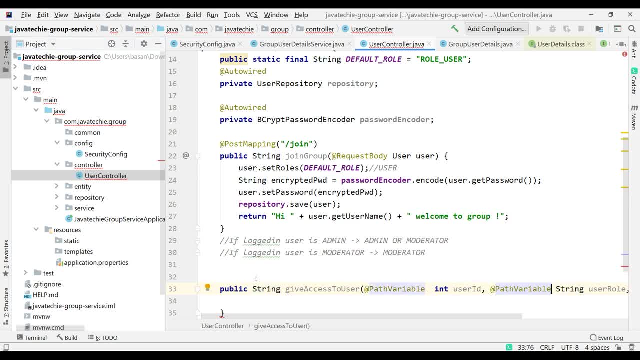 will specify path variable and then I need to annotate this at the rate gate mapping. so there is no object. I was passing as the input, so we are not going to write as a post mapping. so specify the URL: user access slash. pass the user ID, which will be dynamic parameter, then pass the user role. 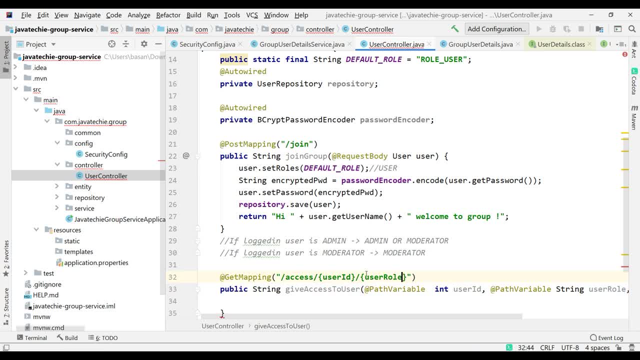 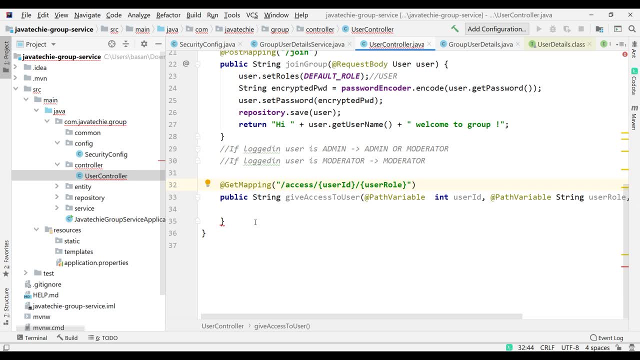 just copy this, fine. so before write this, a pay first we need to know who is the logged in user, right? so that's the reason I will write. one private method will return me the user object: get loaded. logged in user, pass the principal object. then what I will do? I will just return repository. 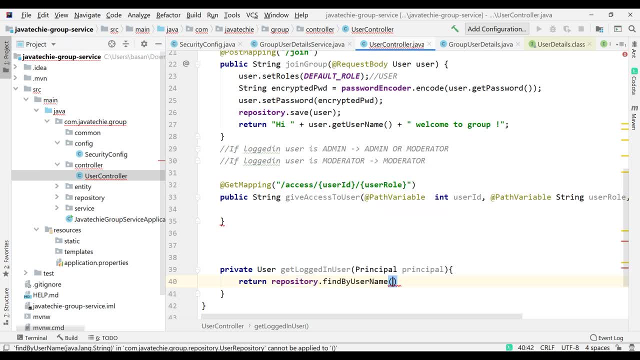 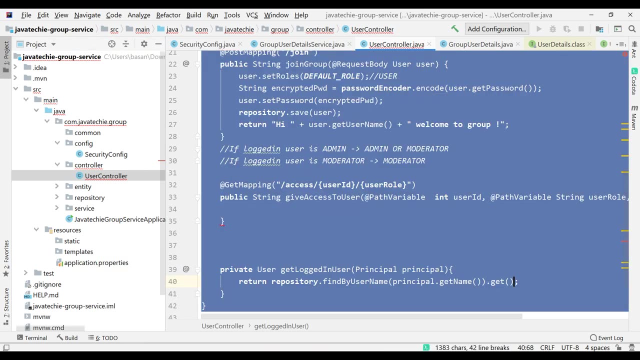 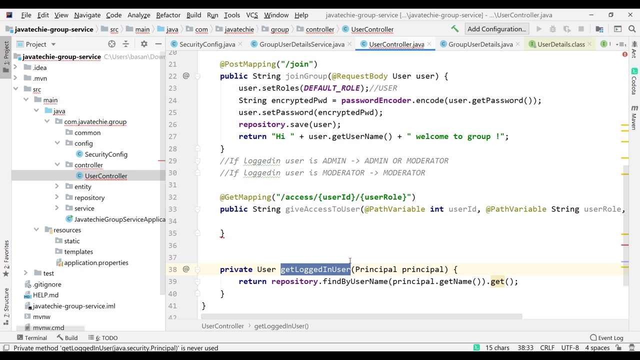 dot find by username, the username I will get from the principal object. it will return me the logged in user. so what is the okay? this is the optional, so get the object. fine, now I get the logged in user. so I should know the logged in user access, whether he is a. 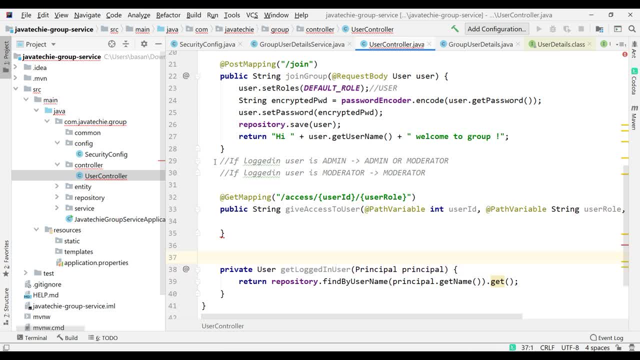 moderator or he is admin. based on that, I can assign the role to the user, right? if I am a moderator, I don't have permission to give admin access to someone. that's what the feature right? So that's why I will write one more private method: private list of string, because I just 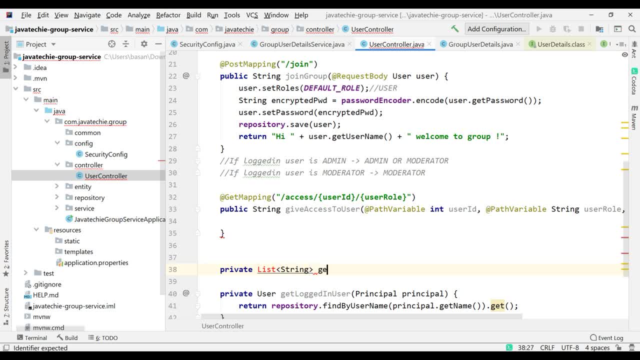 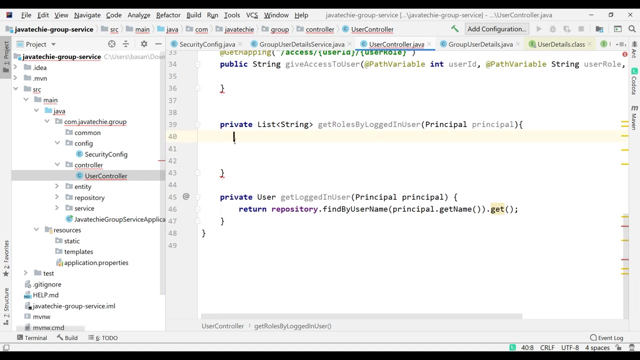 want to return the role right, so get roles by logged in user, something like that. so just input it and I need to pass the principal object here. So let's write the logic. so this is very simple. So what I will do, I will just go up, okay, so first let's get the logged in user, the method. 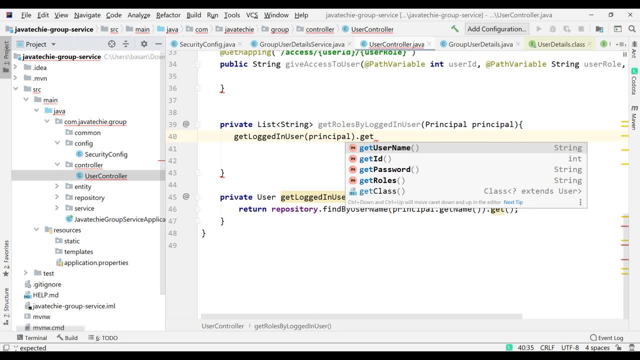 we wrote recently. then get all the roles. it will return me the role as a string, right? so string roles or something like that. then I just need to split the rule based on the command right, because that is what we wrote here, right? so if you'll go to this user, 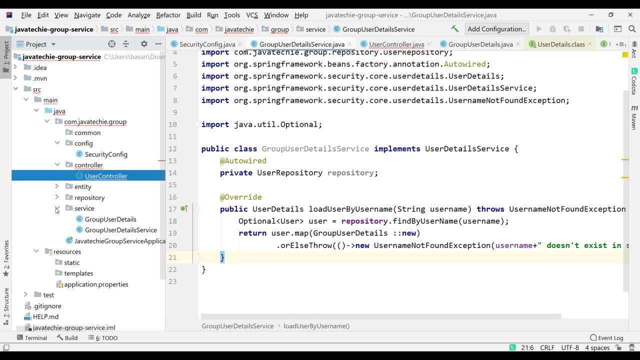 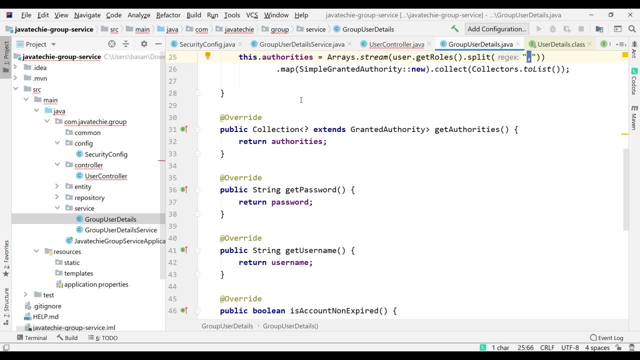 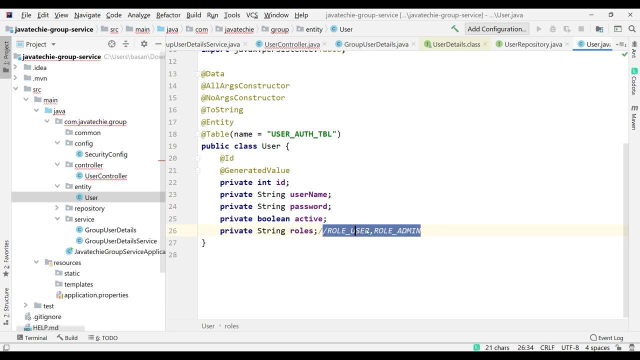 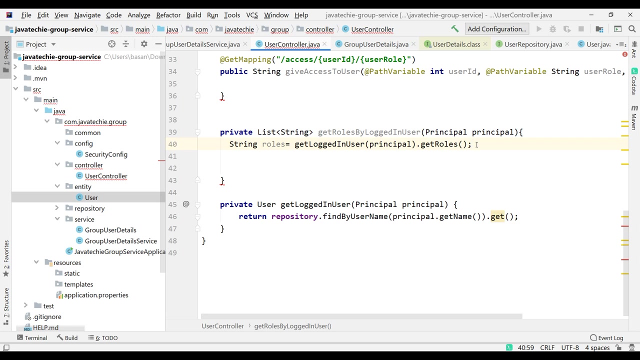 details go to this service. so this is how we just split the role, because the role we assigned like this. I already explained you in my entity class how the role will be saved in my DB like this. so we just need to split the role based on this comma. okay, so what I will do: list of string assign roles. then get the. 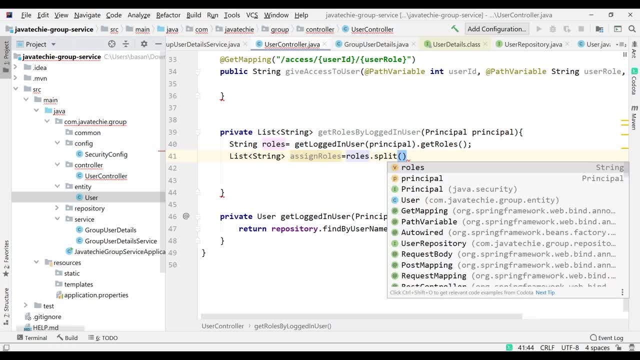 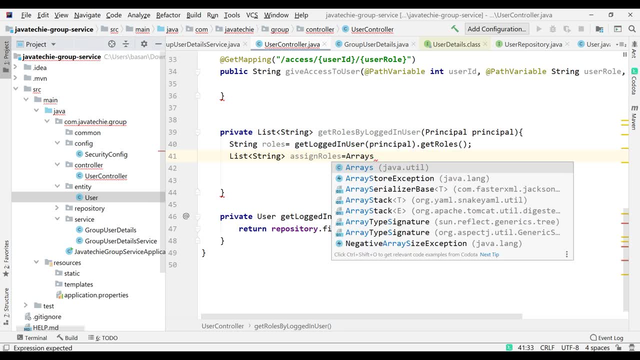 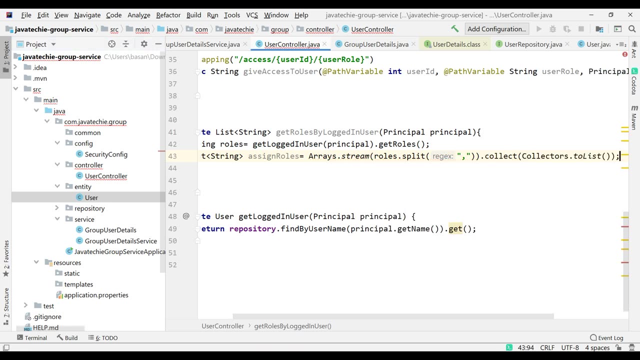 roles. dot split it using semicolon, so I will just convert it to RS dot stream. okay, dot collect as a list. fine, now what you need to do. we just need to check the role. if it is admin, then return the role access which admin can provide. okay, so, 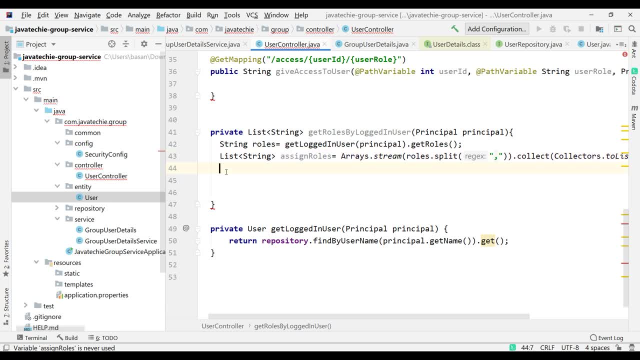 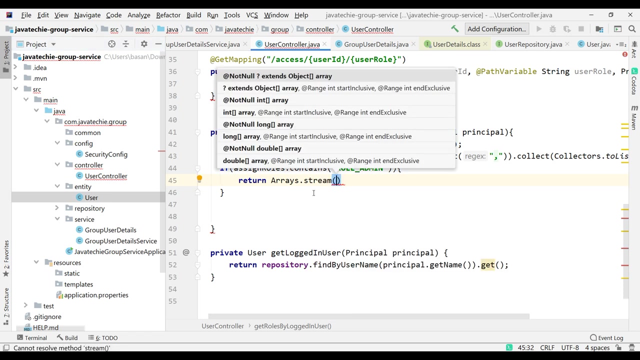 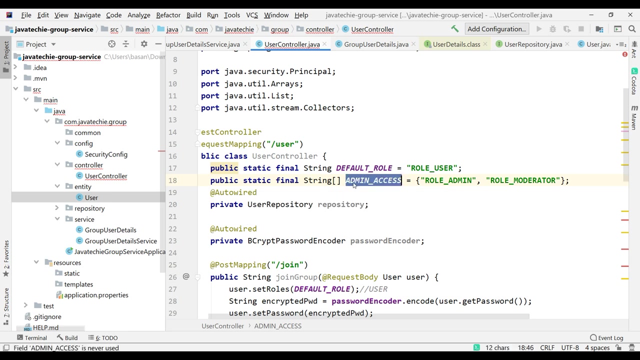 if you observe this, assign role is logged in user assign role. so what I'll do. if assign roles dot contains role underscore admin, then return RS dot stream. so what I will do. I will just declare a constant which admin can return. if the access is means if the user role is admin, he can provide these two access role: admin and 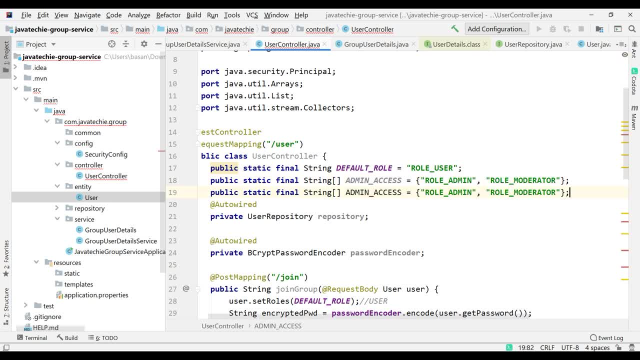 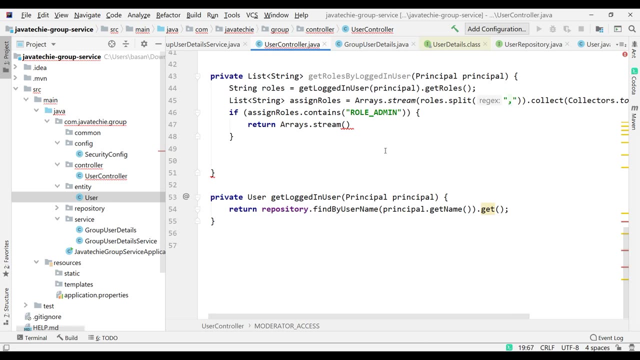 role moderator. so similarly I will add for moderator. then he can only give the role moderator. okay, so we'll write this. okay, so admin access dot list. similarly, check for the moderator. if logged in user role is contents role moderator. if logged in user role is contents role moderator. if logged in user role is contents role moderator. 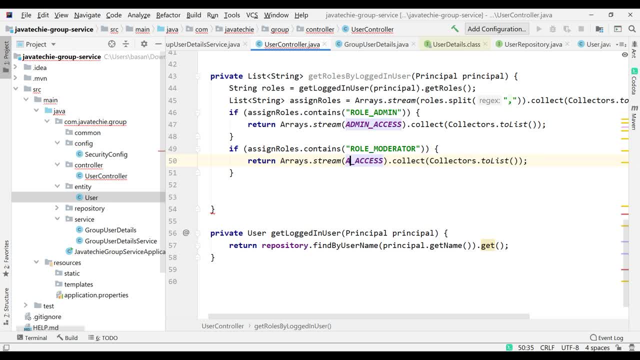 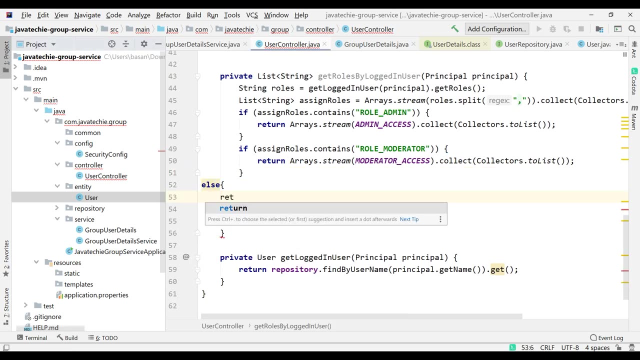 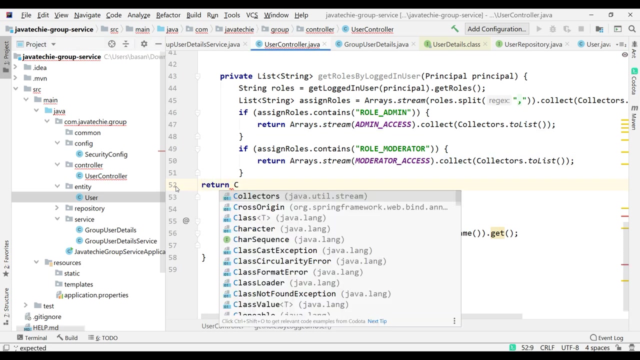 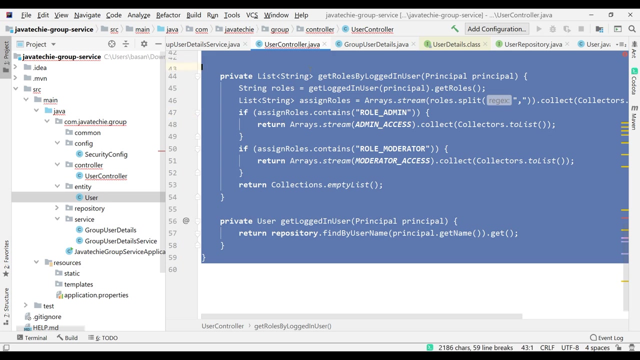 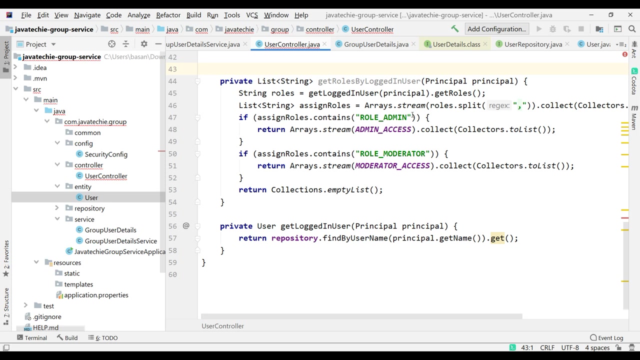 then return moderator access, fine, else just return the empty list. else not required here, we can directly return it. collections foreign. so this particular method will get the role based on the logged in user and it will just check what role this user contents. if it contains the admin, then 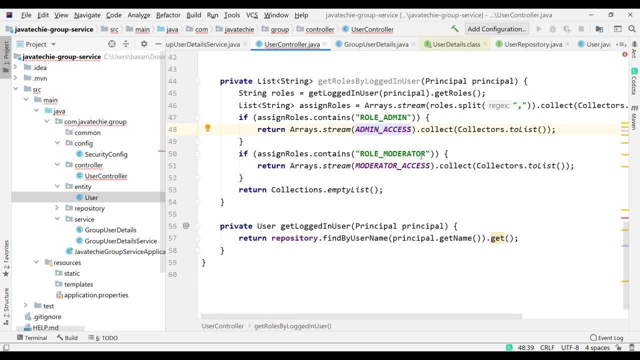 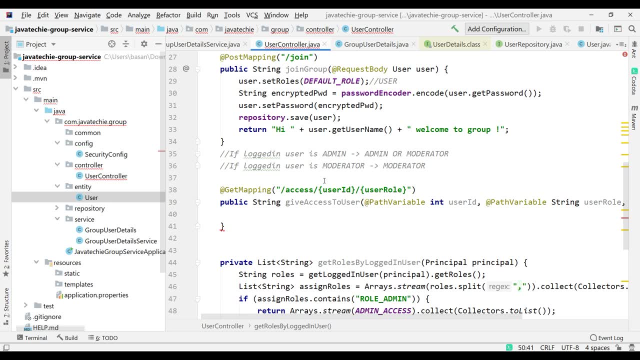 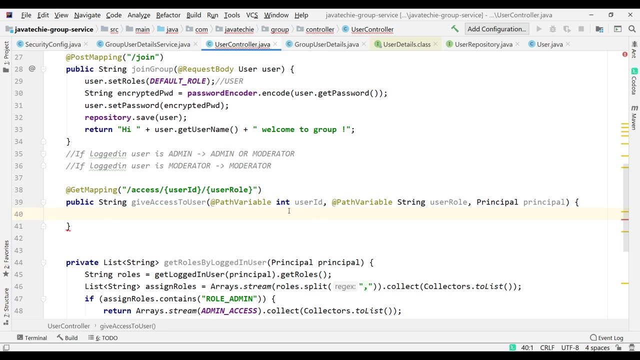 he can give these two access. if he contains moderator, then he can give these access to the user, nothing else. okay, now we just need to implement this in our actual API. so what will do? let me minimize these. first, get the existing user means to whom you want to give the permission or role. 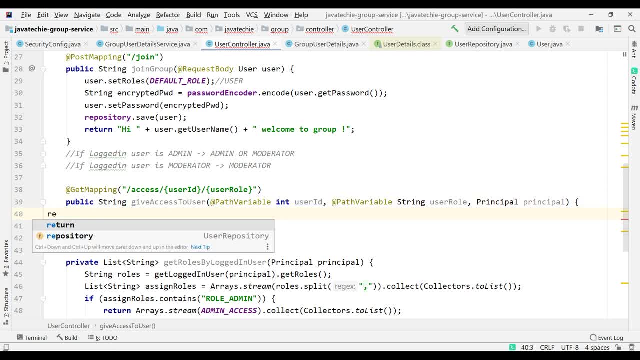 okay, so what we'll do, let me minimize these. first, get the existing user means to get the existing user means to whom. user based on this ID. so I'll use repository dot. user based on this ID. so I'll use repository dot. find by ID. give the user ID. please welcome the user ID to the user ID. it. 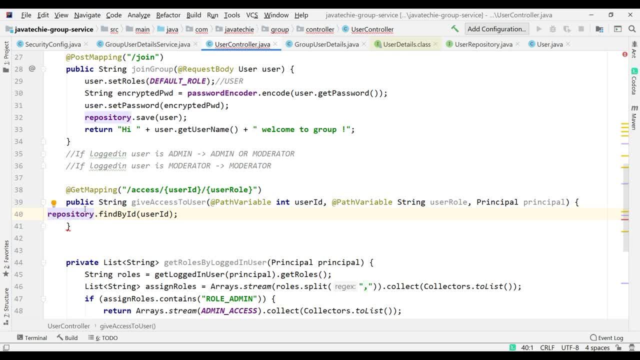 will give you the user object related log means not logged in user ID, the user area. eventually consumers will be not allowed to go through. user ID's are also Search results cloud. I second line down user ID which we are passing to give the permission. therefore, it is not that the world, the user ID has something. the idea that I am trying to 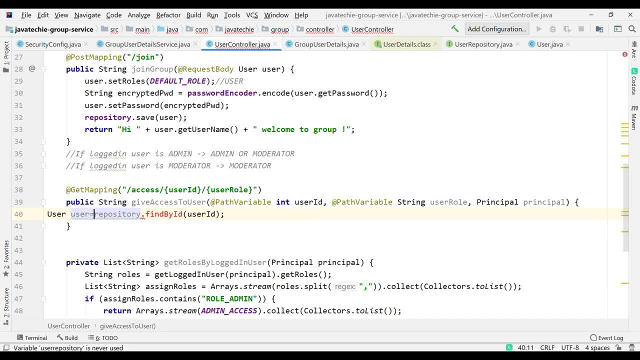 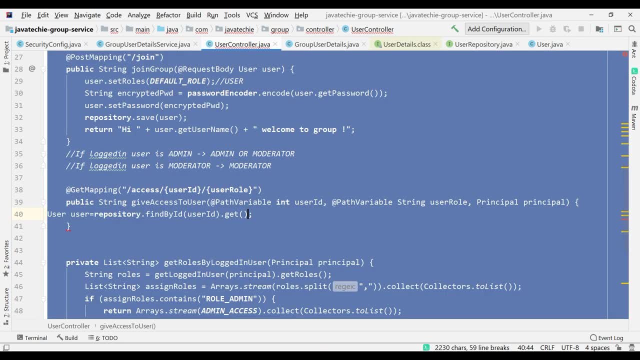 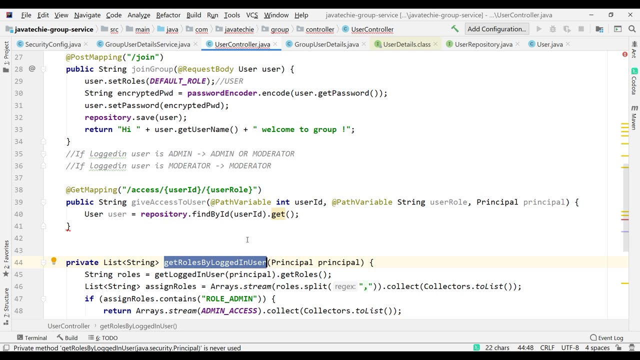 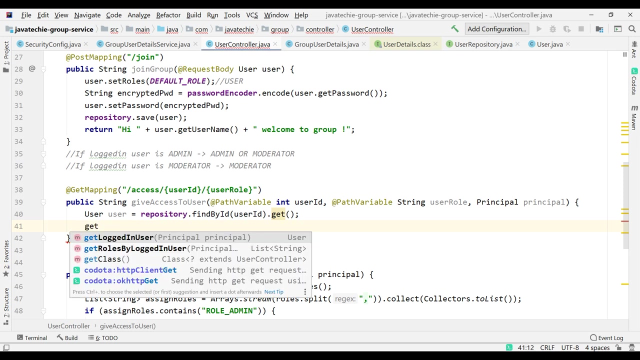 it will just give the user object: okay, this will dot get. this will also optional. fine, now just get the active roles. okay, based on the logged in user, which role he can provide, get those roles. so what I will do: get roles by logged in user. pass the principal object. 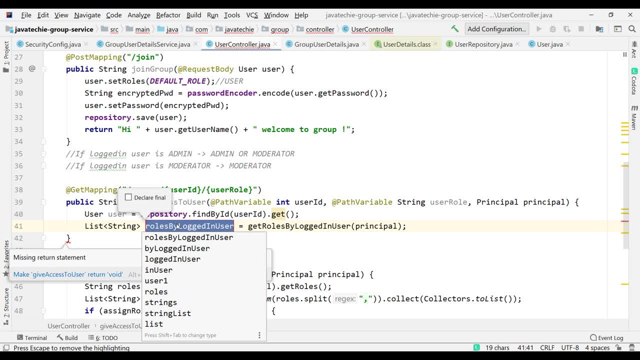 then define the local variable. I will name it active roles. okay, now simply just check the role which we are trying to assign: is part of this active roles or not? because this active roles will be the role which a logged in user can provide, right? so what I will do? 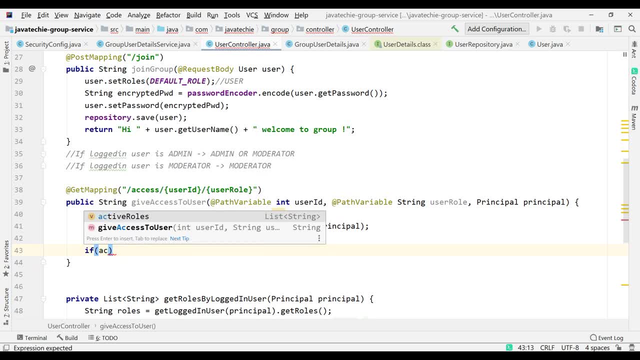 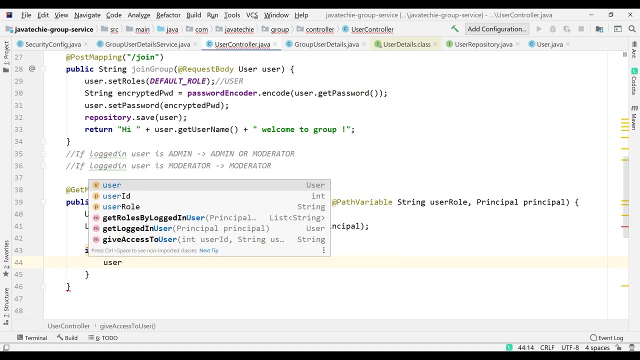 I will just write a if condition. if active roles dot contains role type, which will pass as part of input. now it is user role, user role. then just set that role to this user object. that's it. so what I will do. I will simply write user dot, get roles dot. so no need to get the roles, you just need to append. 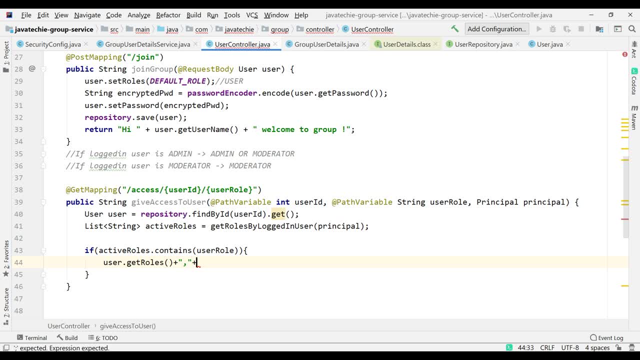 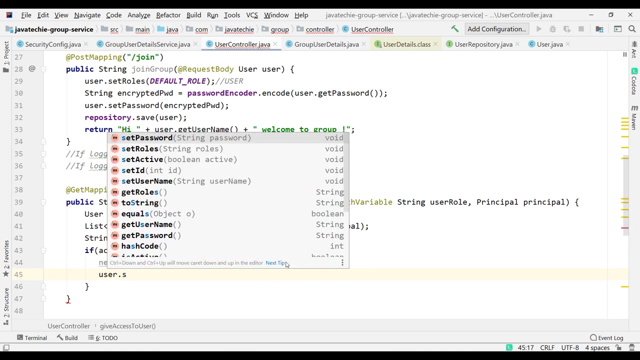 that role. okay, give the comma and append the new role. fine, so I will define a variable string- new role. so name it new role equal to this. then set this new rule to user object: user dot. set role- new role. this new role will contain the existing role of the user and the new role which we are. 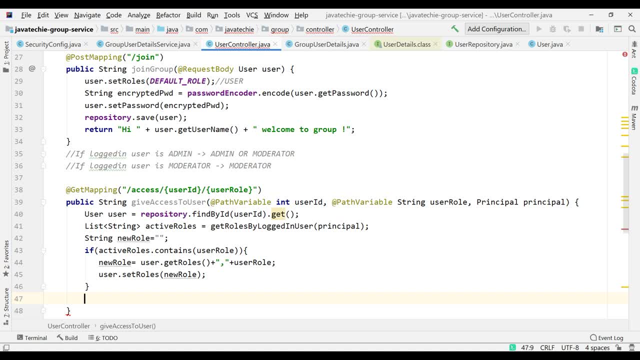 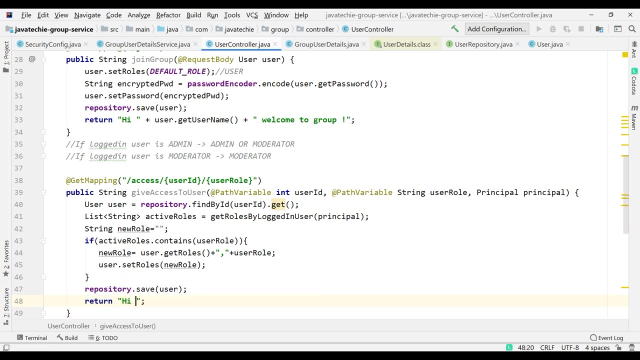 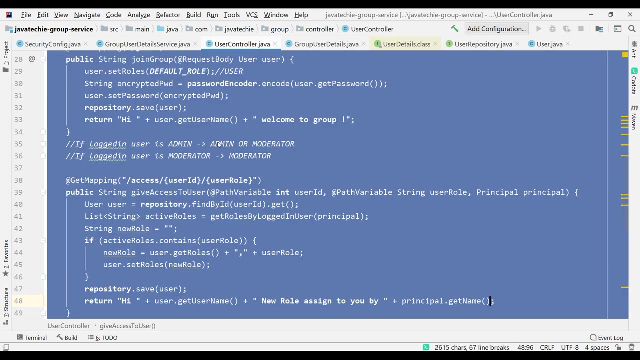 assigning to the user. okay, now what I will do. I will simply repository dot save user, that's it. and then we just need to return some message. hi, then give the user what is that user? dot get user. just inform that who give the access. okay, new role assigned to you by get the logged in user name: principal dot get name, that's it okay. 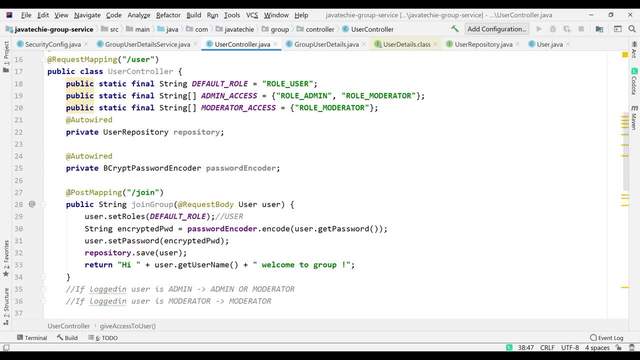 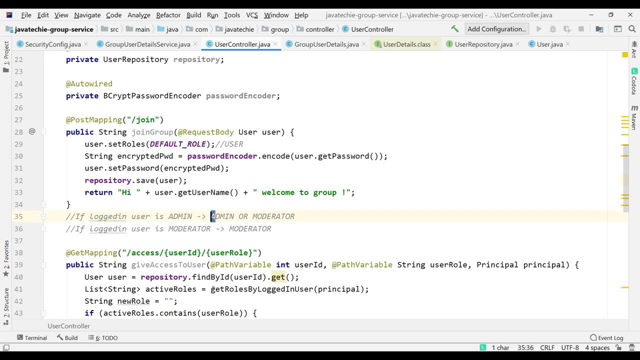 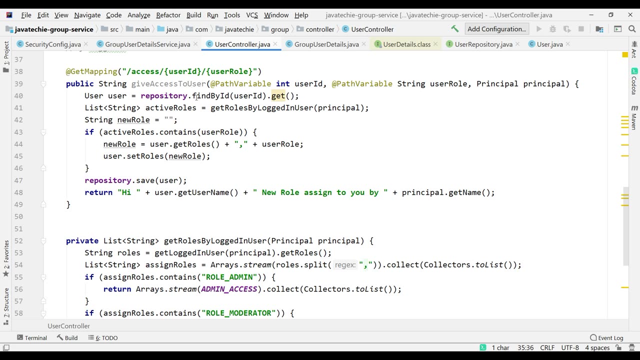 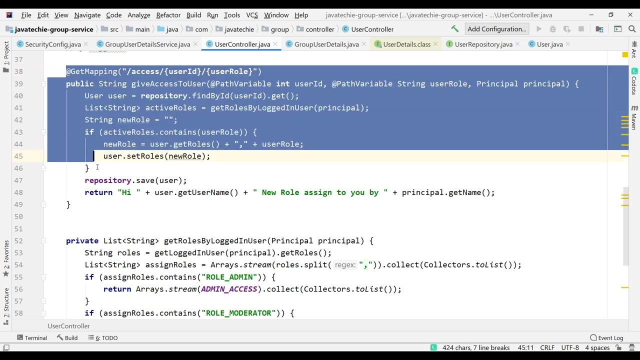 so now we wrote two API. the first API will add the user to the group, so for this we no need to add any authentication mechanism. but for this particular second API, where we are just giving the access to the existing user there, we just need to enable the role base authorization. I mean the moderator and admin can only access this API. user can't. 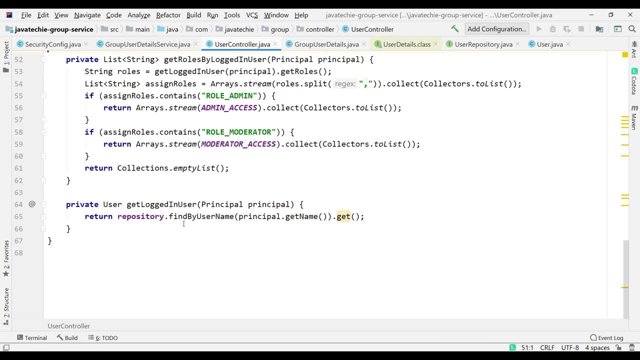 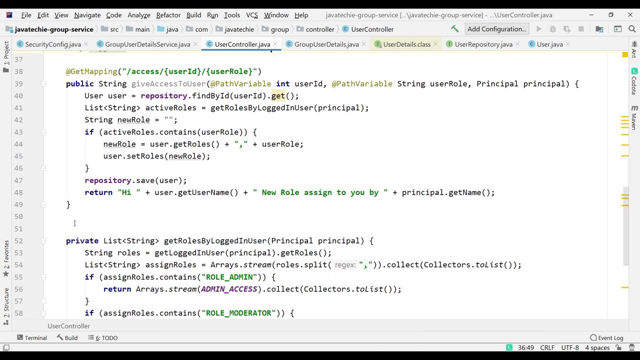 access this API. okay, so for understanding purpose, let me add two more end point. so I have the template. let me copy paste: software server browser blocks очно, so I'll just add here- that is just for testing purpose- one page, all the user from the repo and one. 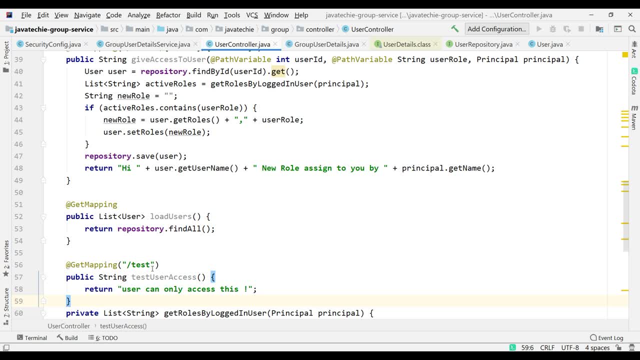 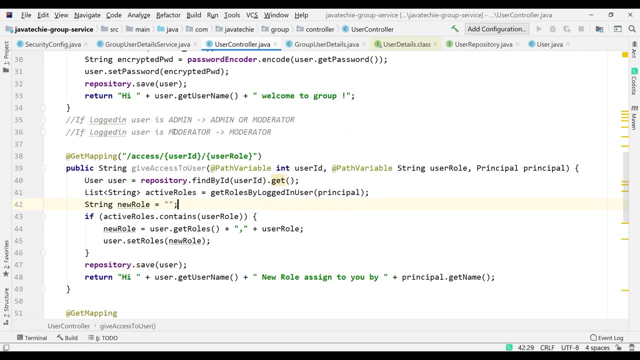 ornlly written because I just want to specify. I just want to demonstrate the authorization paues to our that's ok with this particular repeat and be only access by user. this particular API can be accessed by only admin or moderator. similarly, this second API also can be accessed by only admin and moderator, but 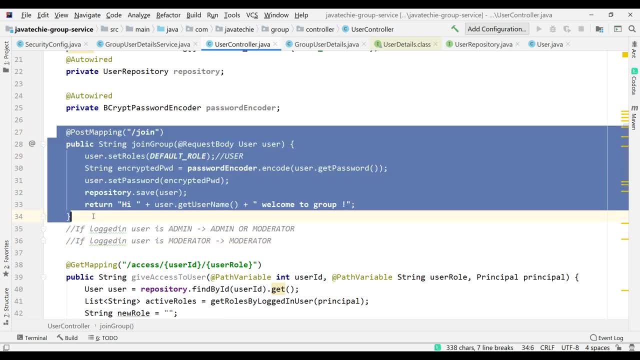 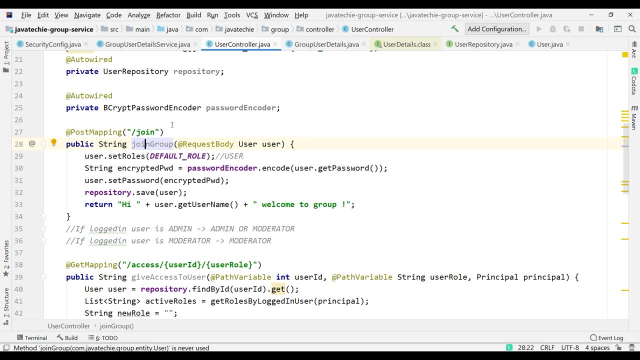 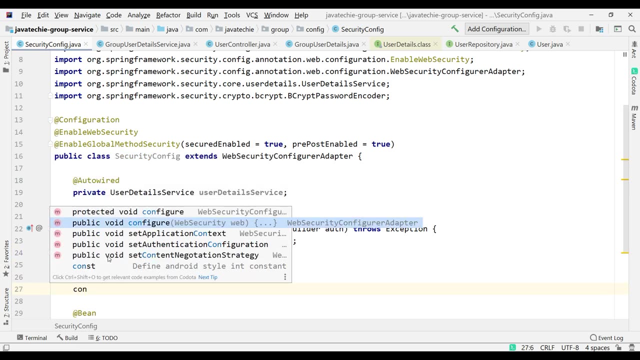 for this first API. there is no restriction. anyone can join the group, so we don't need to add any authentication for this particular method. so this authorization things we need to configure in our config file, right? so there is one more configure method, just override it, not this one, this one. so 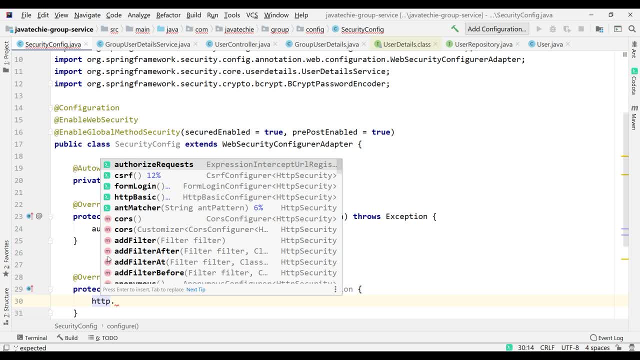 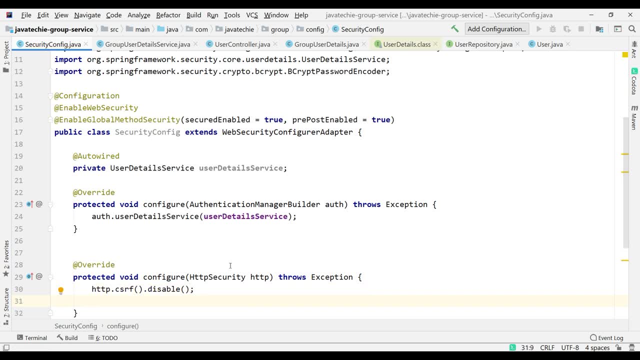 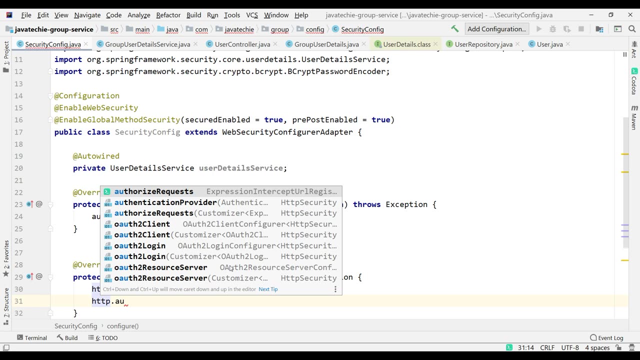 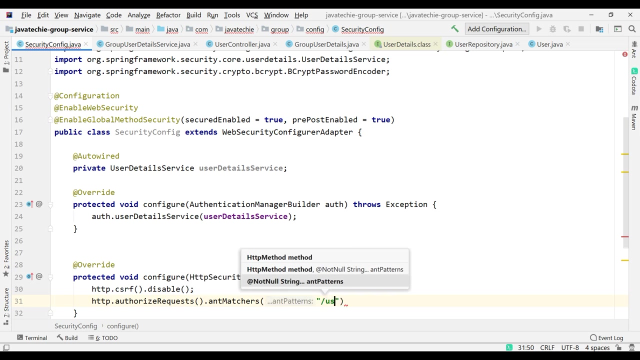 first we need to disable the CSRF. fine, then we just need to authorize all the requests based on the URL pattern. right? so HTTP authorize, request, dot aren't matchers. if URL is coming from you, slash user, slash, join, then permit all. there is no authentication required for. 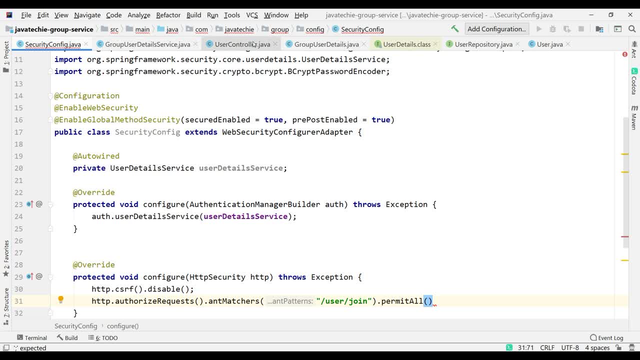 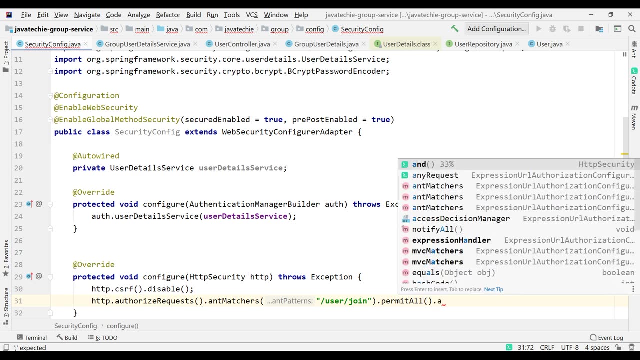 this particular endpoint. that's what I mention here. right, where is my controller, this guy? for this first method, I don't want to add any authentication or authorization. that's what I specify here. if request is coming from slash user, slash join, then permit all the request and authorize all the request. 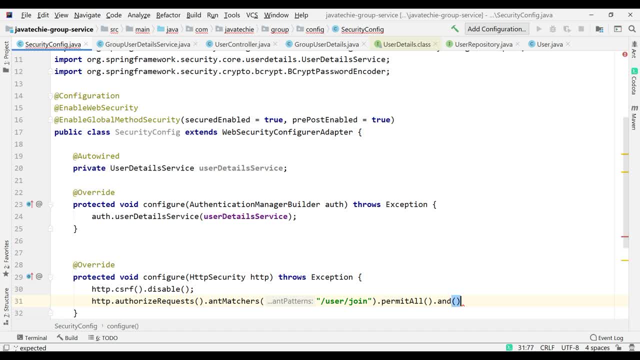 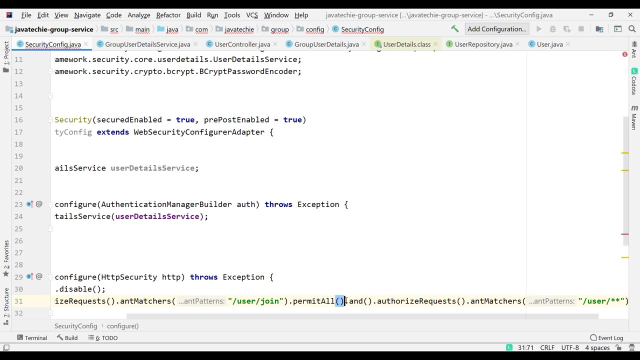 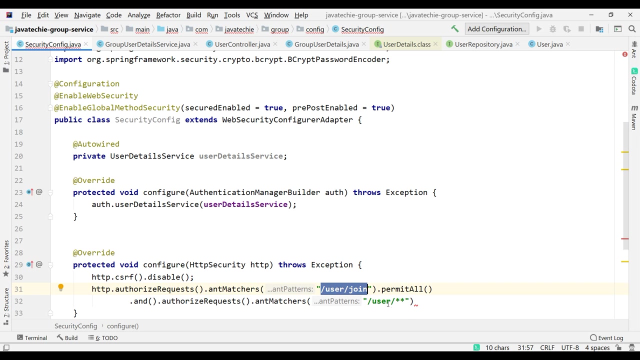 if the URL is coming from any other, just specify the aren't matches. so: slash user, slash star, star. so I will just split it, okay, so for this particular endpoint we are just disabling the security, but authorize all the request. if the request is coming from slash user, slash tester. for any other endpoint, just. 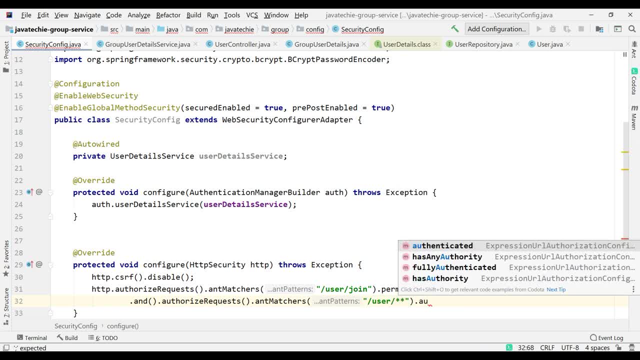 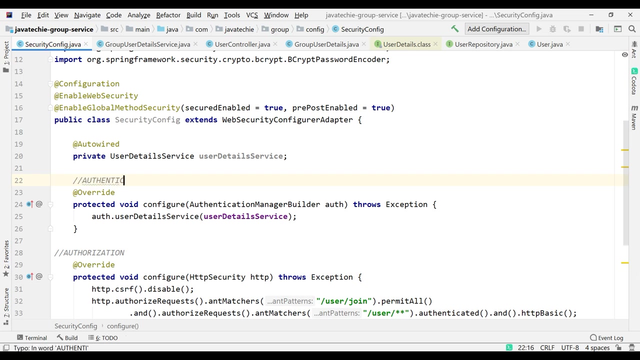 authenticate it. okay. authenticated dot H03. basically long, so hope this makes sense. one URL pattern to disable the security. one URL pattern to enable the security. I mean this particular method is for authorization. so let me specify here: authorize some, this particular method used for authentication. okay, so this is how spring. 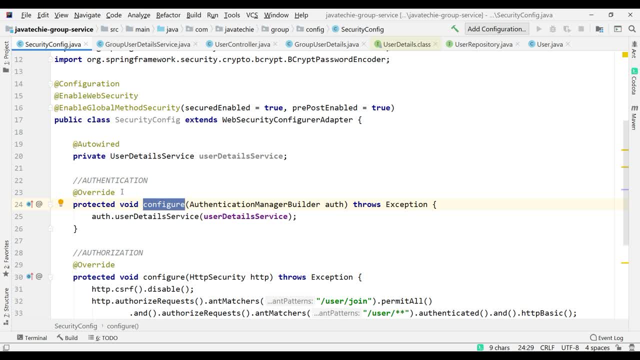 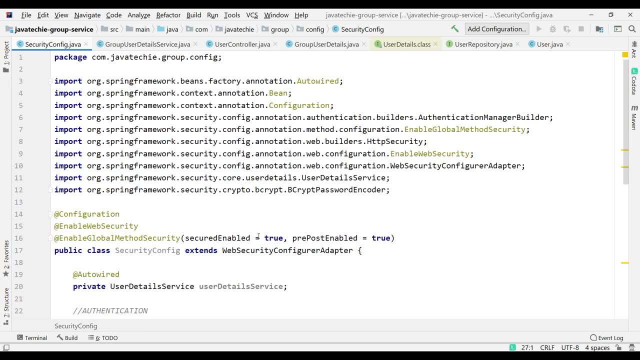 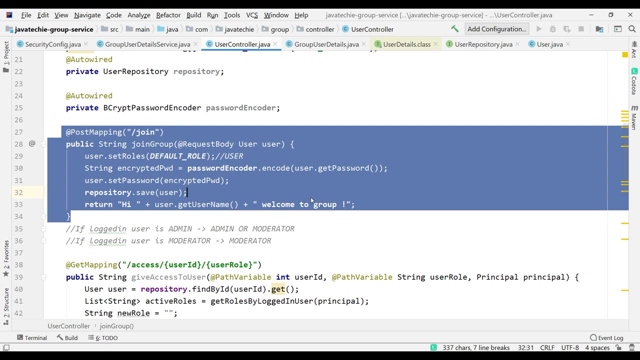 security actually work. there is overloaded configure method. you need to understand what used for authentication and what used for authorization. now I guess we are good, but we just need to enable the authority to access the API. so what I will do? I will just for this. you don't need anything but for this. we 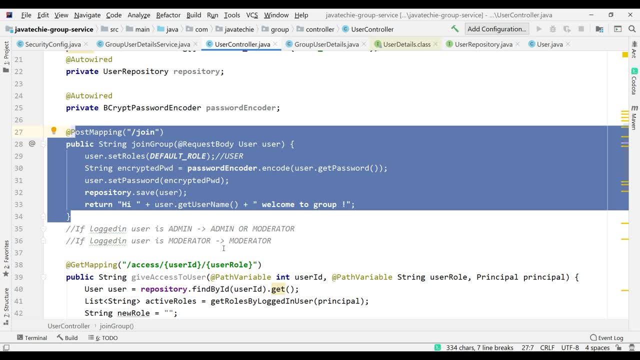 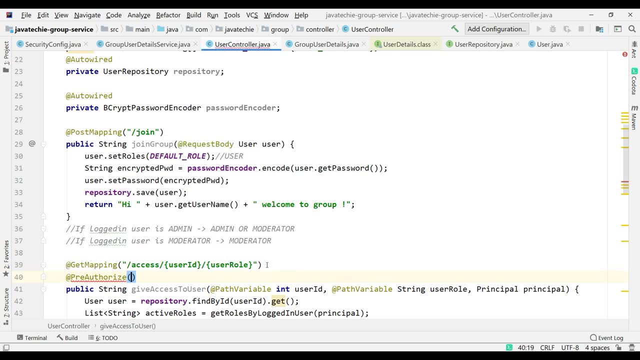 just need to validate whether the user who is trying to access having the admin or moderator access or not. so what I will do, I will just- there is something called pre authorized. okay, then specify: has authority role admin or has authority role moderator, if the logged-in user has authority role admin, 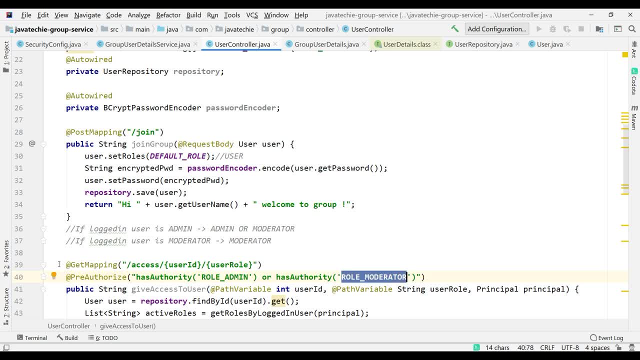 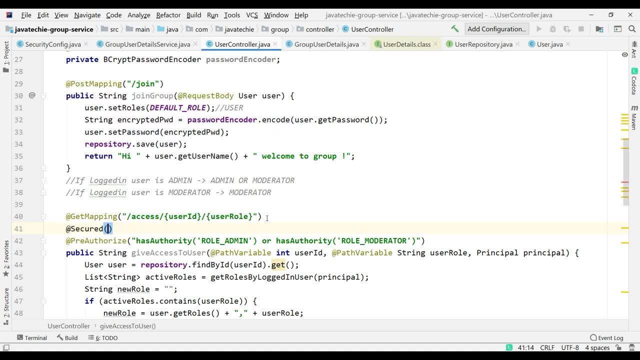 or has authority- role model moderator- then only he can able to access this endpoint. okay. also, if you want to specify, you can specify secure role admin or role moderator, like that. okay, but the purpose of these two annotation is different. so for this example, we need this pre-authorized. but if you want to, 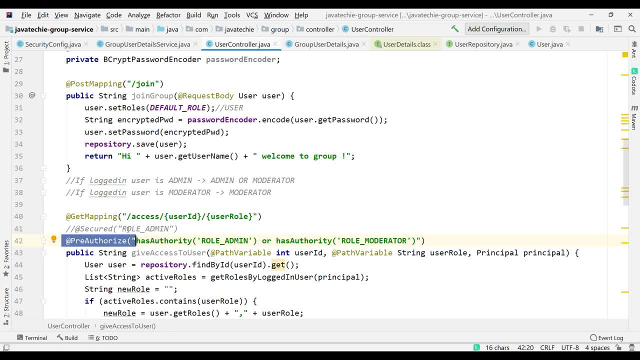 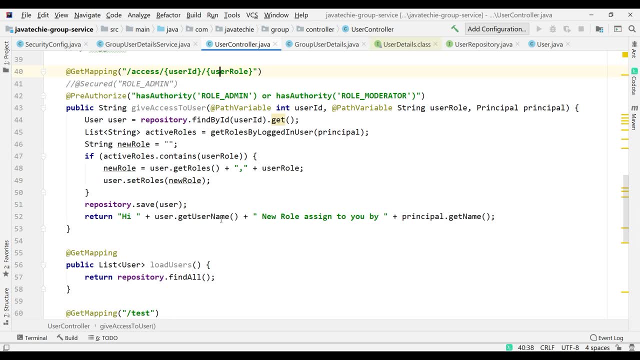 validate based on the api. based on has role: you can go for this. secure also has role. you can go for this. pre-authorized also okay. so now let let's add for other api. so let me copy this, so this i want can be accessed by only admin. so i will remove this. 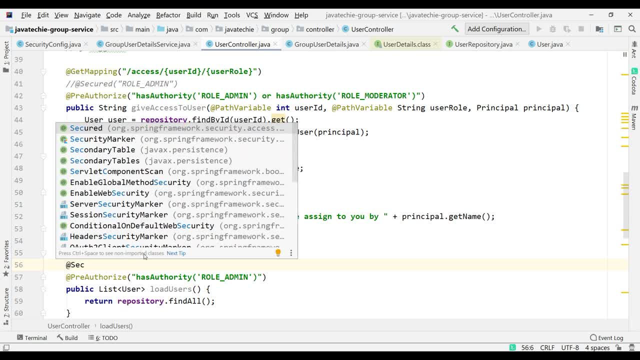 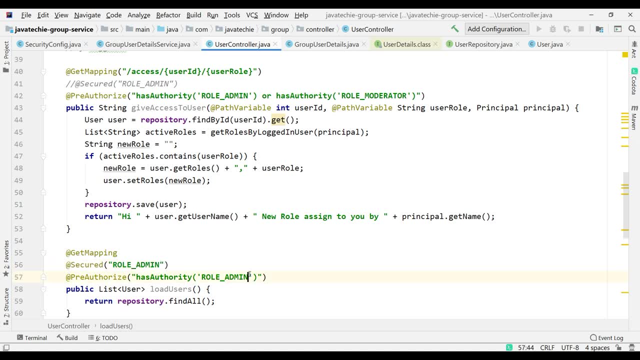 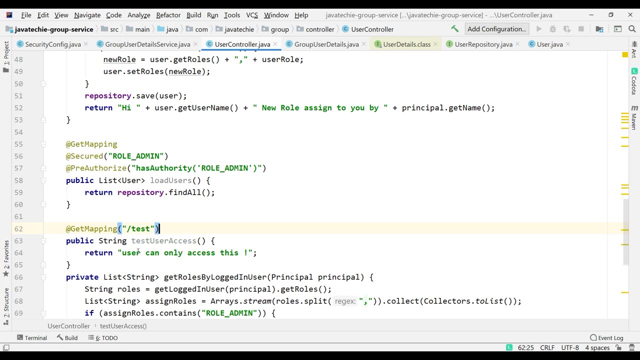 okay, so for demo purpose, let me add this secured also. even you will not add this secured, it will work. now the last api can be accessed by only user. admin can't access this user information, so i just return a string. we just need to add some real-time scenario means real-time world, example. 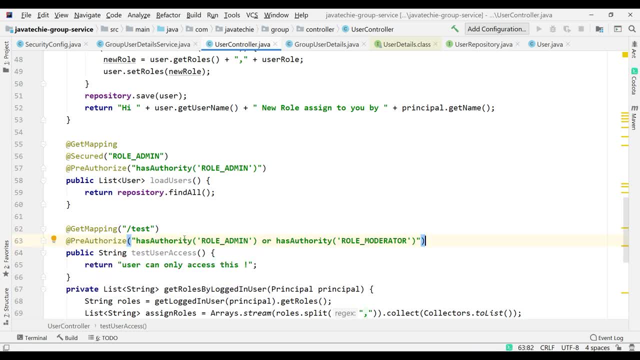 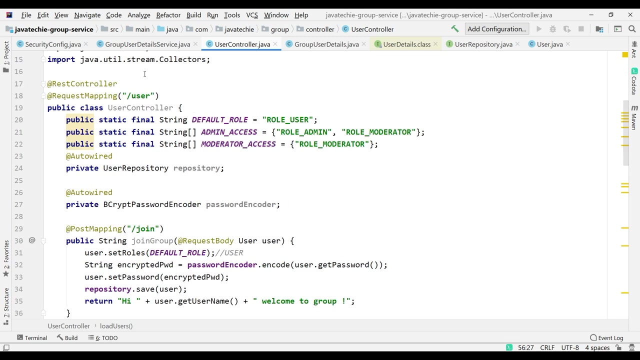 here, so i'll just copy paste this. this can be accessed by only user. fine, so there is no url for this. i can directly access using user slash, user, right? so i guess we are good. now let's start our application, but before that let's follow the coding practice. 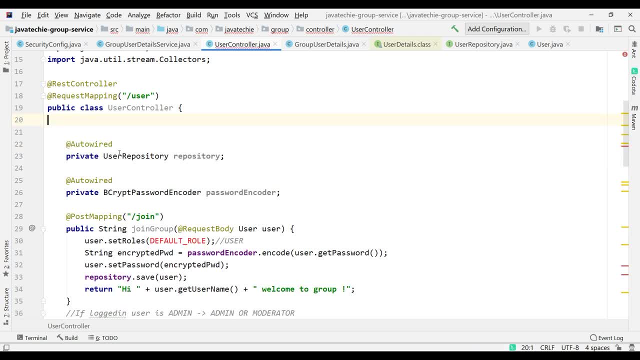 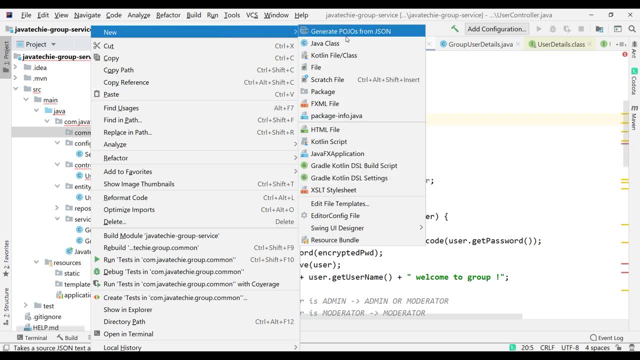 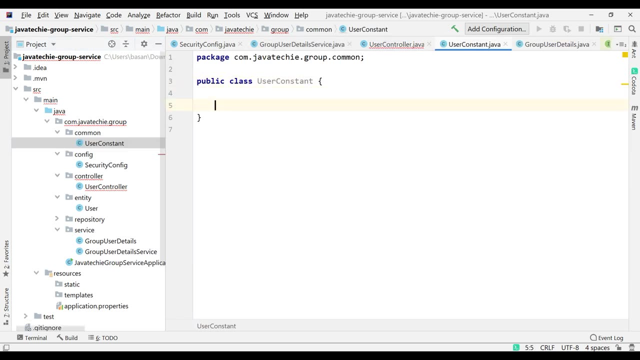 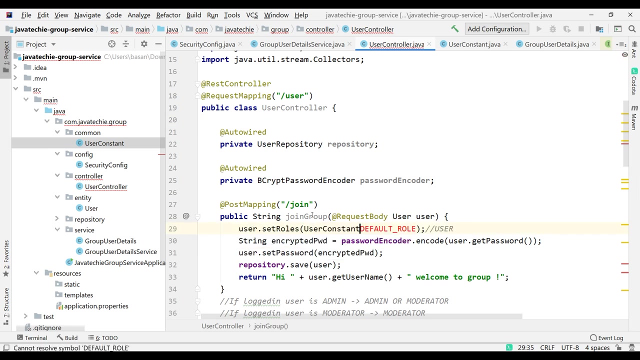 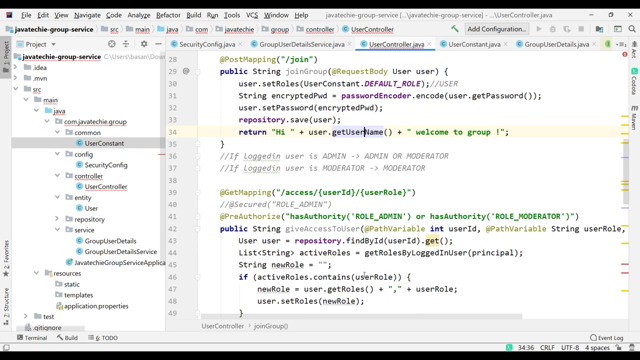 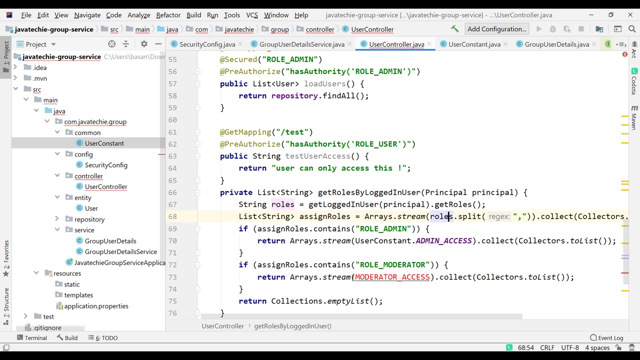 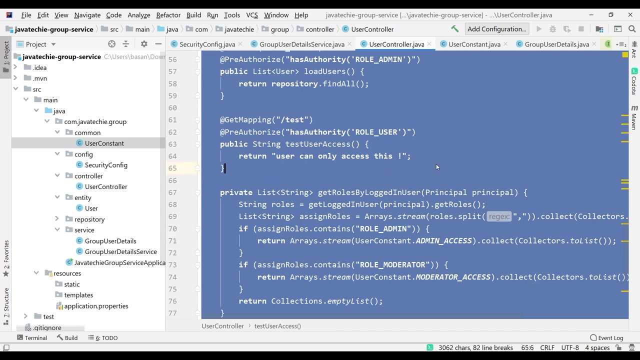 will not add this here. go to the project. already i created a folder called common, so just add it here. user constant. fine, now let me copy this class name in controller. i can directly use this. fine, now let's run our application first we'll add couple of user. 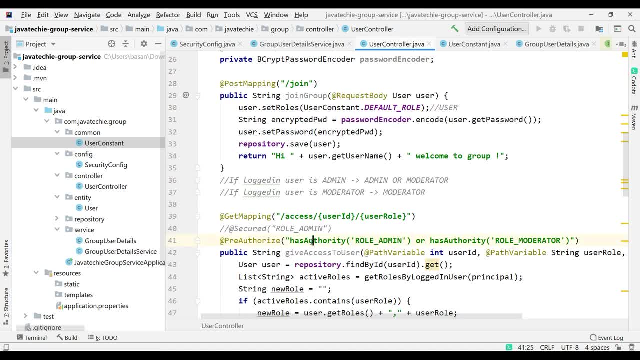 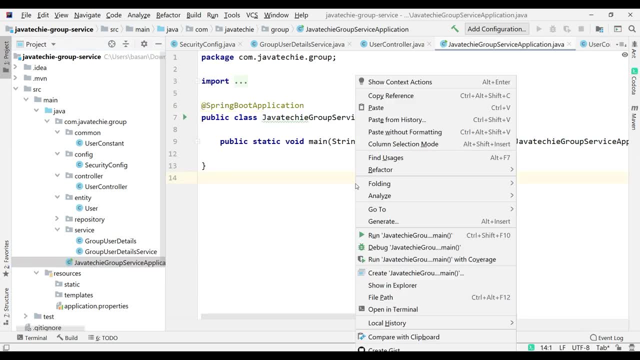 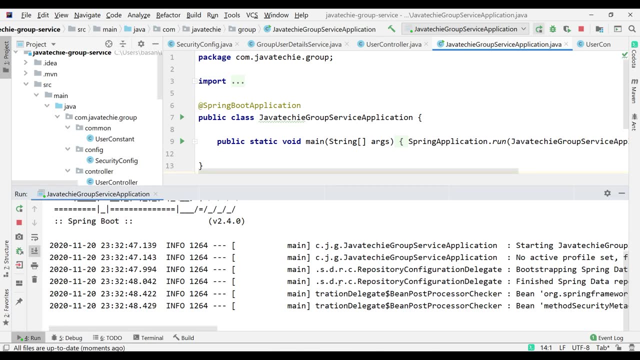 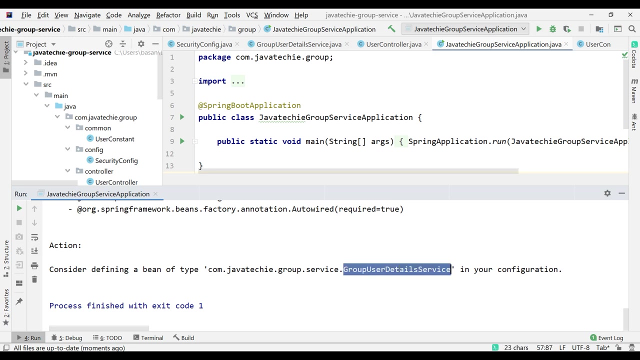 then we'll go for the other api testing based on the authority. okay, yeah, so let me start my application. go to the main class run as java application. so let's wait it to complete. there is some compilation error. comjavatk. this class is not found. it need auto add. 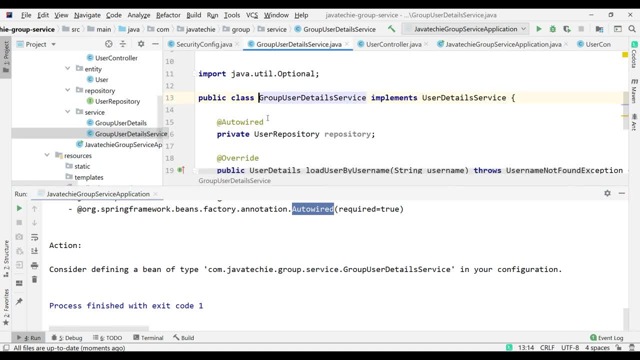 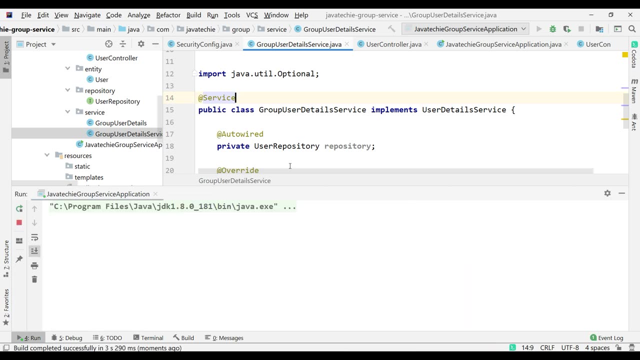 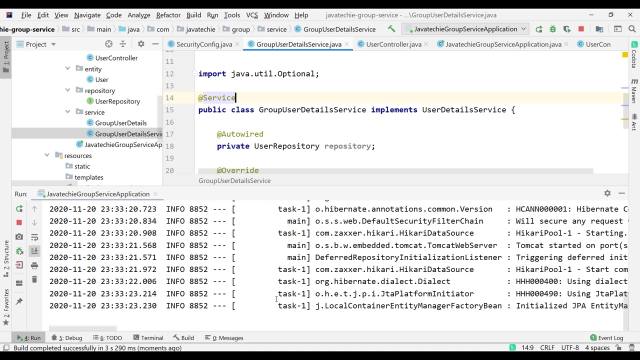 so go to this class. okay, so we need to annotate here at the rate service. that's why spring is not able to scan this bin right now. save this and let's restart it. yeah, let's starting now. so, if you observe, our application is up and running now let's try to. 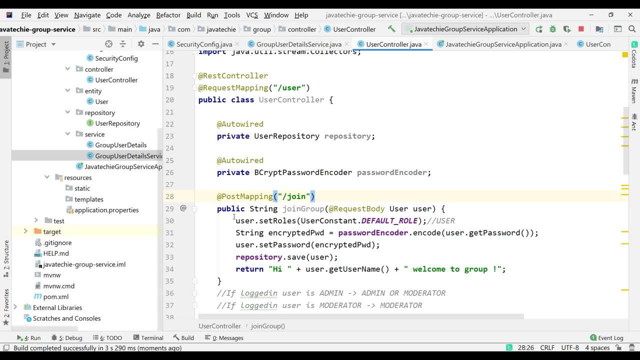 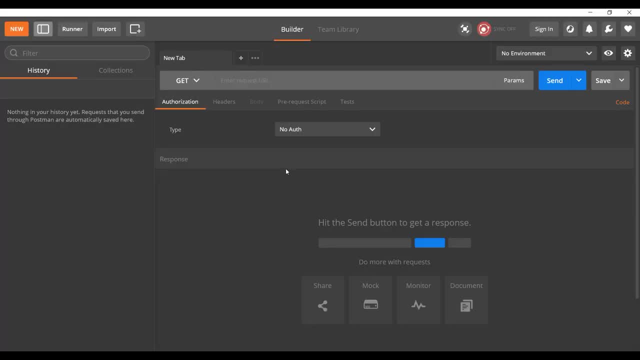 access the endpoint, so the first endpoint. we just need to add the user to this group, right? so for this we disable the spring security. so go to the postman. method type is post type: http: localhost 9090. user join body raw. then change the media type and give the request. so username password. 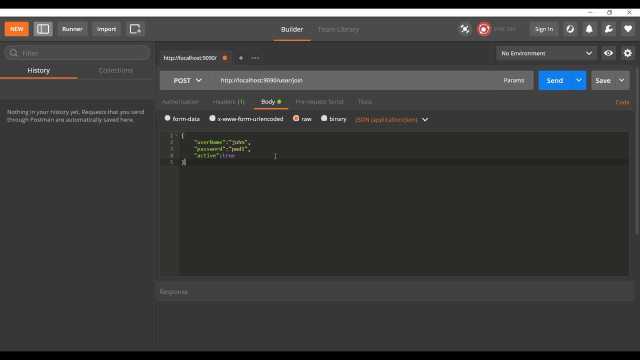 and active user id will be auto generated and role by default. we are setting as a user right now. click on send one record inserted. now let me add couple of record. so i will add smith. change the password to pwd2. then i will add basant. i will change the password to three. 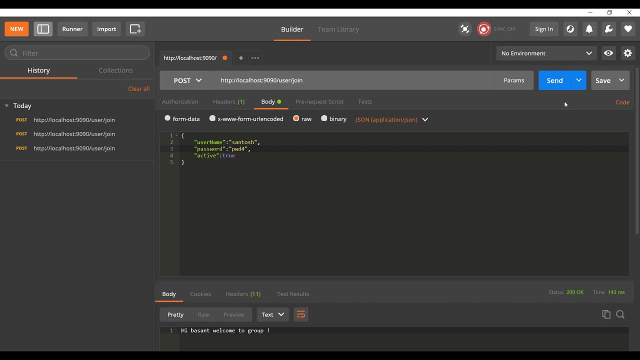 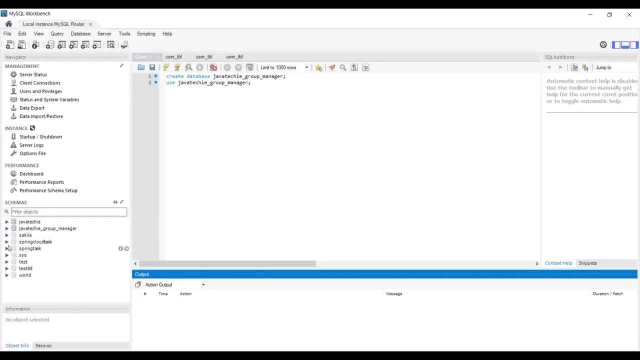 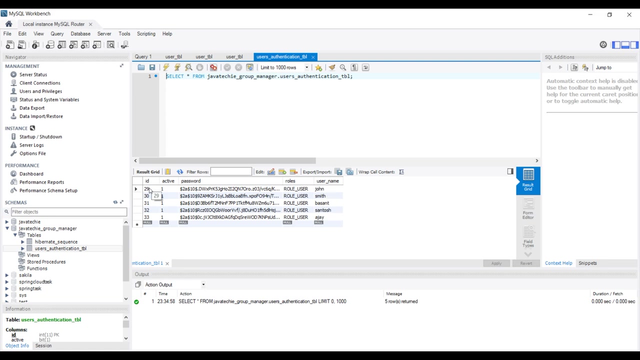 santosh. then i will add azure password five. okay, so i added five user object. now let's verify the same in our database. so just refresh it. go to this. i change the table name to the user authentication table. okay, so you can see here we added the five user object and the id is started from 29 and i don't. 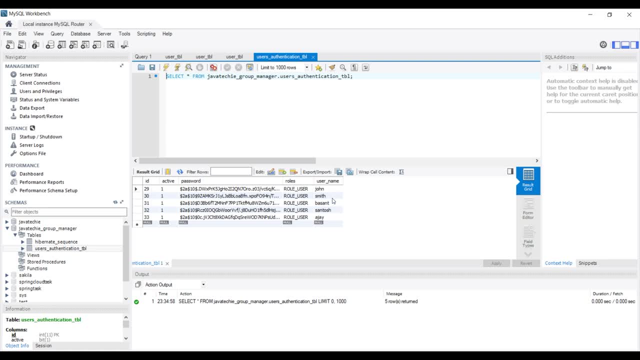 know why it's behaving like this. okay, so our intention to check with the username and password. let it be so by default, all the user having the role user. so i need to make someone as a admin so that we can perform all the operation right. so what i will do? i will just write a update query. 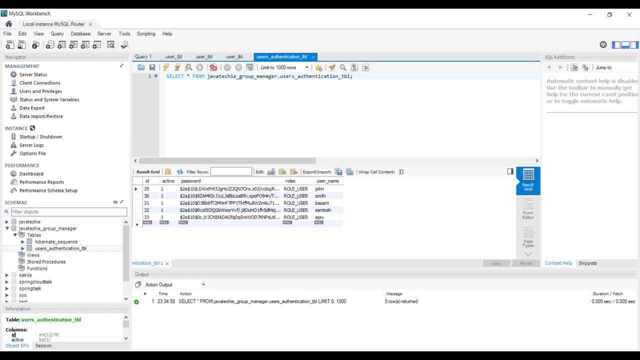 so just write update, then table name: set the field roles equal to. i just want to give the admin role right, so i will specify role underscore admin, then give the where condition where id equal to. so i just want to make this guy as a admin okay. 31. 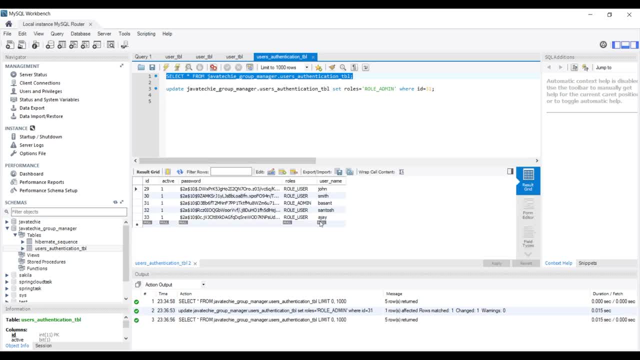 now just select the table. fine, so if you observe, the role has changed to role admin, so this guy having the role admin. now as a admin, i just want to give moderator access to some of the user. that's what our second api right. if that api will tried by any user then he won't be able to. 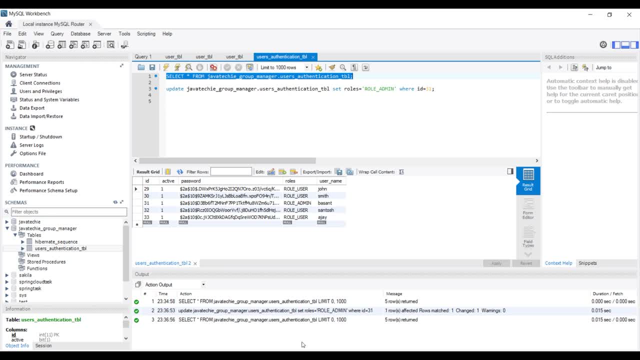 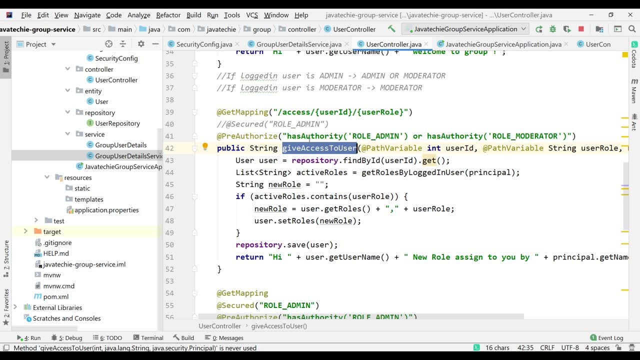 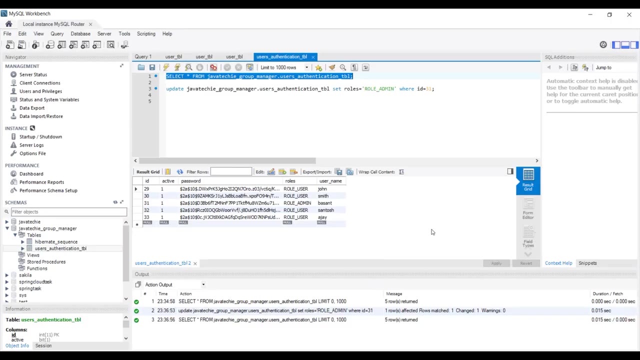 that api can be accessed only using admin or moderator. so let's go to the endpoint. if you observe here, this particular, give access to user. api can be accessed by who is having the authority- role admin or role moderator. right, as this guy is admin, so i can give moderator. 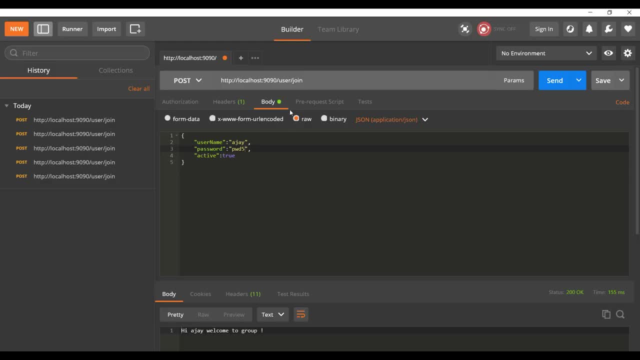 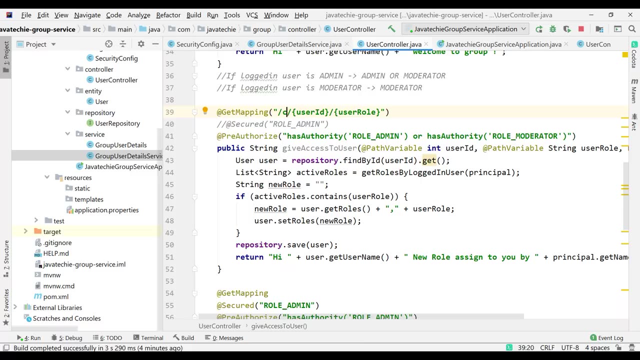 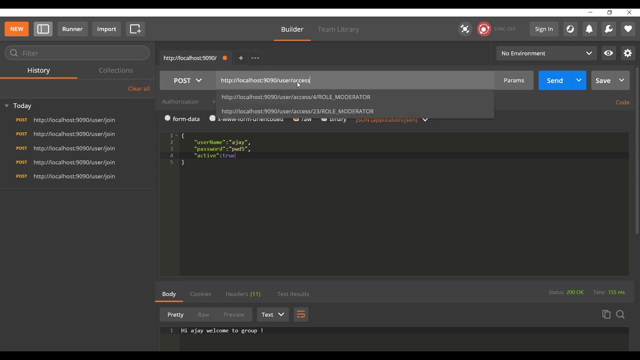 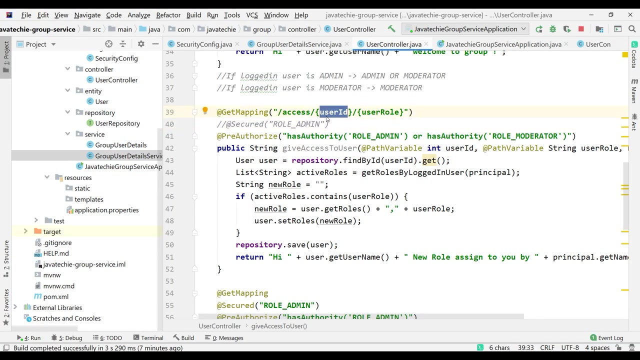 access to some of the user. so let's try that. let me copy the endpoint access and paste it here. okay, then, what we need to pass. so if you observe here access, then pass the user id to whom you want to give the permission. then pass the user role, what permission you want to give, right? so if you 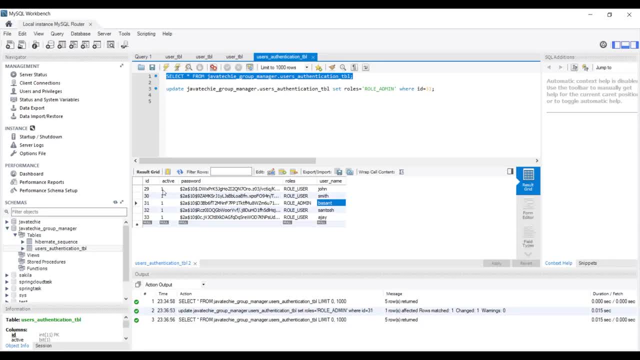 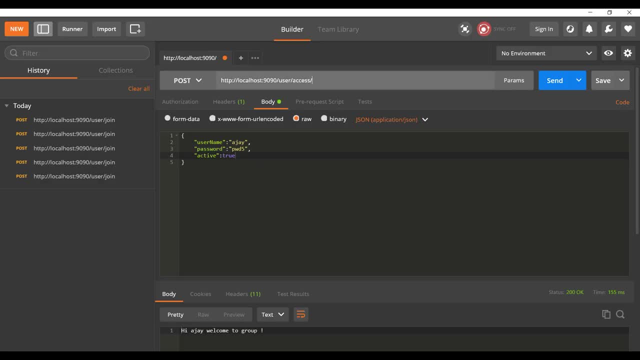 will go to the db. so for this first user, i just want to make him moderator. okay, so i will give the id as 29 go to the postman and i want to give him a role- moderator, okay, fine, now this is the gate api. just change it and you need to pass the authentication. 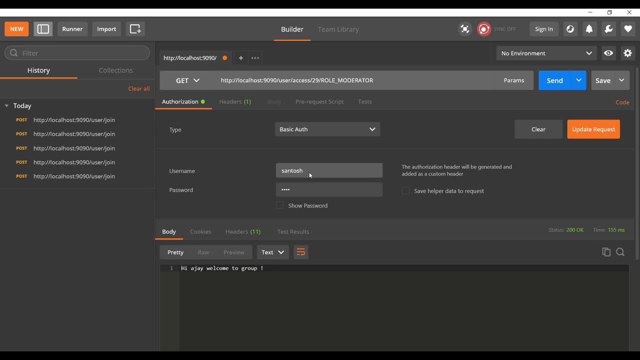 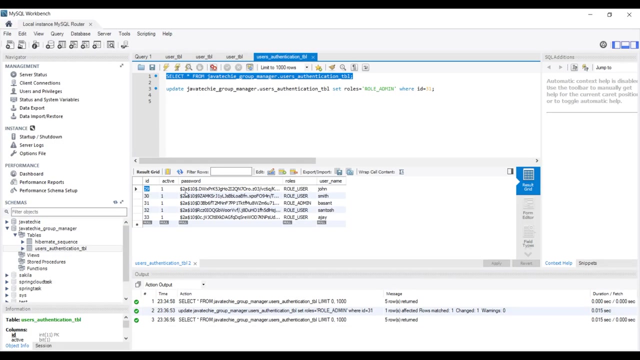 right, that is the basic auth, so click on this basic auth. now you need to pass the username and password so this api can be accessed by only admin and moderator. so let's try to access this using any of the user, then we will see how we are getting the error. so let me try this guy. 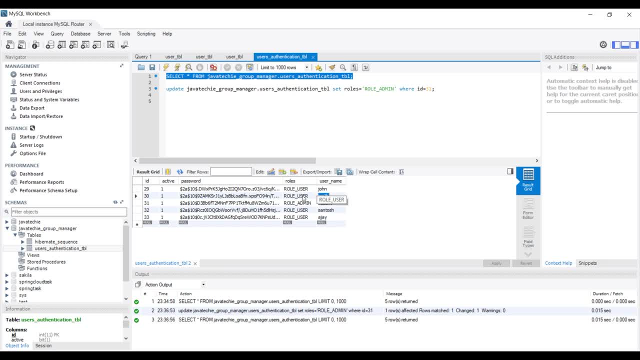 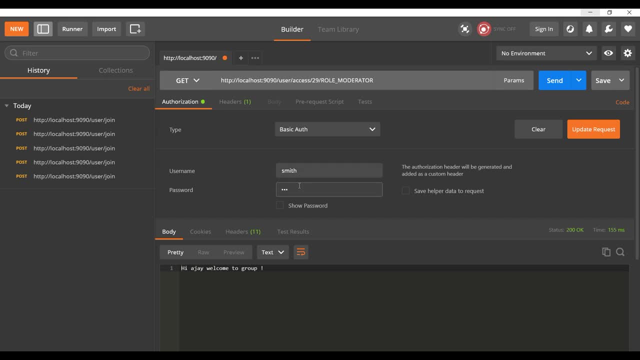 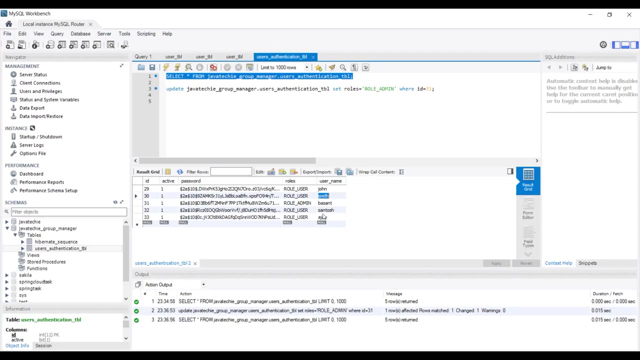 okay, smith, because if you observe the role is user and the password of smith is pwd2, right, update the request and click on send. so if you observe we are getting 403, which is forbidden, it means that particular user don't have access to this api. okay, so now who can access this? the guy who is having admin access. currently we have. 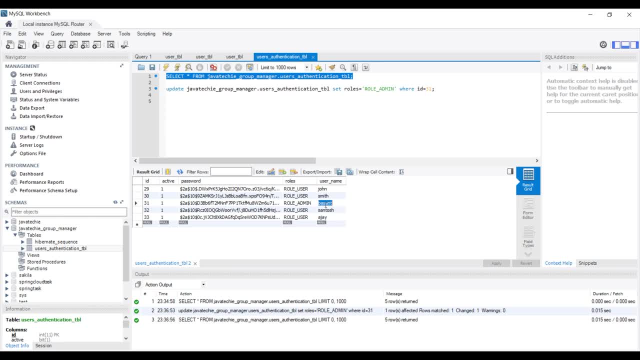 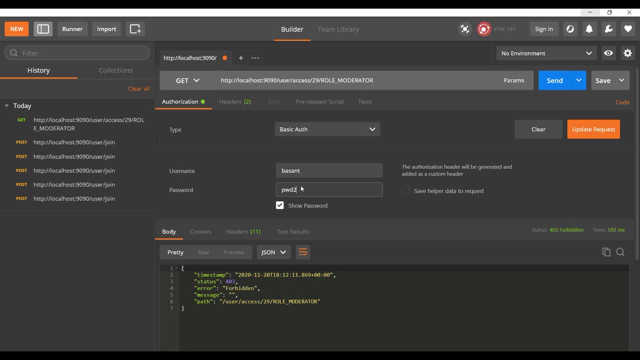 only one user who have the admin access. so let's pass that credential, then password 3: update the request, send it. so now you can see here, right, hi, john, new role assigned to you by basant. this is what the string message we are returning from our controller, isn't it? so now, if you will go, 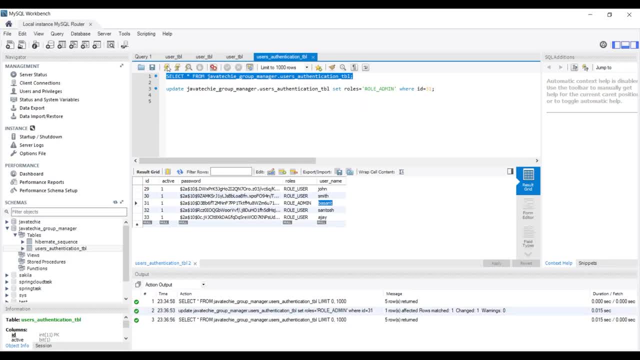 and verify in your database. if you observe john have two access. by default the role is user and second we just assign to moderator. now if john will try to give access to someone, he can give only moderator access. he can't give admin access. so let's try that. 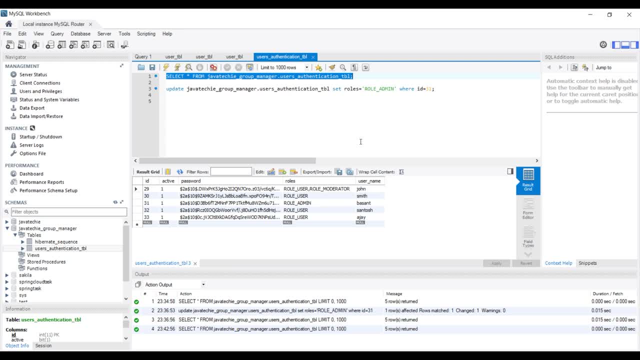 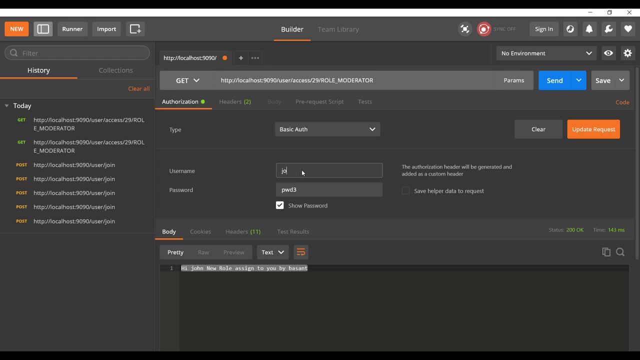 so let's login by john and we want to give to this guy 33, okay, john, pwd1, and he can only give the role moderator. if i'll give role admin, it won't work to the user. what is the user? 31, right? 33? okay, hi, aj, new role assigned to you by john. if you will go and check in your db. 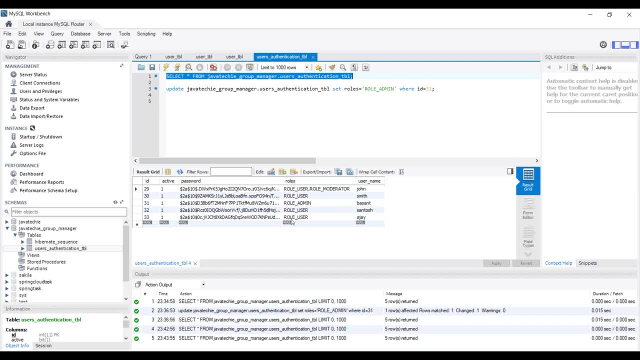 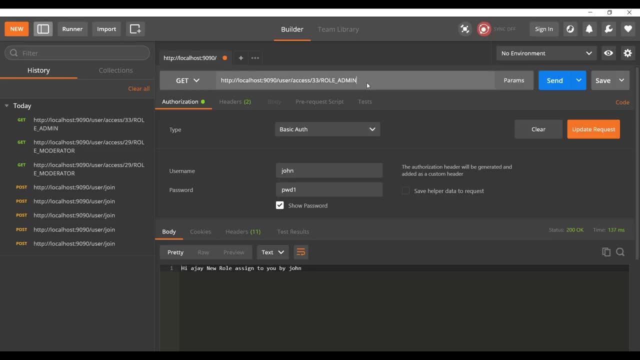 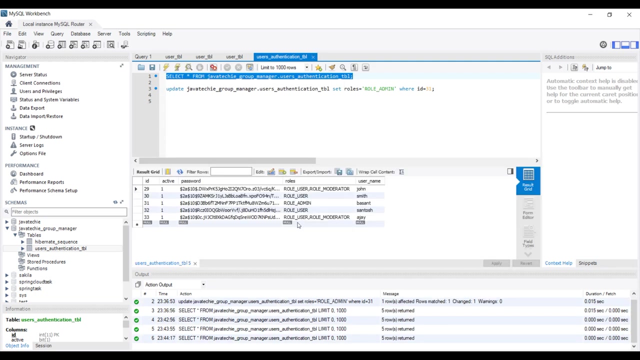 to this guy. there is no change right, because he can't give the admin access. but if he he will try the moderator access he can give it because this guy is moderator only right now. if you verify in your database you can see here. right, it got changed to moderator. now i can. 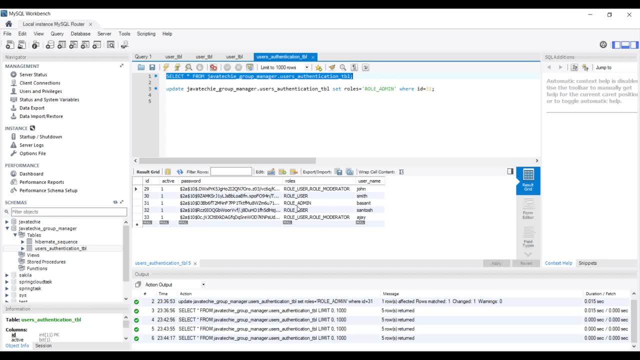 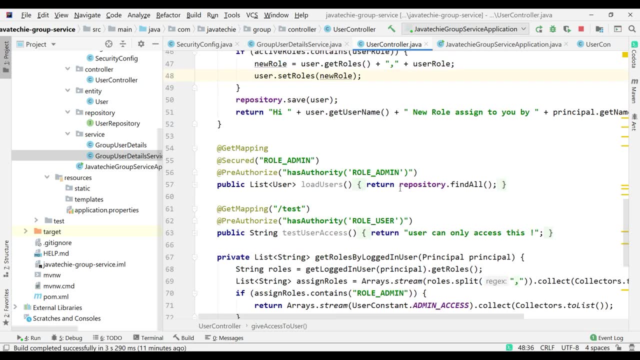 give the admin access if i log in through this basant. okay, so this api is working as expected. now go to the third api, so this particular load user. it will return list of user from our db. this can be accessed by only admin. okay, so let's verify in db who have. 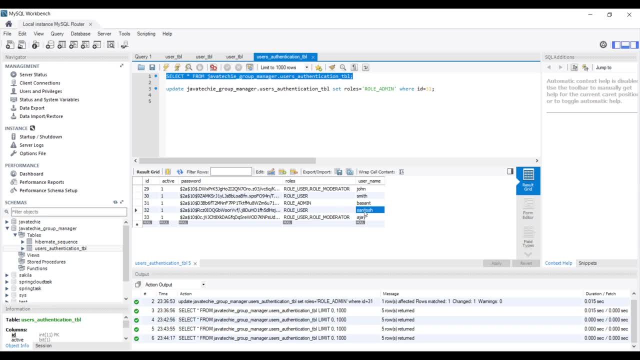 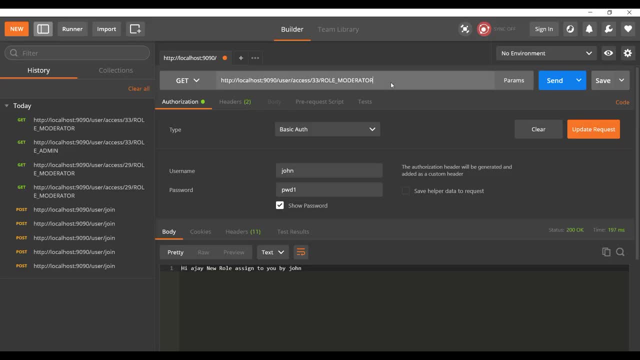 full user access. uh, santosh, he is a user. let's try to access that by a user. okay, user. so let's give the santosh and password is: password is four right pwd4. update the request. you will get 403 because the role of this particular santosh is user and this api, particular api, can be accessed. 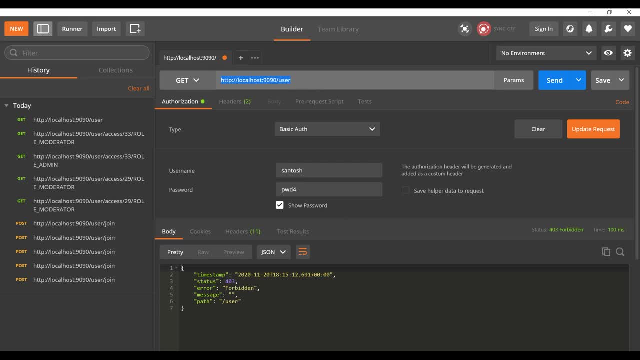 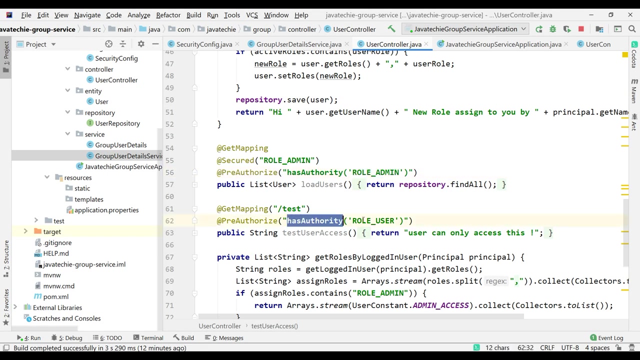 by only admin. even moderator can't also access this, so let's try with the moderator. okay, so who is having moderator? john john, and password is one. update the request, send it. you are getting 403 because we specify this can be accessed by the person who is having the authority. sorry, this one who is 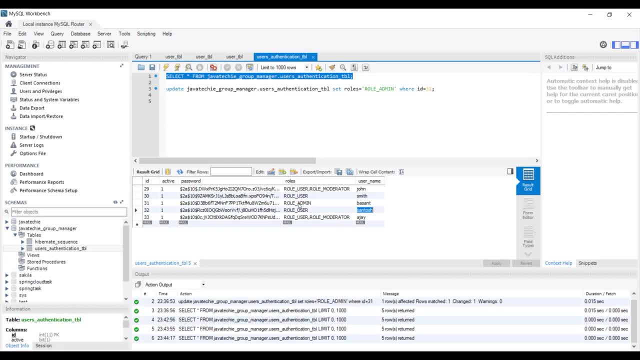 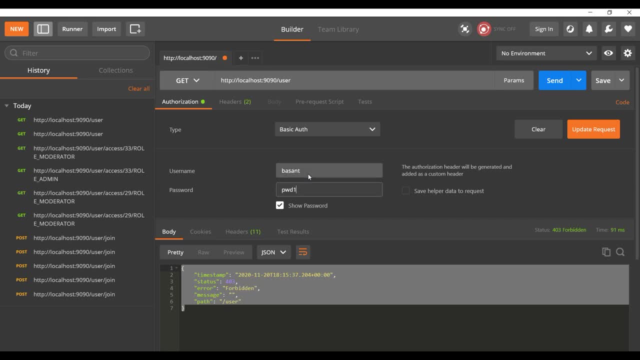 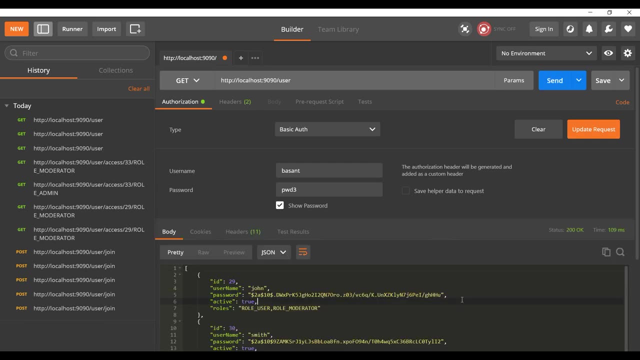 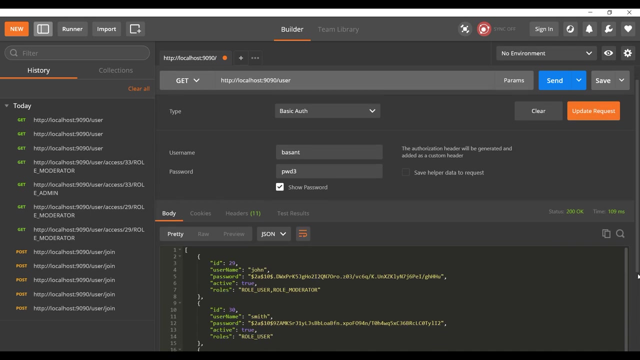 having the authority admin. okay, now let's try access using admin. go to the postman who is the admin. give it Vasant PWD 3, update the request, send it. we can see all the user here, right, let me drag this up. okay, we can see all the user. 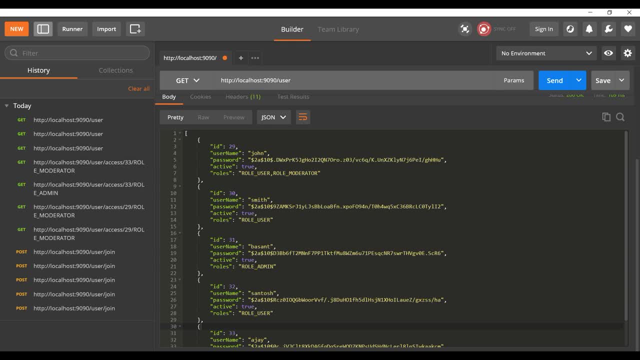 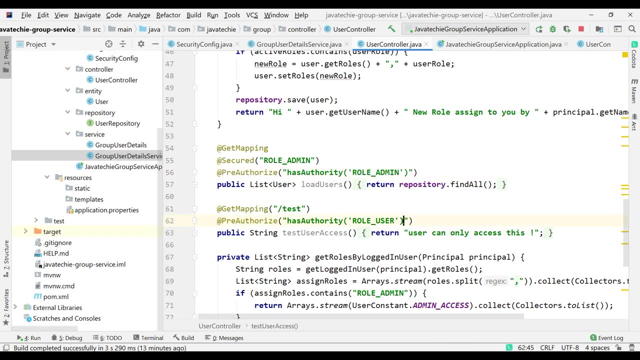 here. now let's go to the next EP. yeah, so if you observe, the next EP can only accessed by the user. if admin or moderator will try to access this, you don't work. okay, you can see all the users here. right, let me drag this up. okay, we can see all the 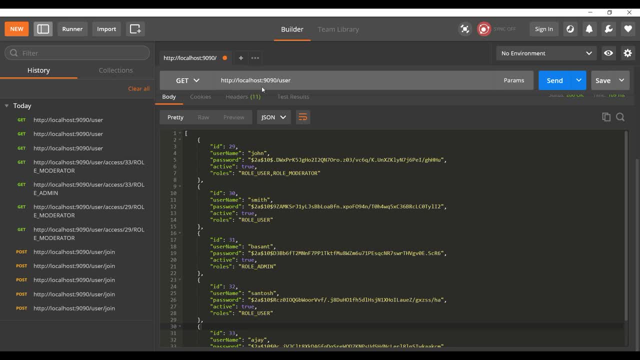 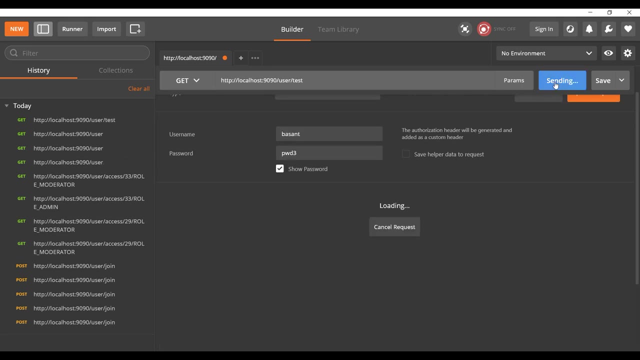 so let's try accessing by admin user slash test. so already i logged in by admin, right? so why it's not going down? yeah, this is the admin. now if i try to access it, i will get 403, because this particular api can be accessed by only user. 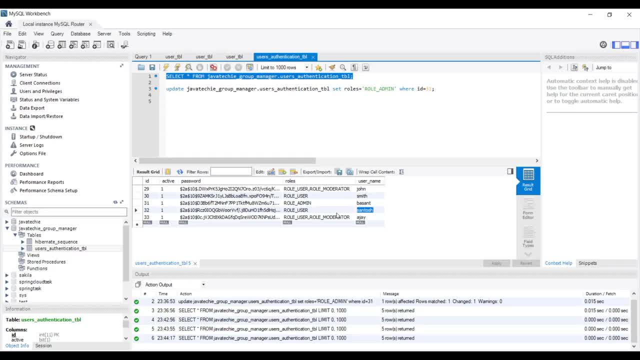 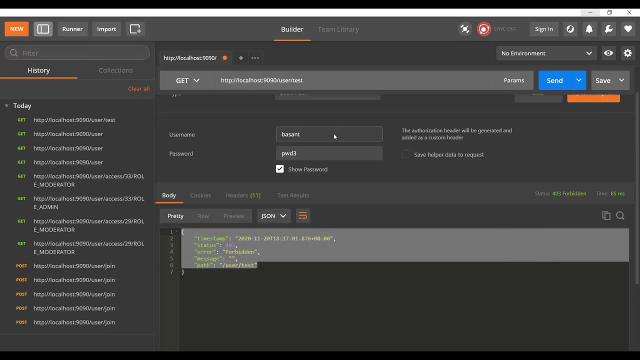 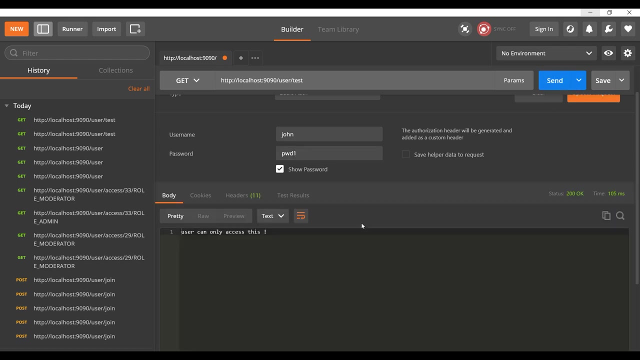 so who is the user? let me verify db. smith john, everyone is user apart from this basant. okay, because this john have role user and moderator access. he can also able to access this because he have user access. so let's try this. update the request, send it. he can able to access. 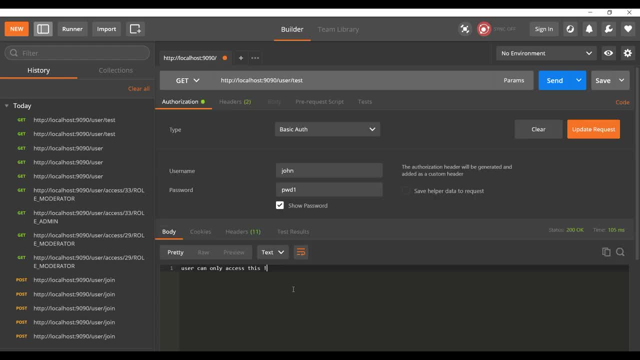 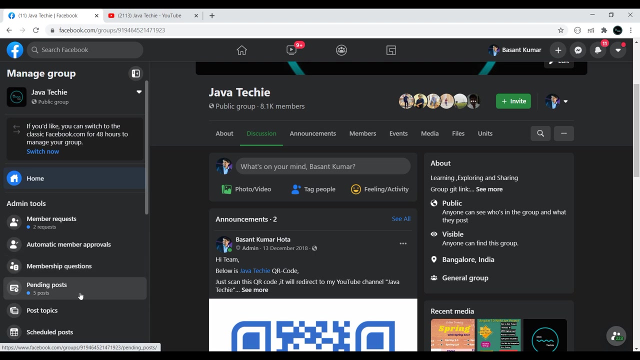 right user can only access this, so so. so this is how we can implement role-based authorization in any of our real-time application. so in my next tutorial i will cover one more feature. if you go to the facebook group, there is a option called pending post. if i am a admin or i am a moderator, i can see this option. 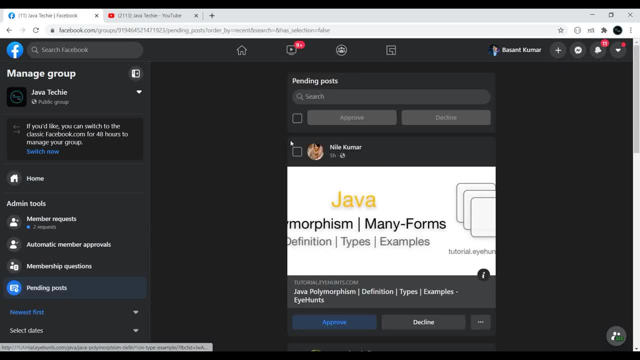 okay, so if i will click on this pending post, as i am a admin, i can do the bulk approval. if i will tick mark and if i will click on this approve, all the pending post will be approved. similarly, if i click on decline, all the pending post will be rejected. 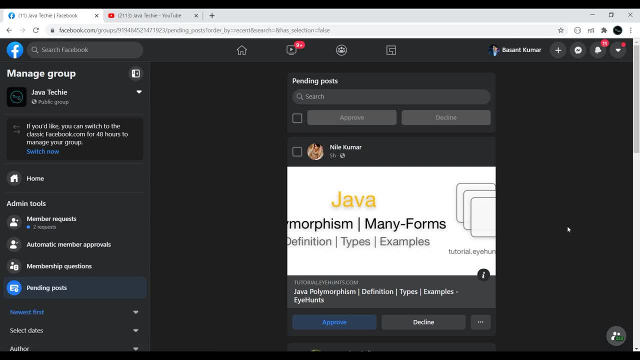 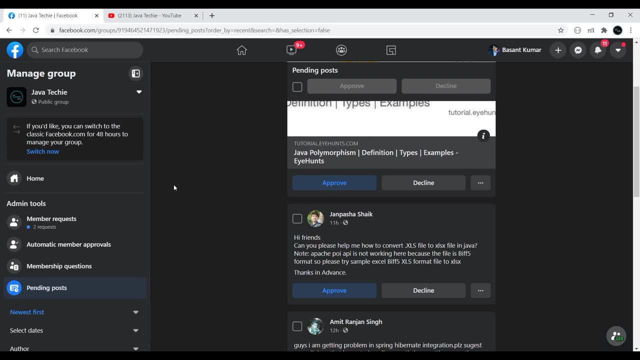 if i want to do individually, i can do that. click on approve- it will approve the post. click on decline: it will decline the post. okay, so let me know in comment section if you are interested to see this kind of scenario using spring security so that i can prepare the content on same okay. 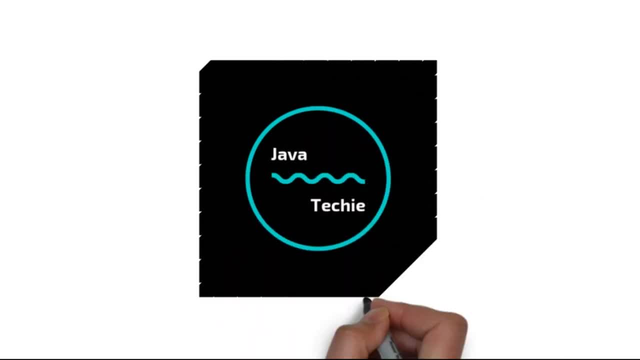 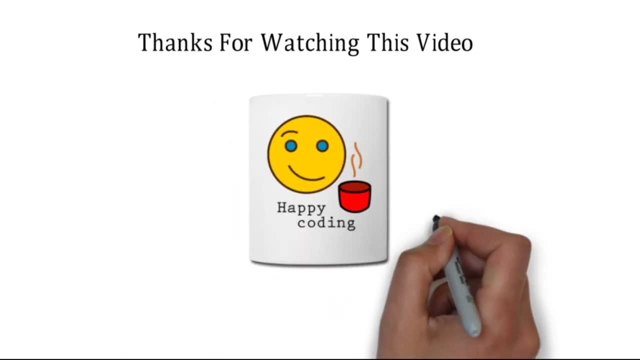 that's all about this particular video. guys, thanks for watching this video. meet you soon with a new concept. you. 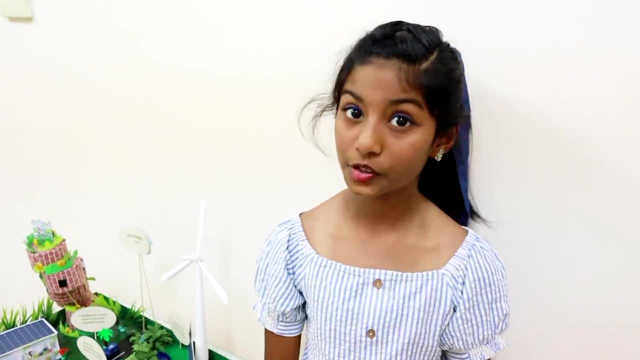 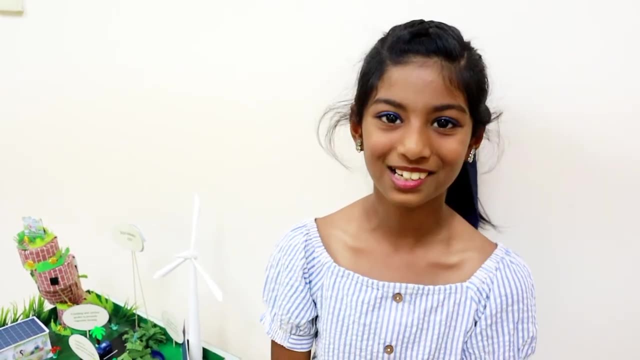 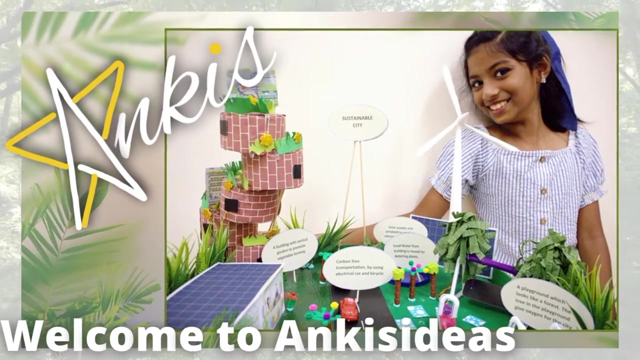 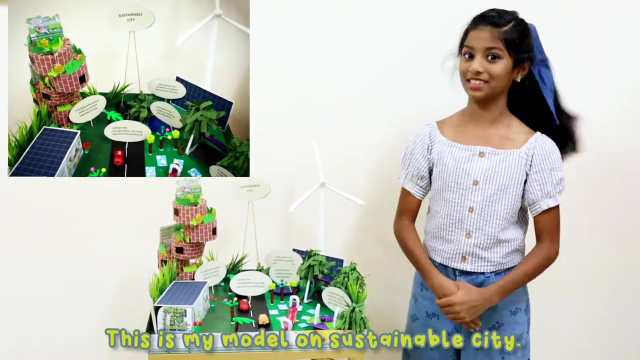 Hi everyone, welcome back to my channel. Today I am going to show you a model which I did for my project, So let us go into the presentation I did with this model. Good morning teacher and my dear friends. This is my model on sustainable city. 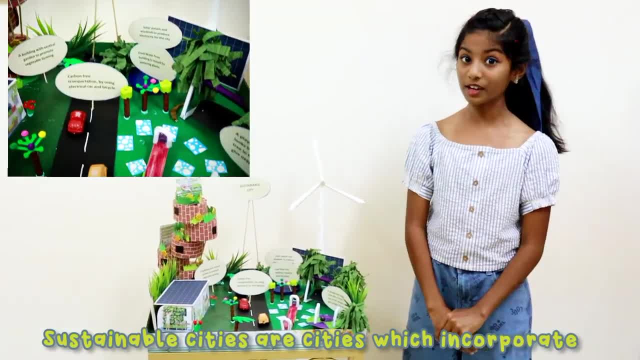 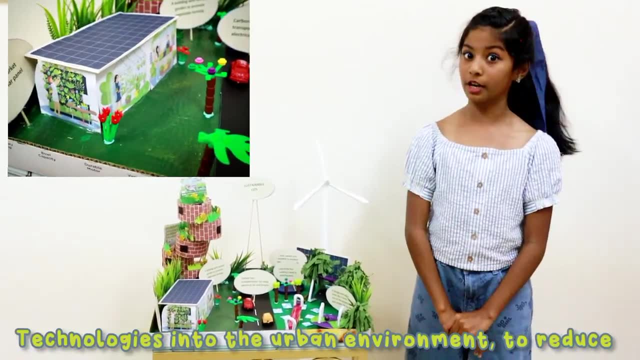 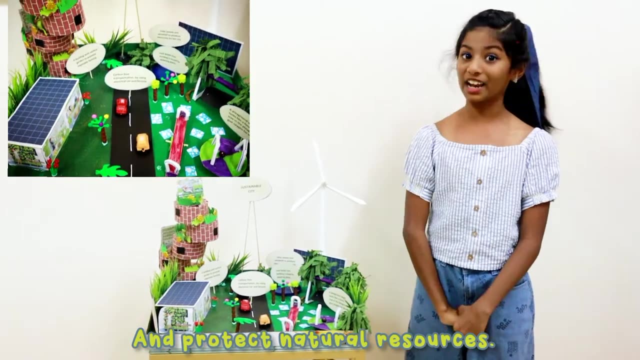 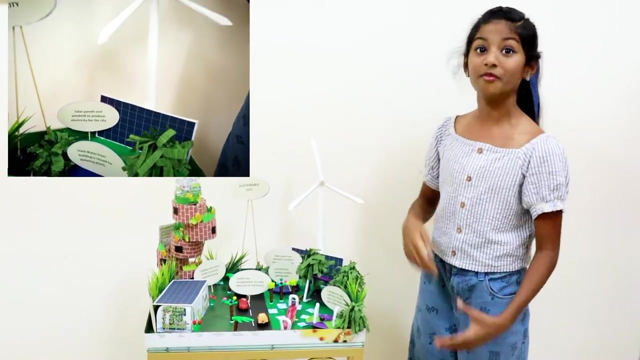 Sustainable cities are cities which incorporate eco friendly particles, green spaces and supporting technologies into the urban environment to reduce air pollution and carbon dioxide emission, to enhance air quality and protect natural resources. Here in my city you can see solar panel and windmill which produce electricity for the city by using sun energy and wind energy. 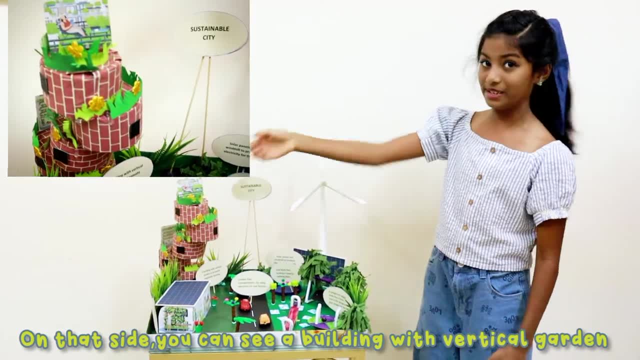 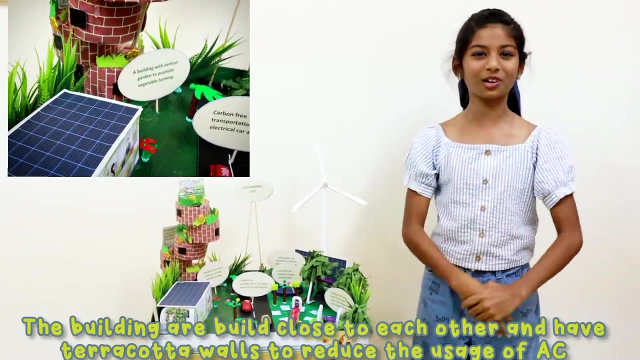 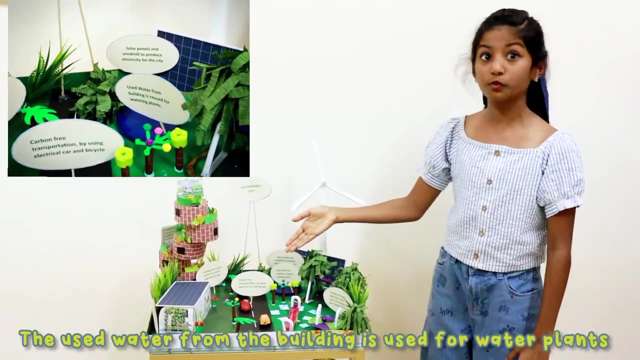 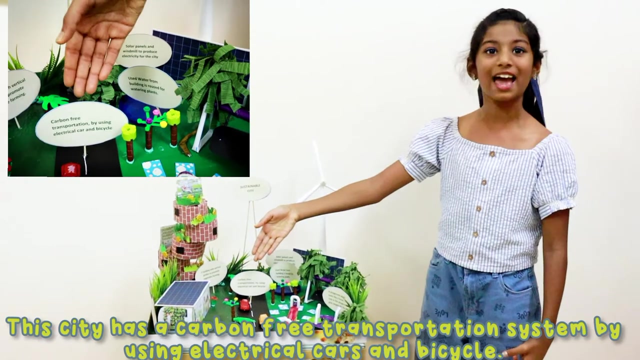 On that side you can see a building with vertical garden to promote vegetable farming. The buildings are built close to each other and have terracotta walls to reduce the usage of AC. The used water from the building is used for watering plants. This city has a carbon free transportation system by using electric cars and bicycle. 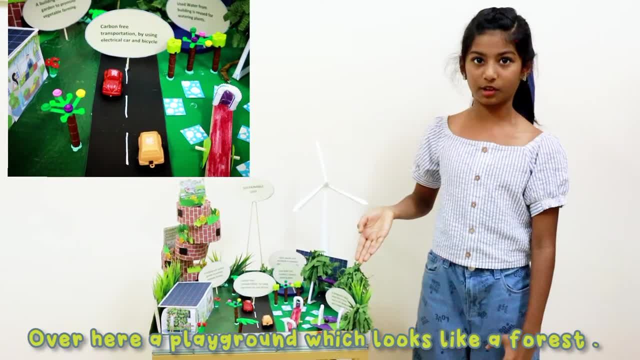 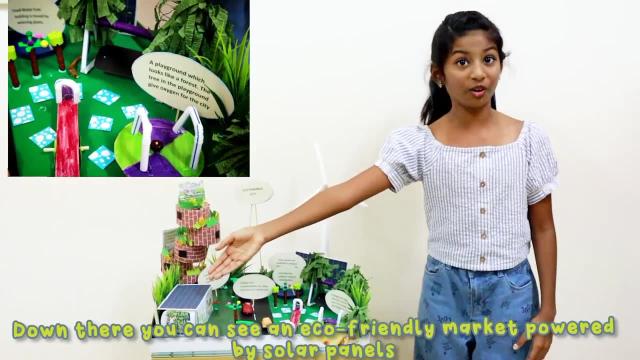 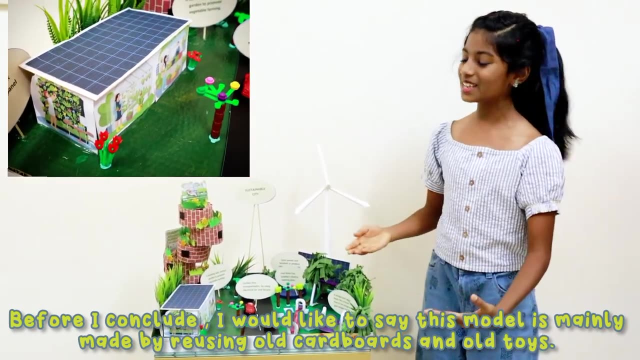 Over here a playground which looks like a forest. The trees in the playground give oxygen for the city. Down there you can see an eco friendly market powered by solar panel. Before I conclude, I would like to say this model is mainly made by using old car boats and old toys.